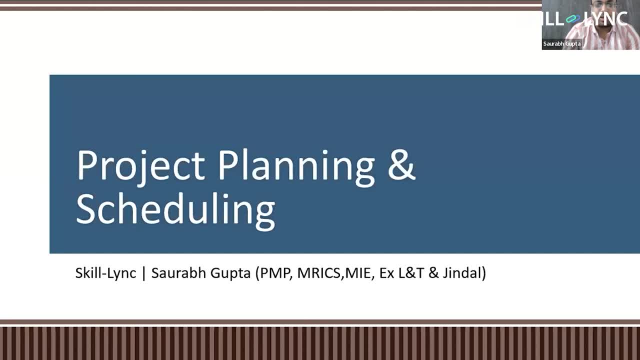 general group. So mostly I've done my entire work in the construction management field only And during this tenure I have got some certifications also. But these certifications if anybody is pursuing they can get only after five to seven years of experience only. 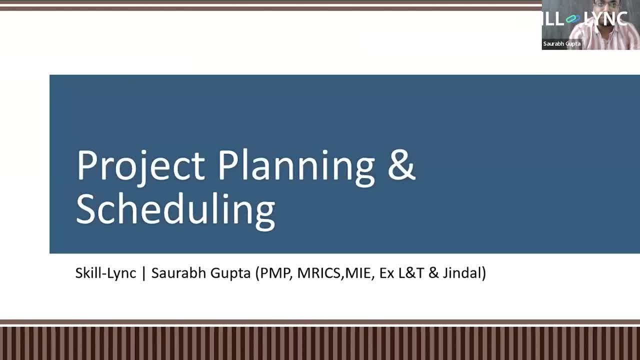 So this is the favorite topic of mine: project planning and scheduling, Because, you know, I believe that everything is related to the time, and even in our construction projects. So today we'll be going to discuss about this topic. Einstein describes time. He did a lot of. 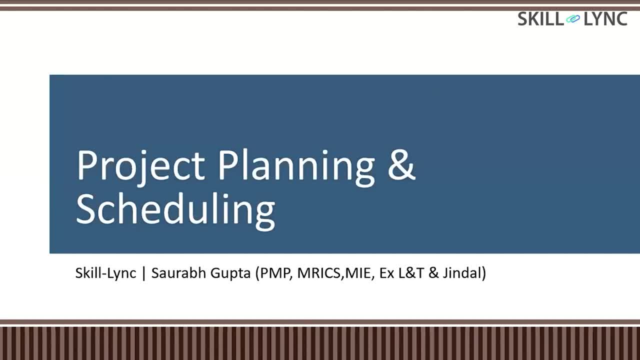 research on time. Even Elon Musk says that. you know, time is everything. So how to plan the things And even in construction projects, why we emphasize on the timing. So we'll be covering those aspects. So, first of all, let's see that we'll be starting with: you know, basic, very basic, that what is? 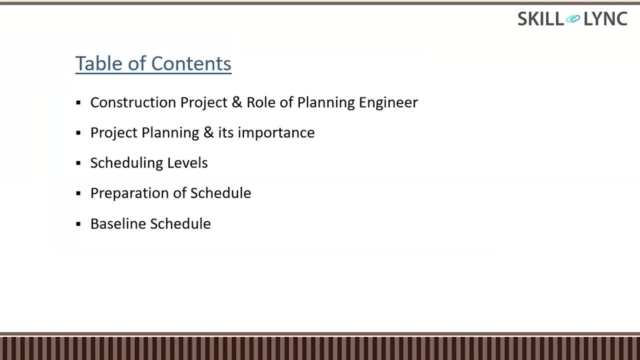 construction project and what is the role of a planning engineer. that we are going to discuss first. Second thing: we are going to discuss about the project planning. and, Okay, Somebody said that you start your video. Okay, All right, All right, Great. So second thing, we are going to discuss about the project planning and its importance. 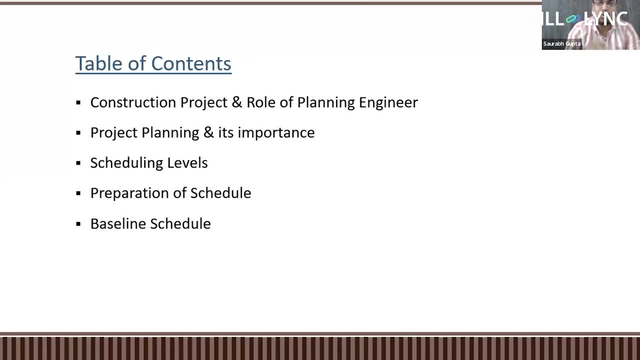 why this project planning and scheduling is so important that we are going to discuss. Then there are a lot of levels in scheduling: Scheduling level one, two, three, four, five. So what are these different levels of schedules? What is the purpose of it that we are going to discuss? Lastly, very 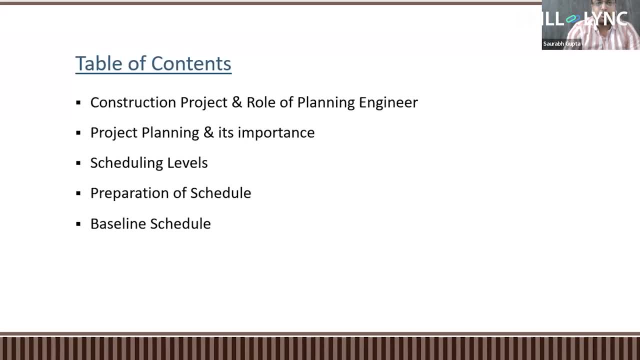 basic thing, that we have understood the terminologies, But how to prepare a schedule of a project that we are going to discuss And, lastly, what is baseline schedule and what are the other aspects related to the scheduling. And guys, whatsoever is coming on your mind maybe in between, because you know, don't hold that thought whatsoever. 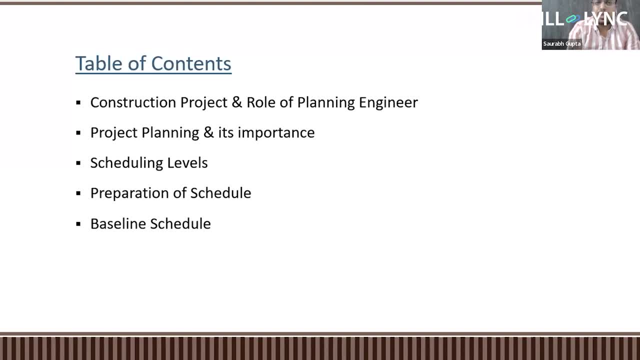 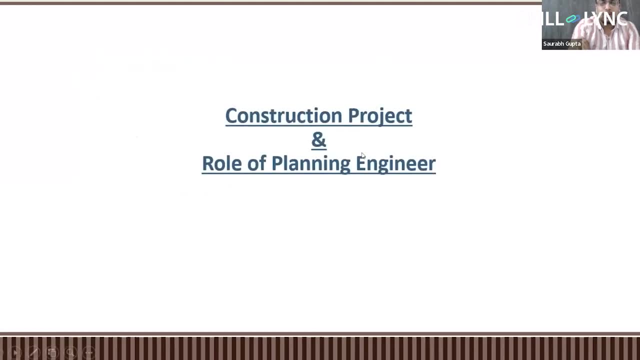 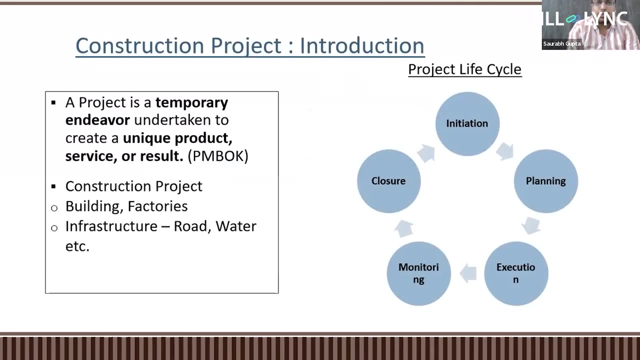 is coming in your mind, put it in the chat box so that we can have that query and we can resolve it in between the way. So first of all, let's discuss about the construction project and role of a planning engineer. So we'll start with the project. So project is basically? it is defined by one of the body. This body is PMI Project Management Institute. 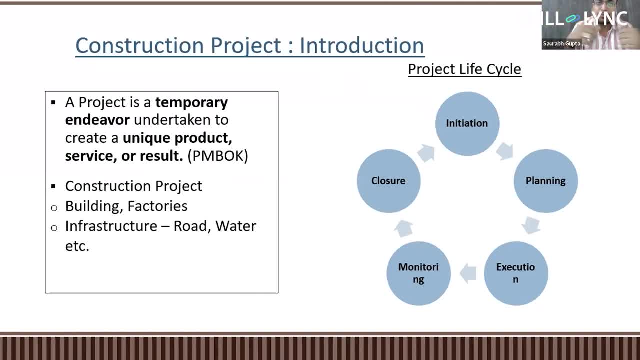 It's an American body. They have defined how they have defined the project. They have defined that this is a temporary endeavor undertaken to create a unique product, service or result. So let's say that if, let's say if you are having one project that you have to complete the BTEC, that's one sort of project. 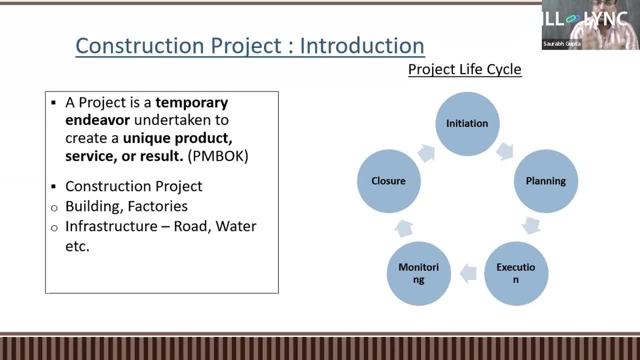 And from any of the example and with the definition, we can emphasize that. what are the major aspects of this project? that it's a limited time period. It's not like that. It's an ongoing process. In fact, it happens if some factory is there and they are making the cars or any pipe or any any kind of object. 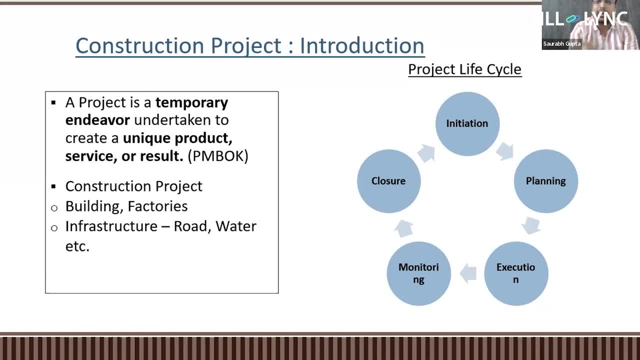 So the state of the project depends on the project. So if the project is not in the process, then it's a recurring process. Same times it will be happening again and again, but it doesn't happen in the project. Project has a definite start and a definite ending. 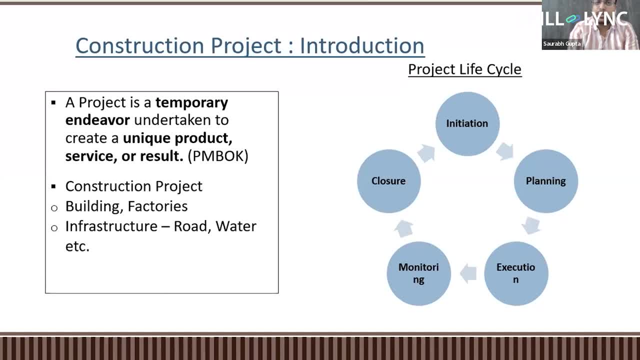 So the time period is defined, That's the logic of a project And, ultimately, by completing that project, we will be having something- either it will be a product, or it will be a service, and the result, or any you know goal which we have. 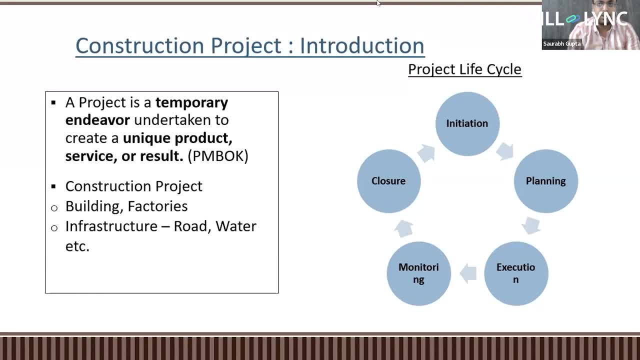 been achieved by completing that project. So Now, Oh Okay, what is construction project? you know the activities related to the construction activity. if we are building something, or you know renovating something, those are called the construction projects. so on a broad term basis, we can bifurcate the construction projects into two. 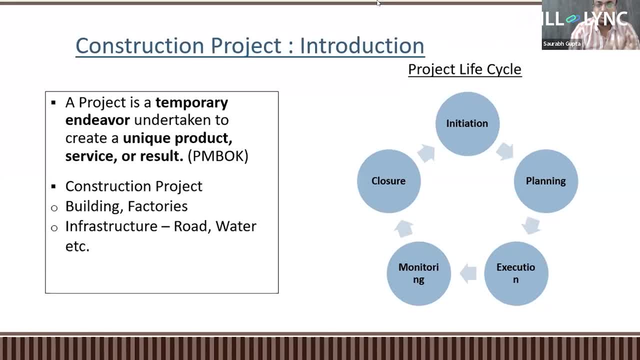 parts one is the building projects. so building, like you know, if any high-rise building is getting constructed, or if a factory like amazon is coming, qualicom is coming or flipkart, they require one factory. another factory is required by the maruti. so these all are the factories. so this is one kind 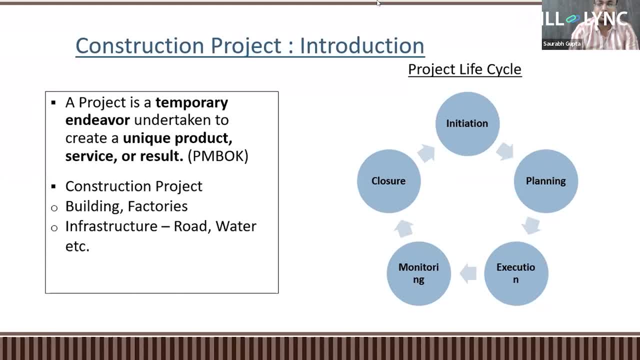 of domain, which is a very big domain: building and factories. second kind of domain is infrastructure domain. so this infrastructure domain is what? because india is a developing nation and to become a developed nation a lot of infrastructure is required. only then we can reduce the cost of our supply chain management. 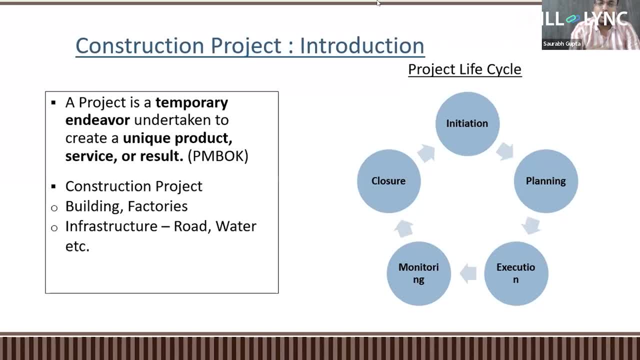 and a lot of infrastructure is required. also in india, a lot of investments will be happening, so therefore, a lot of roads will be required, highways will be required, railway will be required, metro will be required, a lot of airports will be required. similarly, we will we will be requiring a lot of water projects. 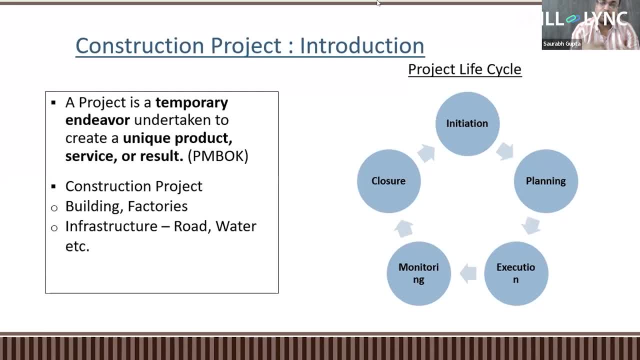 from river to the house and wastewater disposal from house to the sewerage treatment plant. so likewise this infrastructure projects, which is carrying a lot of under domains. so that is why India anybody can emphasize: currently we are having almost 8,000 plus infrastructure projects which are in pipeline from the government initiative. so this is the kind of thing. 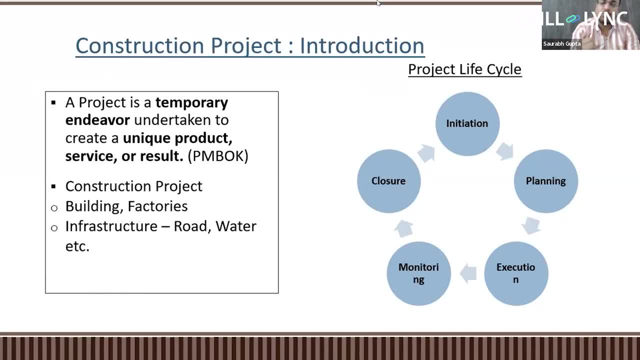 which India is having a lot of lot. infrastructure and building projects are coming so that India can become a second number of. you know the country all over the world. right now it's on the fifth position with respect to the economy. so to become the second number of economy, they require a lot. 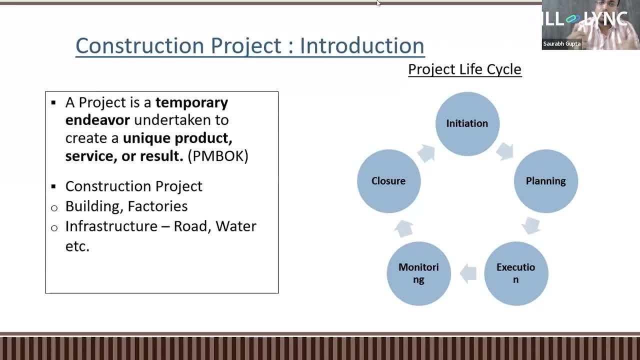 of infrastructure projects. to become a developed nation, they require a lot of infrastructure projects. now let's come into the topic: project life cycle. so what's a project life cycle? so we know that a project is there with a limited time period, with a definite goal. so we can define the entire project into five phases, starting with the initiation. 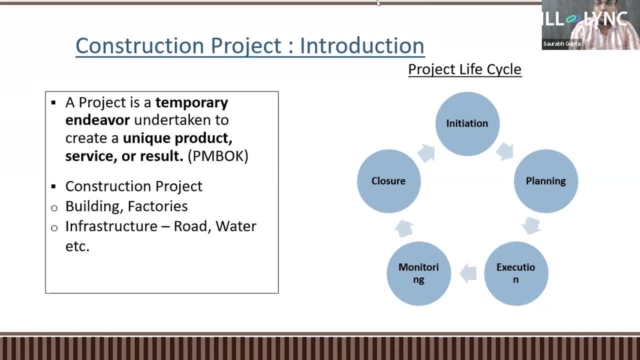 so we'll be taking one example. let's say we have to make one flyover project. government wants that project because so much congestion is there at some place. so they'll be floating the tenders to so many parties, construction companies like Tata Island, Tisha Port, GGR Infra. 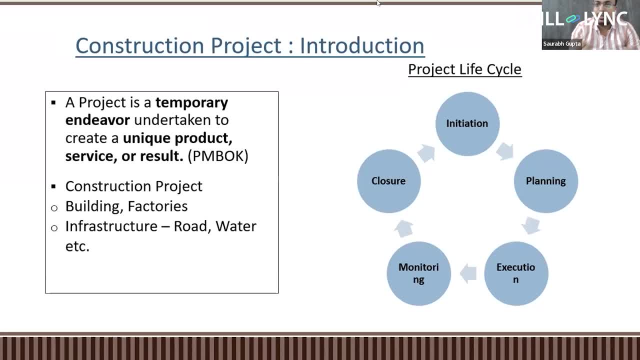 so these parties will be bidding, they'll be participating in the bidding and the whosoever will be at the L1 position. the contract will be given to that contract company. so now they are two parties. one is client, second is contractor company. now this contractor company has got. 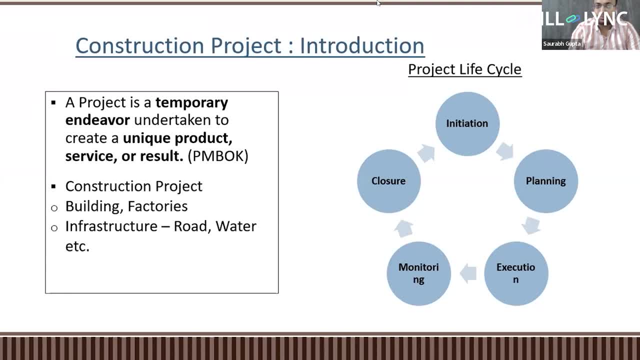 that tender. let's say in two years they have to construct this flyover. so they will be completing this flyover in two years. but to do that they will be first doing the planning: how they will be completing this flyover in two years, what activity they will be doing. 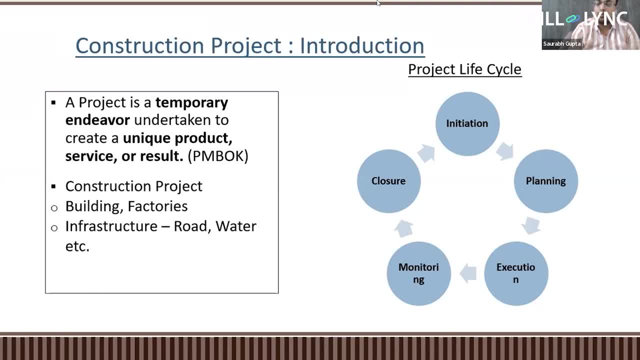 in this month: weekly basis, daily basis- that is the role of planning and then the execution will be happening after the plan. then people will be going to the site, site engineers, they'll be doing the construction activity. they'll be doing everything based on the plan, but during 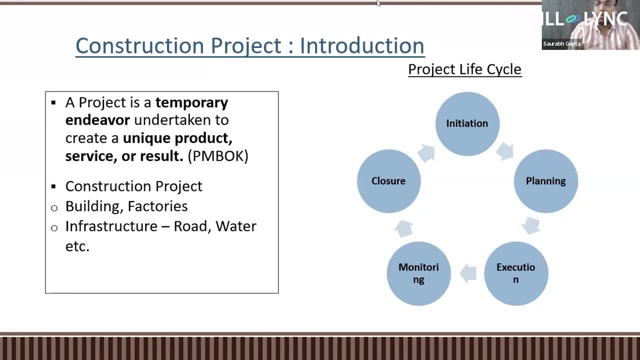 this period, the planning engineer will be monitoring how this execution is going, whether it is going as per the plan or not. so they will be getting the progress reports on periodic basis from the site team and then they will be evaluating whether this plan, whether this project, is moving as per the plan or not. lastly, once everything is achieved, whatsoever has been, 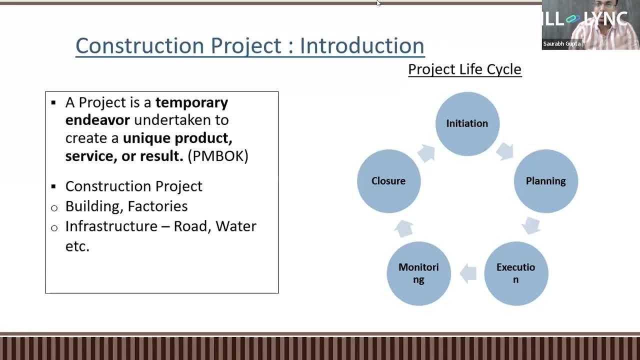 mentioned in the contract document that has been accepted, and then they will be doing the planning and then the project will be closed. so these are the five stages. now, in this today's class, today's webinar, we are going to discuss about this planning. so now let's. 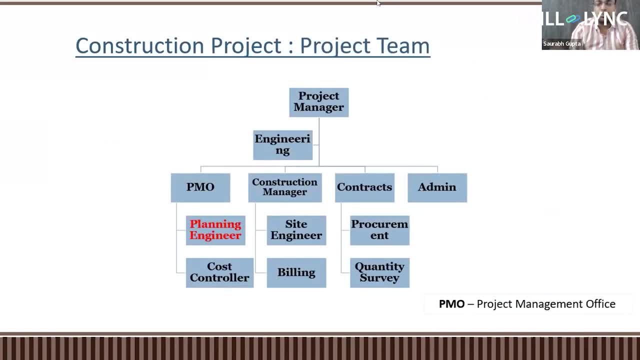 understand. we have understood that this project is there, the project life cycle is there, but something: some people will be required. civil engineers will be required, or even the mechanical and electrical engineers working in the construction industry will be required to complete this project. so how does this project team look like generally? on broad basis, we can quantify this entire project. 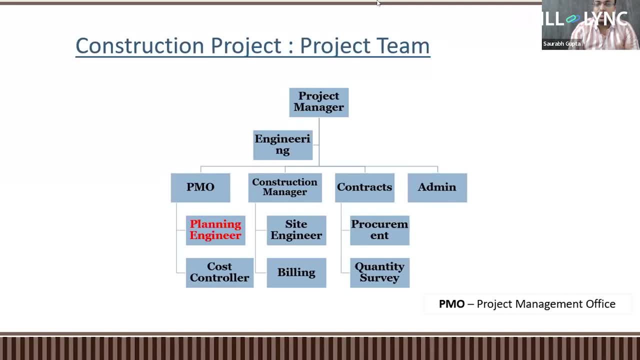 team into three parts. so one part is the project management office, so that is called the PMO. this PMO basically takes care of the two major aspects, that is, time and cost, because every project we started with the flyover project as an example, so a flyover can be of 200, 300, 500. 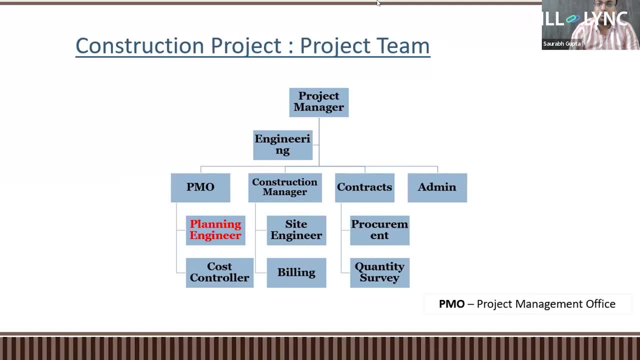 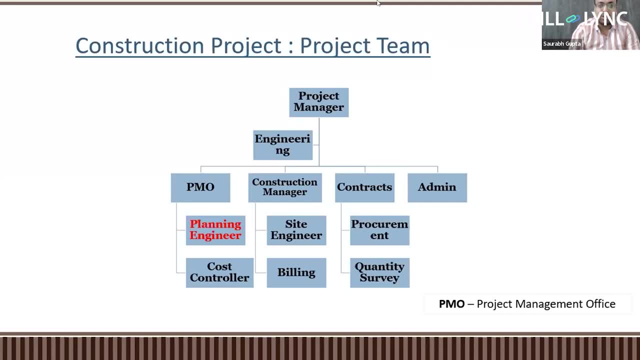 year time slot is there in which we have to complete this flyover, but what will happen? it will not be completing. so, as per the contract document, which will be mentioned in mostly contracts, there will be a penalty. let's say that two in two years we have completed the. 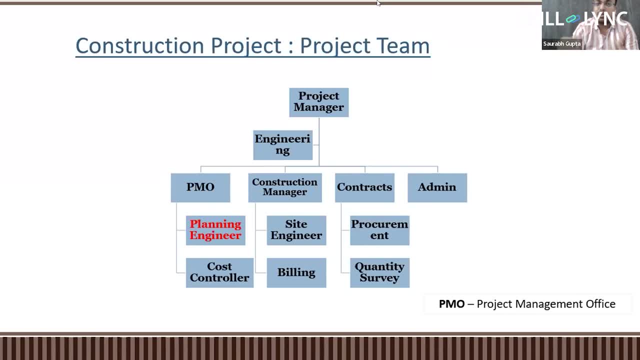 only 70% work, then for the 30% work there will be huge penalty. so then the profit will be gone and the company will not be gaining anything from that project. so that is why time is very important aspect. other aspects are like contracts in the project team. so under the contracts 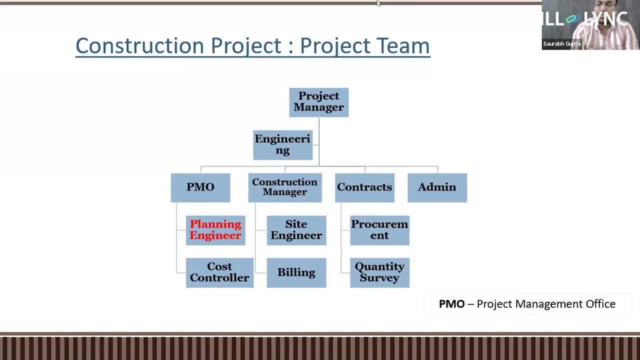 procurement department will be there. who will be procuring all the material and services. quantity survey is there. these people will be doing the tendering and billing process. then construction department is also there and under the admin few people will be there like hr and other. yeah, great. so penalty means you know the client will be saying if you will not be completing. 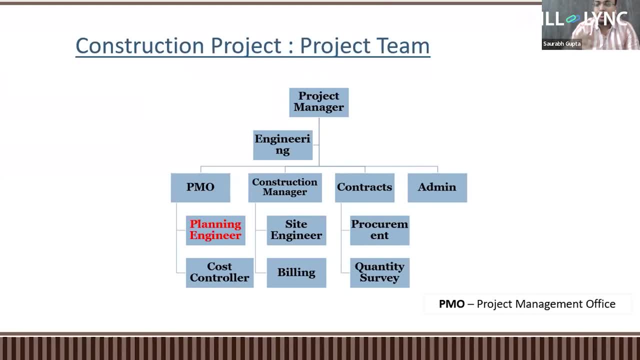 the project in two years, which is defined in the contract document, then they'll be leveraging for this 500 crore rupee project. we have completed 350 crore rupee, 150 crore rupee. work is pending for that 150 crore rupee. if you will not be completing daily, they'll be deducting some, let's say, 10 lakh rupee or. 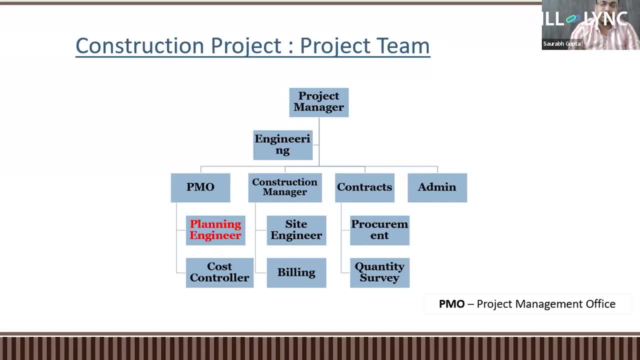 depending upon one percent of the remaining work, as per the contract condition. so that will be the penalty of it. so now let's understand. okay, PMO, not clear. okay, PMO basically is project management office. okay, so under the project team there are three major departments. one department is the 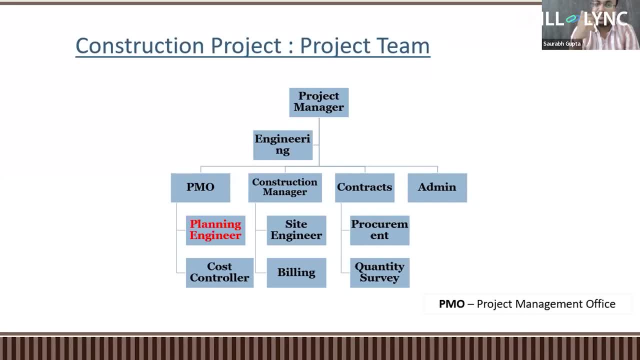 project management office. so in this the civil engineers are working as a planning engineer or cost controller, so they will be managing the entire project time aspect and cost aspect. second department is contracts department. so this contracts department does all the procurement and then they do the quantity survey, tendering how to get the more and more contract from the whatsoever has been done and 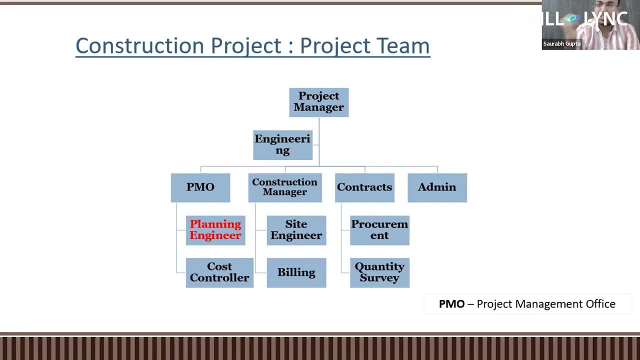 published by the client. third department is the construction manager. so these people will be working at the site level, but the PMO people and contracts people, they will be working in the office only. all right. so now let's move to the next section, which is project planning and its importance. 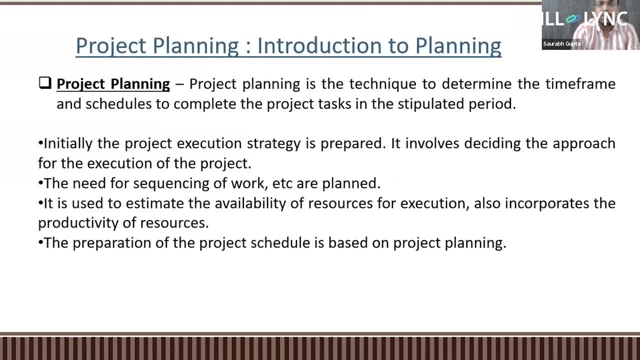 and scheduling levels. so what is basically this project planning? so project planning is the technique to determine the time frame and schedules to complete the project tasks in this duplicated period. so let's say that this is okay, one kind of definition. but basically, if you are going from your home to college or your location, 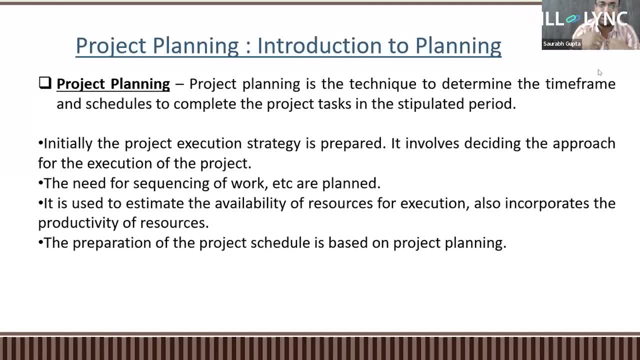 then you will be planning how you will be going and reaching to that particular destination. here the project planner is basically a civil engineer, so he knows that by reading the contract document that we have to complete this project into two years. and these are the tasks, let's say, for this flyover. they have to do the excavation, they have to do the. 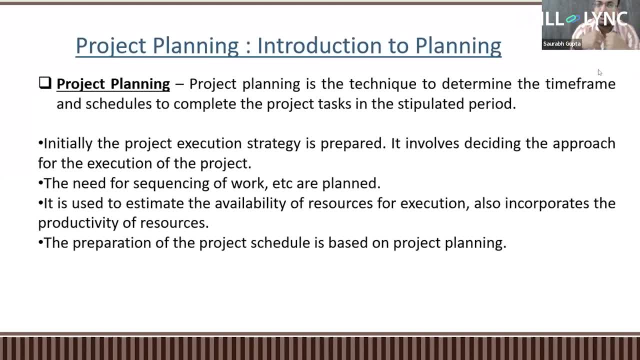 foundation work, they have to do pre-casting work, then they have to do the launching of girders and then finally they have to make the road on that flyover. so all these tasks have been scope has been given in the contract document, so then he will be doing the planning, so he'll be making one. 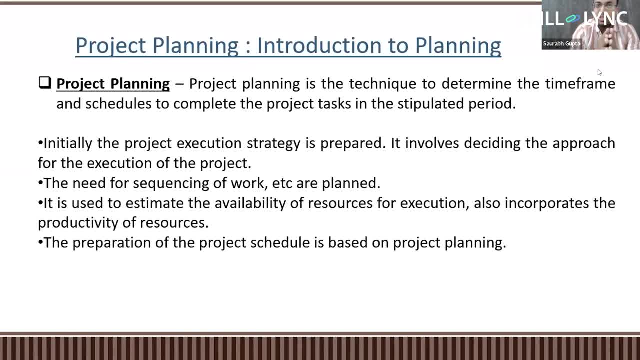 execution strategy. how do they want to do everything? they want to do as per the casting 2 means at the site level only. or they want to some pre-fabricate some material, then transport that material and then place those materials at the flyover. so they'll be making one. 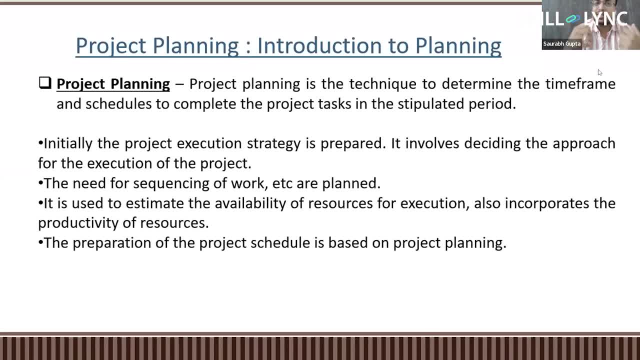 execution strategy. so first they will be planning this execution strategy. based on that execution strategy, they will be making the schedules like we will be completing, let's say, in first three months they'll be completing the construction. for example, first 3 months they will be completing theài. 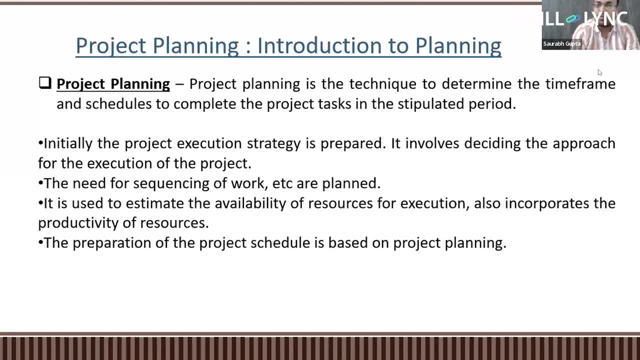 procurement part. first they will be buying the concrete, steel and everything. then in meanwhile the design will also be completed in first two, three months by the design department. that's a separate department. then in the first six months they'll be completing the foundation activity. so likewise they will be preparing the project plan and they will be making a entire. 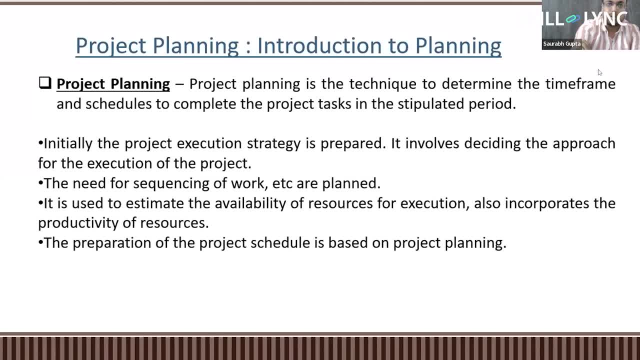 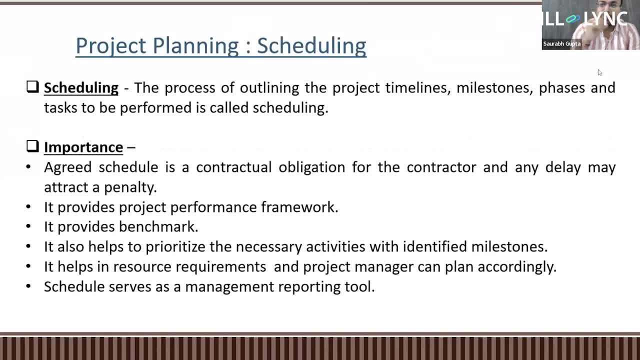 schedule. all right. so now planning is. planning is with respect to the everything. okay, they'll be making the plan with respect to the material: in how much time this material will be coming. then they will be making the plan that you know these risks will be there. so entire execution. 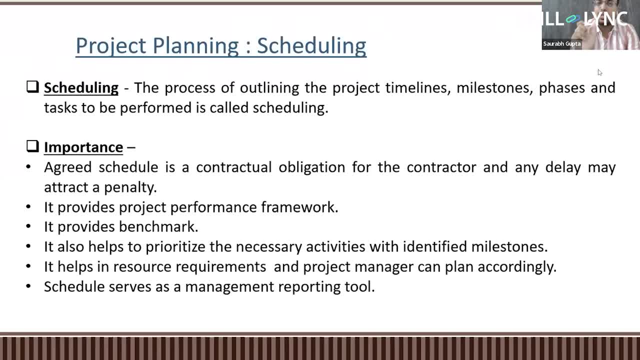 strategy will be there, but scheduling is very simple. it's related to the time frame only. yeah, you guys, if you have any questions in between, just put in the chat box so that it is. i'll be having that kind of visibility. so scheduling is very simple. so that's the. 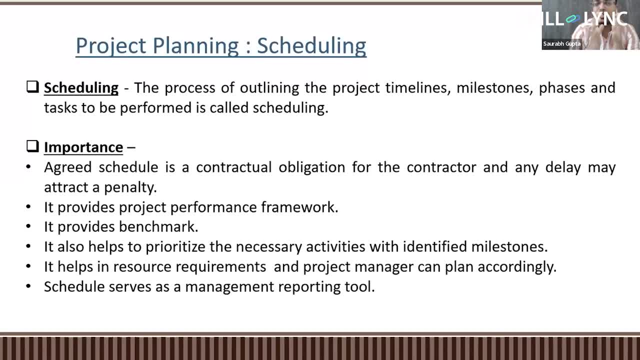 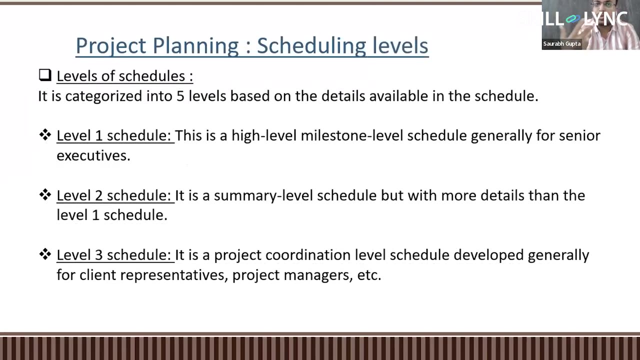 difference in planning and scheduling. planning is basically it covers a lot of broad aspect, but scheduling covers time only. so in time, basically, we will be analyzing that, yeah, in this much time period we are going to do these many activities. all right, now there are five levels of schedule, so it's generally a question when everybody asks either. 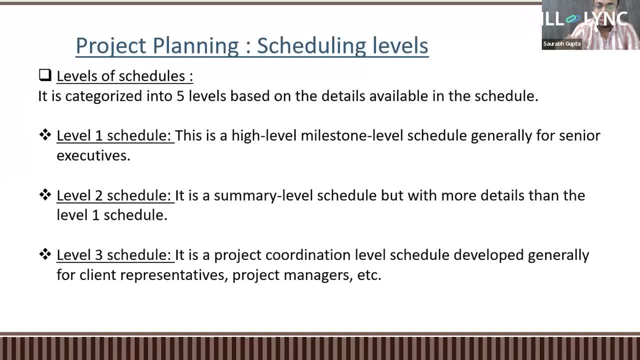 you know, uh, if you are going for a uh outside india in your university or you are going for an interview, question that how many level of schedules are available? so generally, as per the planning, there are five level of schedules. should we do any separate course work? so there is no separate work, so everybody will be working in a different portfolio in pmo. 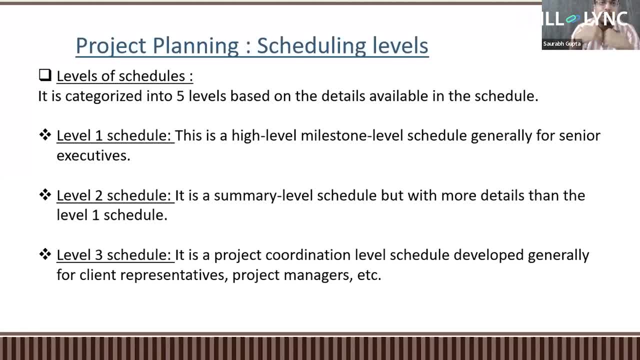 so these people will be planning engineer and cost engineer. so under this project planning, we are having the five schedules, all right. so in these five schedules, what is the difference and why these schedules have been created? so let's take one example. okay, let's say that you are constructing this flyover. so, like i mentioned, 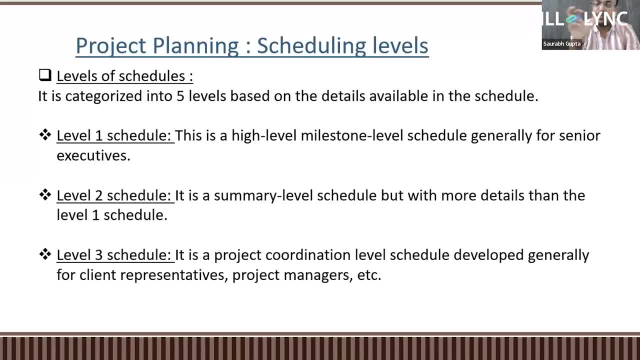 that we have to make a schedule for each of these five schedules. so let's take one example. okay, let's say that you are constructing this flyover, so, like i mentioned, that we have to make the schedule. so then we will be making one very high level milestone schedule, like i mentioned. 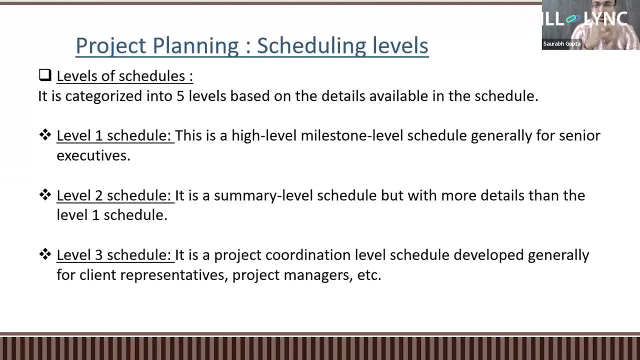 that if first three months will be for design and procurement, next six months for foundation, next six months for prefabricate work, next six months for completion of the execution activity. so this is a broad level milestone. so this generally helps the- you know- client and the executive committee of the company. okay, in this one, in this way we are going to. 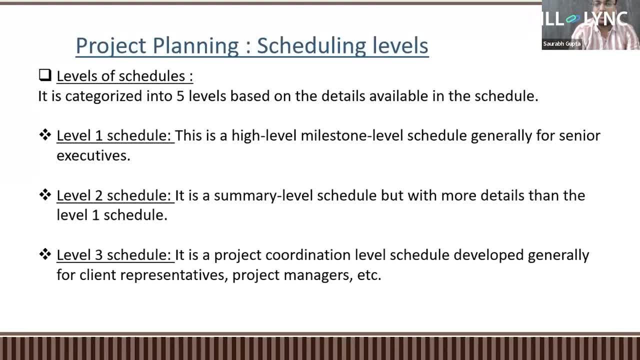 be able to for learn about how much you can do be done within how much time we have in savings. okay, so we are going to talk about how much detail we need to do inside that agenda that was mentioned, the first external from the client and the iit. so this is the further summary level that has been prepared, so maybe 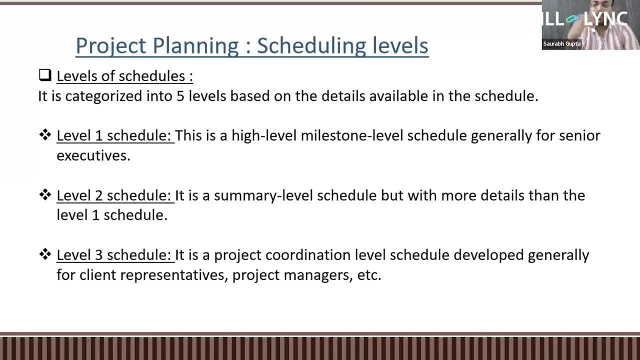 company is a very big. you know big companies are having low, so many levels. so now first high level: milestone level was prepared for the md and ceo of the company. but level two schedule is available for the that particular business head, maybe particular that let's say for that infra head. 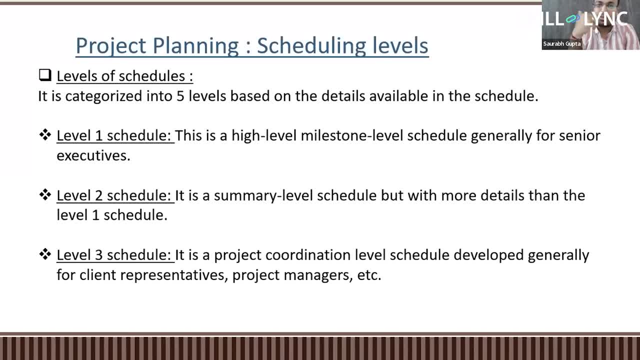 he is looking for this summary level schedule. then further, further, we have given so much thing. so in this level three schedule we have you know, further provided so many details. so that will be for the particularly client and project manager, so that project manager, on day-to-day basis he will be having such kind of details. so in level three schedule 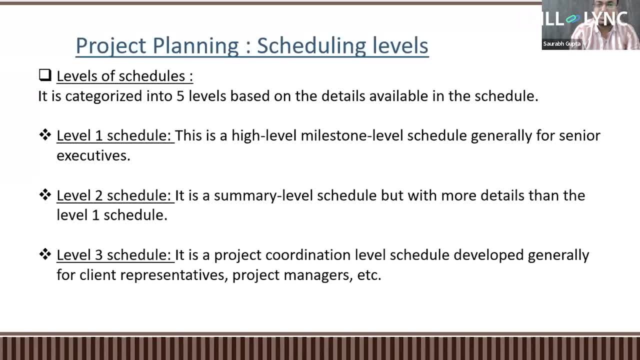 let's say, after the first three months, then we planned another six months for the foundation work. so then in the foundation work we will be mentioning that in this foundation work we will be doing excavation or drilling, then after the drilling we will be pouring the this, we will be putting the steel cage, then we will be doing the concreting. 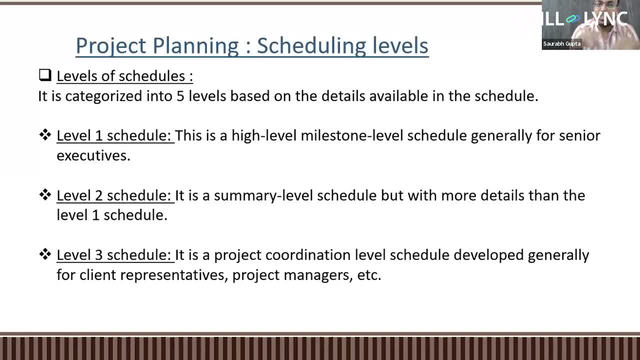 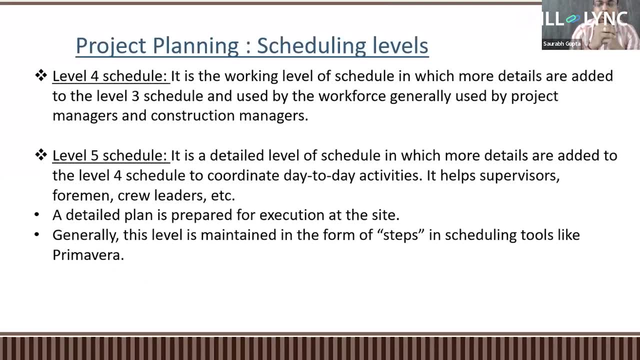 then we will be doing the curing. so that will be mentioned in the level three schedule. now level four schedule is, you know, for the construction managers under the project manager construction managers. so they require more detail. now if we are saying that, okay, concreting is there, then which peer? 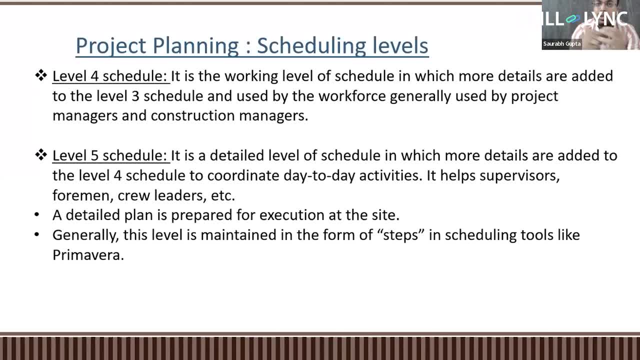 concreting is there to happen and under that concreting you know what are the different activities that are going to happen. that will be detailed in the level five, like they will be mentioning level five, further drill down. it will help the site engineer, foreman and subcontractor. 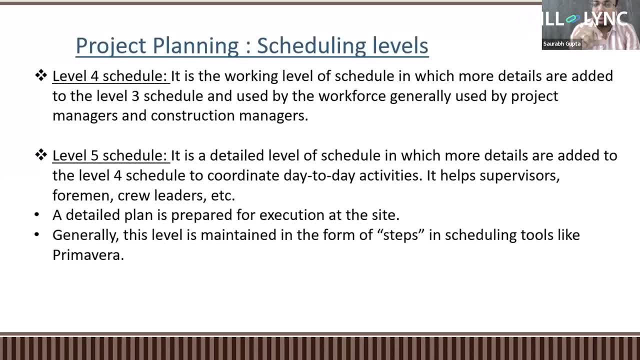 that you know shuttering the site engineer and subcontractor, that you know shuttering the site engineer will be happening on this day and even at shuttering, you know, then they will be doing the re-barring. so after the re-barring and shuttering, before that, staging will be happening, if staging 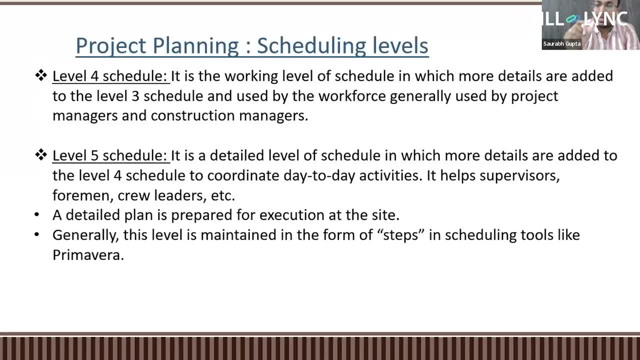 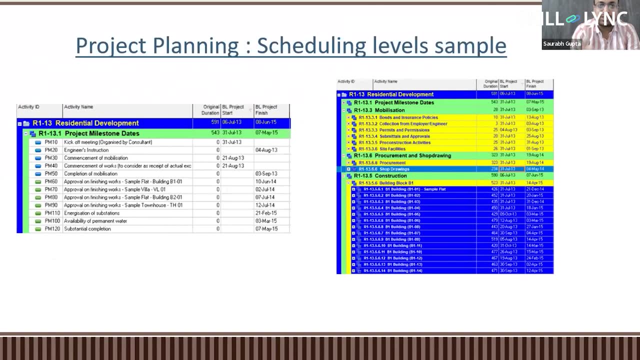 is required. so such kind of activities further drill down at the lowest level, up to what we can go and drill it down. that will be explained here. so let's take one example how it will be happening. now we have gone through the flyover. let's take one example of the 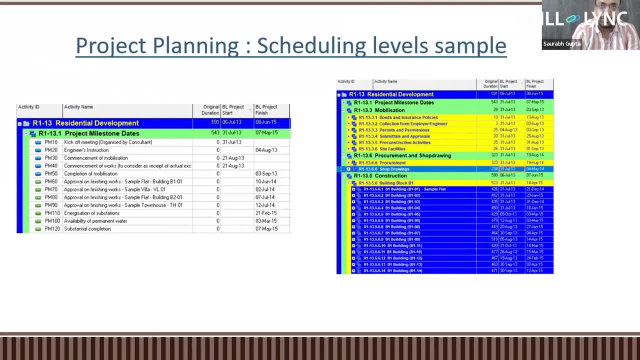 residential development. so in this residential development, firstly, this is the level one. so here we have just mentioned like project milestone dates, so kickoff, meeting, engineers, instruction, then we have commencement and starting of the project, then we have like completion of mobilization, approval, then, uh, approval of permanent water, substantial completion. so basically milestones whatsoever we will be. 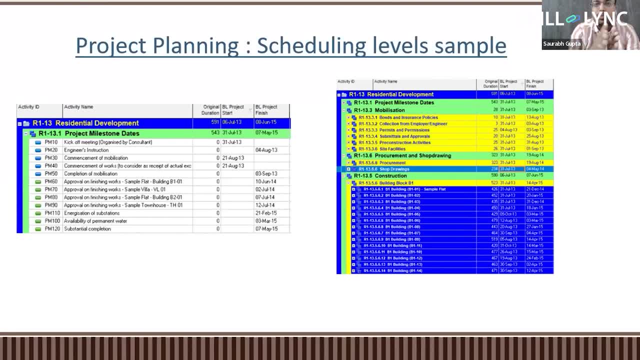 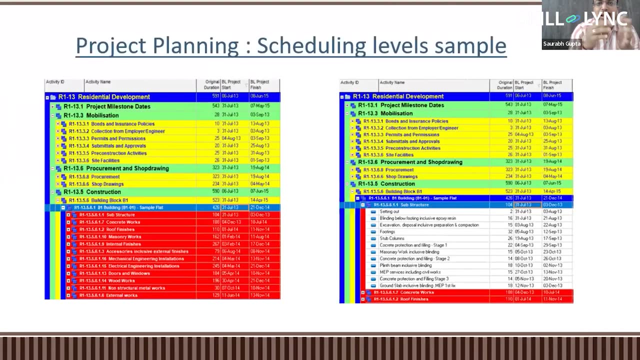 doing that has been mentioned here. then further we will be drilling it down that under mobilization, what will be happening. so this is level two schedule. so similarly, we'll be having level three and level four and level five. so on the left hand side you can see that for this. 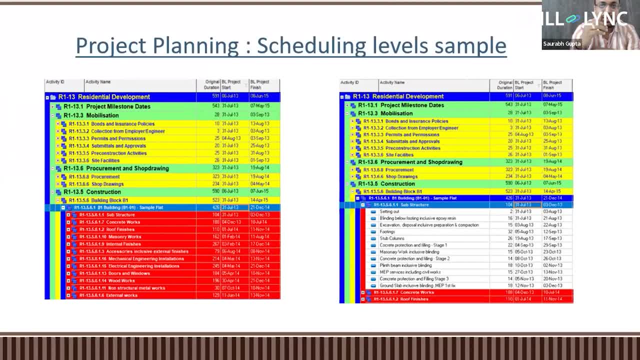 sample: flat on the bottom side we are having substructure. then under the concrete work roof finishes. that is level four schedule. now on the right hand side you can see under the substructure we are setting out then we do have footings, stubbed columns, concrete protection. 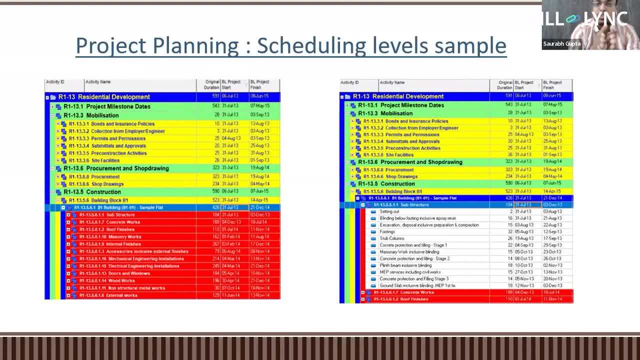 all this further drill down of the activities so that we can, you know, track it on the level four day-to-day basis, even with the available resources. so ultimate purpose is very simple: level one, two, five, level one: we provide the milestone type of summary, then we further drill it down at the level. 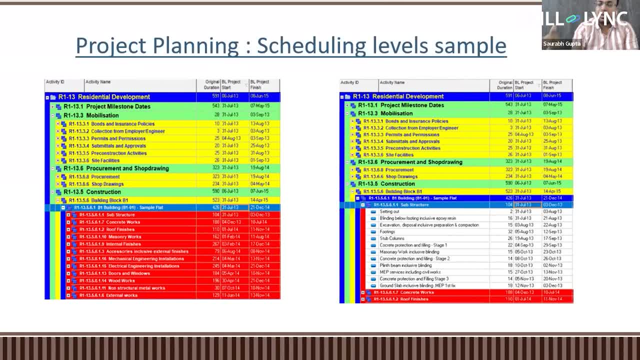 five, we provide ultimate thing that at the last, if we want to track that, yeah, what our labor or foreman or subcontractor he will be doing on that particular activity, then we will get to know that for from milestone, that, foundation in foundation, this peer number, foundation in this peer foundation, concrete work under that concrete work. 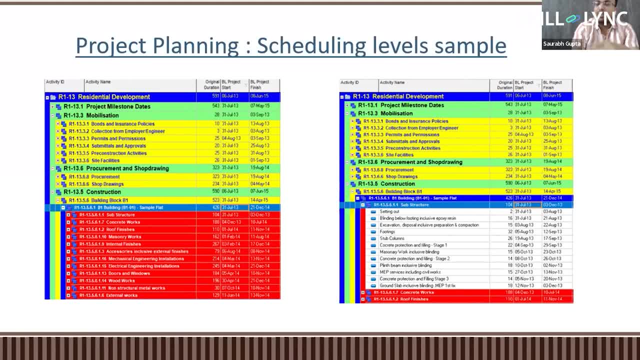 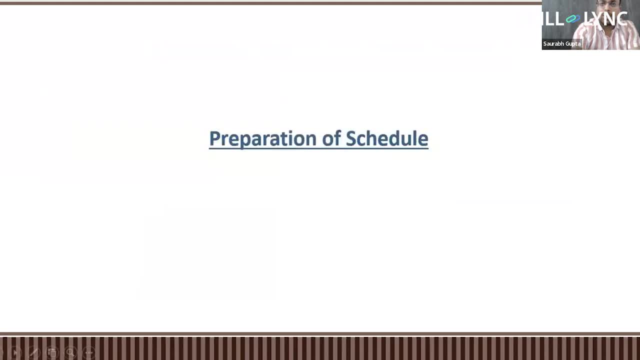 then in level five, this shuttering will be happening on this day, so this will be the level five schedule. so i hope, now we have covered that, you know what is planning, what is scheduling, how many types of schedules are available and why it is required, because you know once we know that 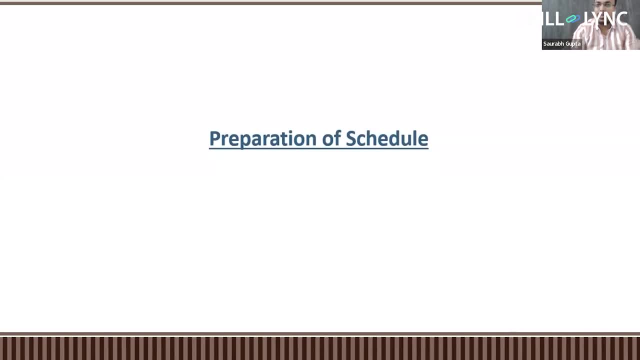 by this schedule we are going to complete the project. we will be tracking it. So therefore, the schedule is required. Now, how to prepare a schedule? Because once you will be going, it's not like that a fresher will be directly making a schedule. 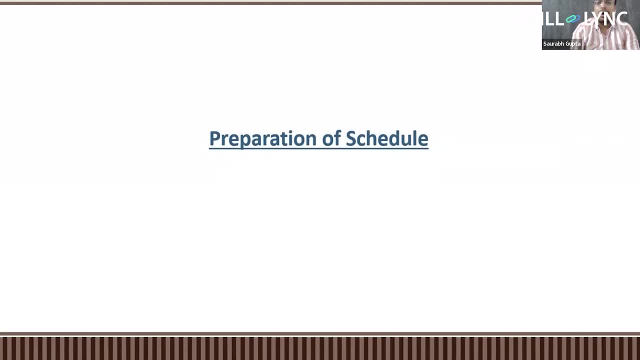 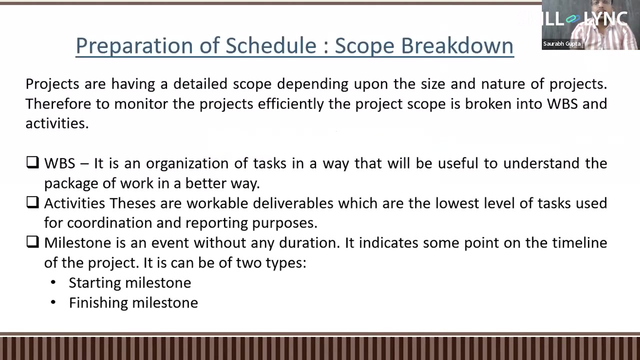 So managers will be there. He'll be directing them how to make the plan, how to make the schedules, So, but you should have a basic idea how to make a schedule, Because for a planning engineer, this is the main thing. OK, so a project will be having a lot of items. 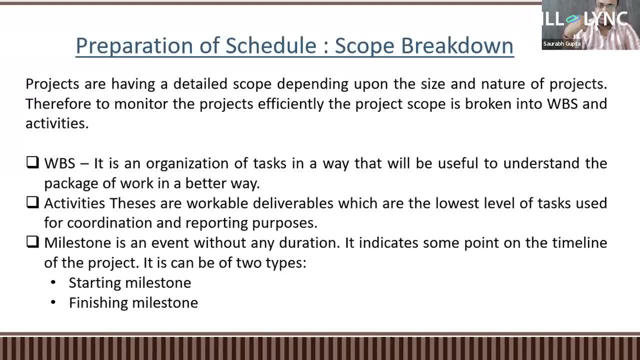 OK, so, like I mentioned, if we are covering a flyover project, so a lot of items will be there. So, first of all, we will be breaking it down and we will not be breaking the entire scope. We will be breaking down the scope in a logical way. 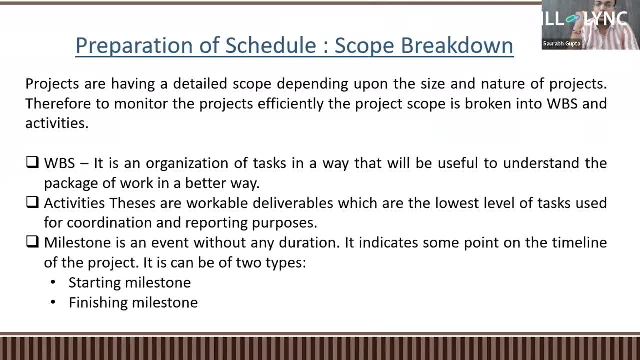 So for a flyover project we can say that, OK, firstly we will be doing the foundation work, Then we will be doing the prefabricated work at the casting yard where all the girders that we will be doing. Thirdly, we will be doing the pier casting work. 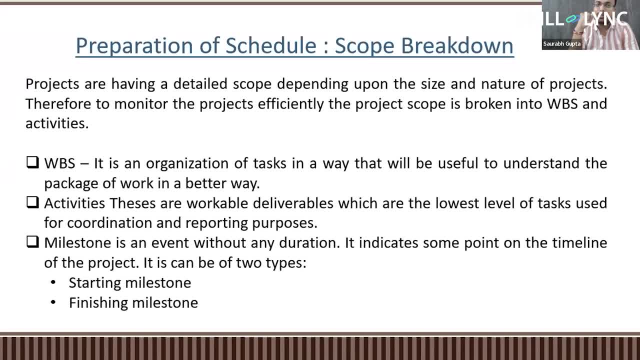 Pier means columns, So that we will be doing at the site, Then further we will be doing the launching of these girders. We will be transporting Those girders which has been prefabricated and bringing it at the site level. 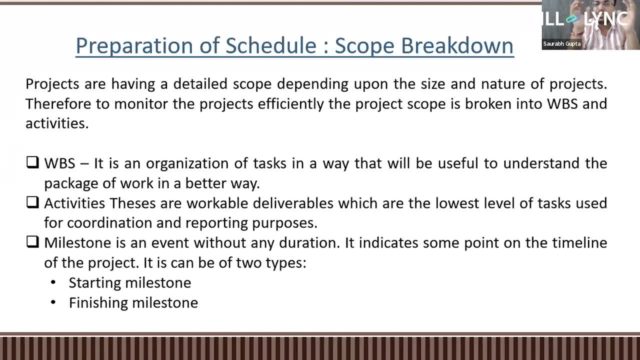 So likewise, we have made some segments that under each segment we will be having the different activities. OK, so this is first way. first step is to do the WBS, is to make the WBS work. breakdown structure: After the WBS then we will be. 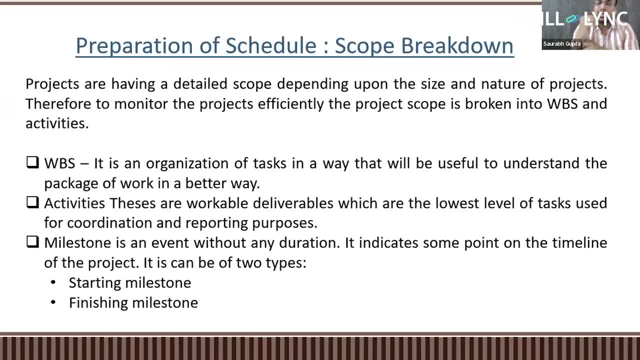 Making the activities in that particular WBS. What will be different activities available? Let's say, if we are making this pier, So first we have to do the. let's say this pier height is of 10 meter. All right, Generally it is not of 10 meter, but let's say it's 10 meter. 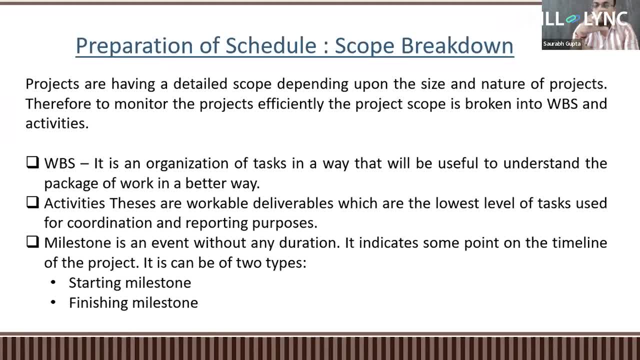 OK, so now you know that up to which level we can do the shuttering. What should be this shuttering height? OK, so generally It is taken as 1.8 meter or 2.4 meter. OK, to improve the productivity and to complete the project in a fast manner, let's say 2.4 meter. 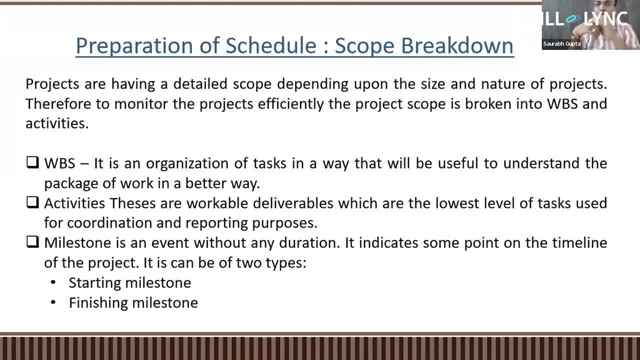 So we have to do the level of four levels: 2.4 into four times, For example. so now we know that to make the activity first we have to do at the ground, then we have to do the first level, second level, third level. 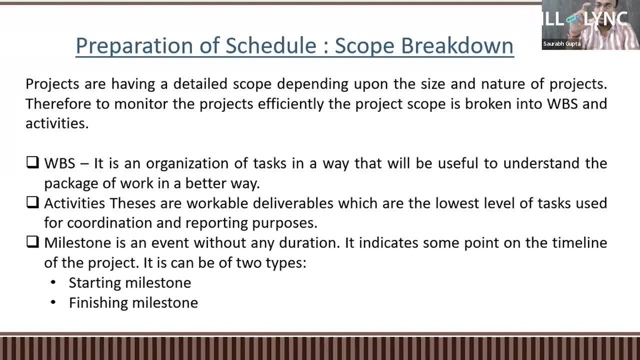 So we have to do the staging work, We have to do the, We have to do the rebar work, we have to do the shuttering work, then we have to do the concrete work, then we have to do the, the scouring activity. 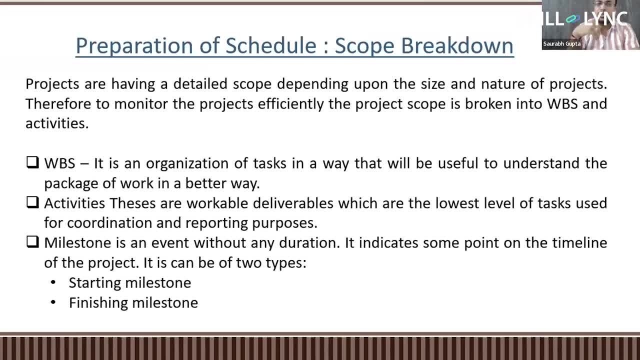 So all these activity for that one particular pier will be mentioned, All right. So similarly, let's say, these will be the activities and that comes under the 1WBS work breakdown structure. So that is the pier one, All right So. 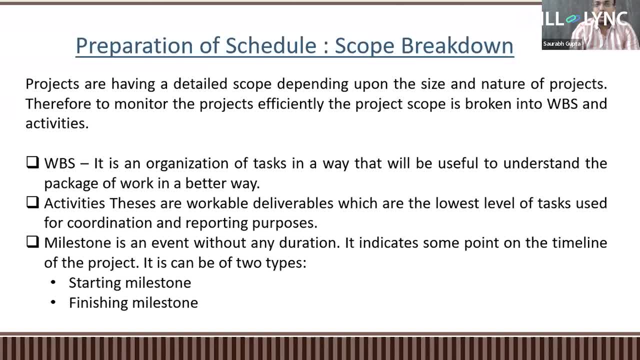 We can also make the milestone. milestone is like that which is not having any duration, and any activity will be having duration. Let's say that you are doing the concrete. So this concrete activity, it may take a few hours or may take a day, or may take any time. 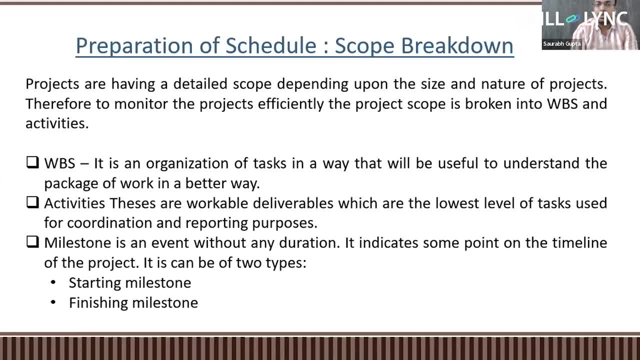 But this milestone activities of zero duration. So if anybody asks what is the full form of the milestone or how you will be defining the milestone, So once a one form to say that milestone will not be having any Duration. So generally we provide that this is the starting milestone and finishing milestone. 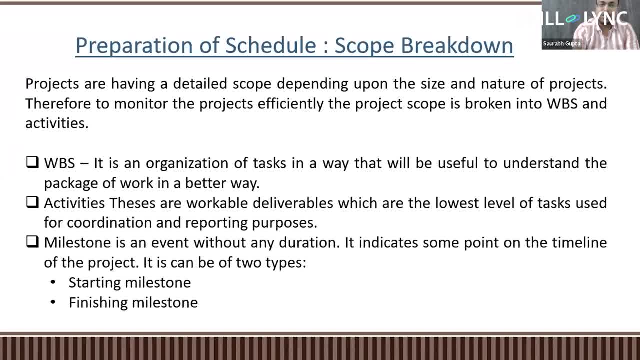 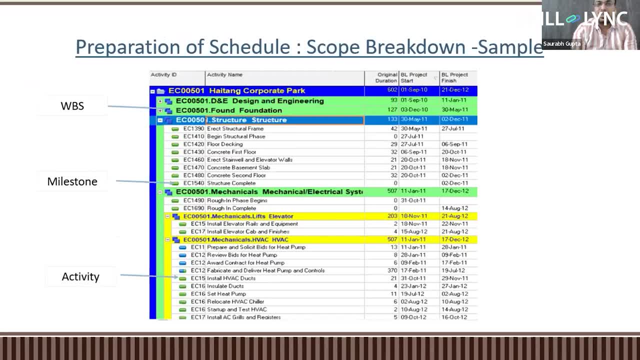 So start of the project is the starting milestone and finishing completion of the project is the finishing milestone. So what we discussed like WBS milestone and activity. So once you will be doing all this, so you'll be making everything like this, first you'll be making WBS. 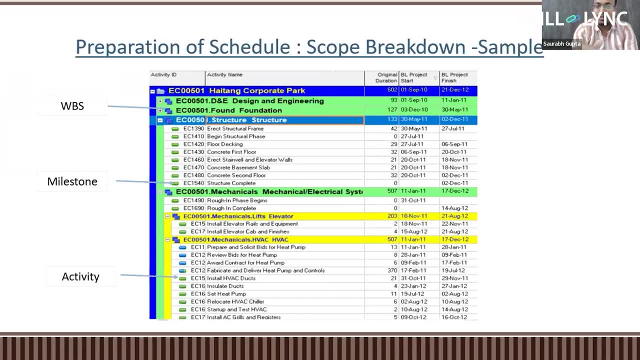 Then You Will Be making milestones which are having zero duration, and then you will be making further activities, All right, So in this entire thing you may see that in the activity name you can see the activity. then there is original duration. 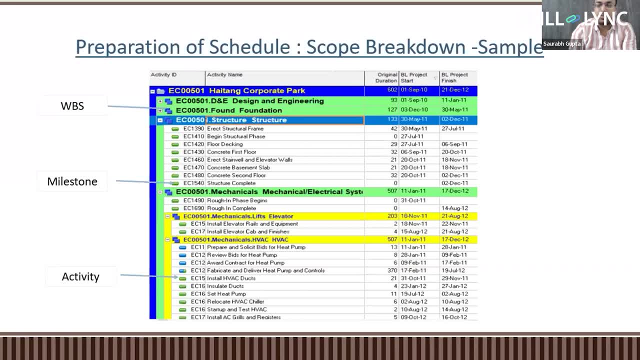 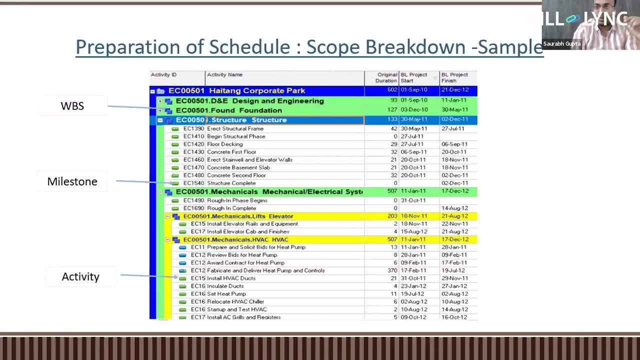 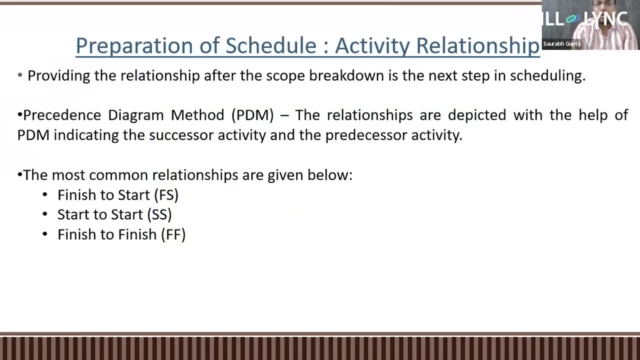 That scope is bifurcated into WBS in a logical manner. Under each WBS we are having further activities. All right, So now we have got the activities. We have made the list of activities. Now what to do with that activity? 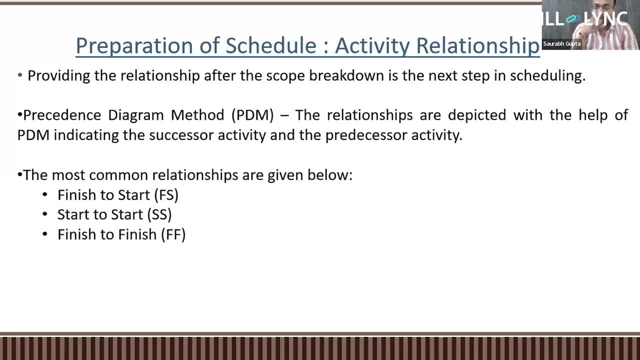 So now we have to align all these activities. Why we have to align? Because then we will be giving a relationship, Then we will get to know that which activity will come after which activity. So that is why there are one methodology, which is precedence diagram method. 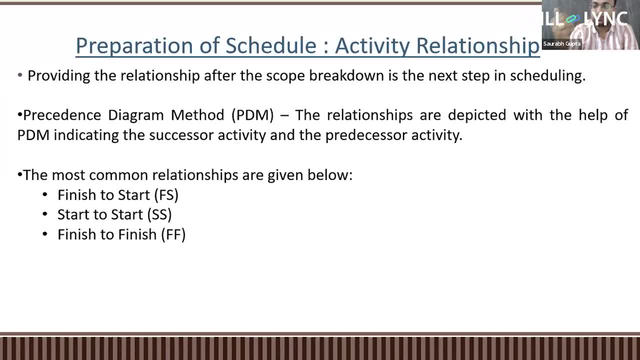 Okay, Who will proceed and who will supersede? So there are two kinds of activities: Predecessor activity and successor activity. Let's say, for our example, flyover, the excavation and concrete is there. So concrete is a successor activity and excavation is predecessor activity. 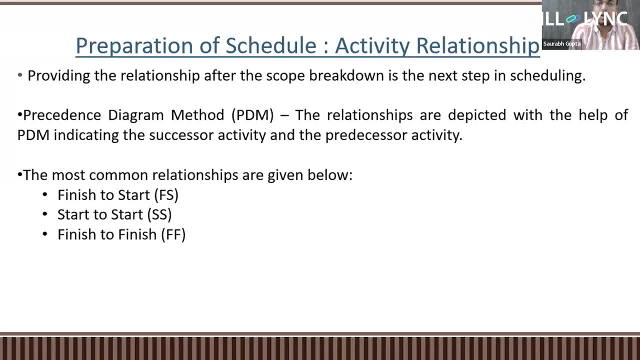 So one relationship is here: finish to start. So finish to start is the relationship which will be given to the 90% of the activities. Okay, Okay, This is the activity like: once you will be completing the excavation, then only you will be doing the concrete work. 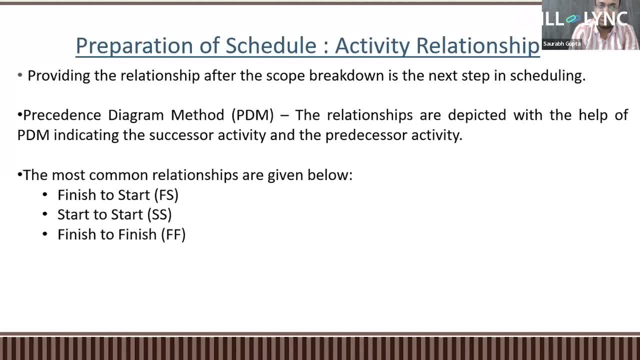 Or once you have completed the rebar work. only then you can do the concrete work. So first previous activity should be finished, Rebar work should be finished. Only then you can do the concrete work. So that is why it is called. 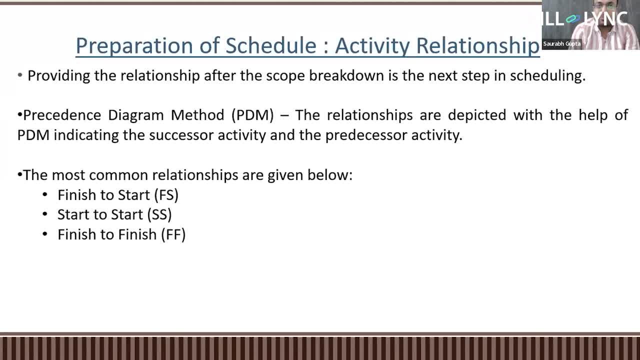 Sorry, Only then you. That is why you Call it finish to start activity. Second is start to start activity. This is also utilized many times. Okay, So what is this activity that start to start? Let's say that we are doing two activities simultaneously. 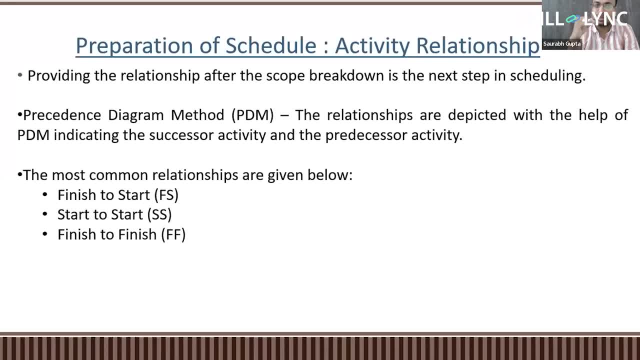 One. we are doing the staging work and we are doing the rebar work, So both these activities can go in parallel. So the staging work Once it has started, Then we can start the rebar work also. it's not like that it will be happening in the same time. 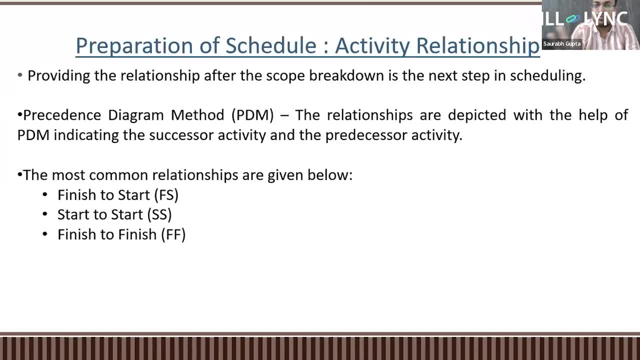 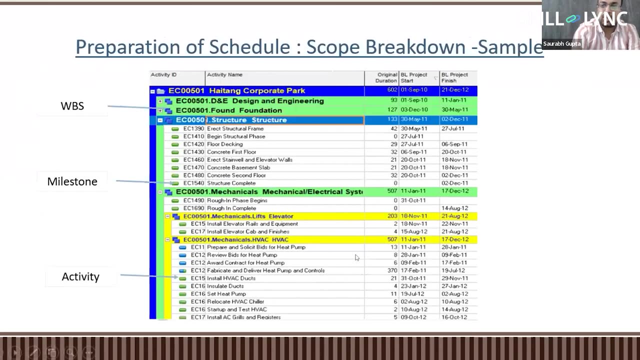 So that is start to start activities. So there are total four type of activities that is available for which we have to provide the relationship among all the activities, But usually for all these activities which you are seeing here. So we will be providing the relationship majorly: finish to start. 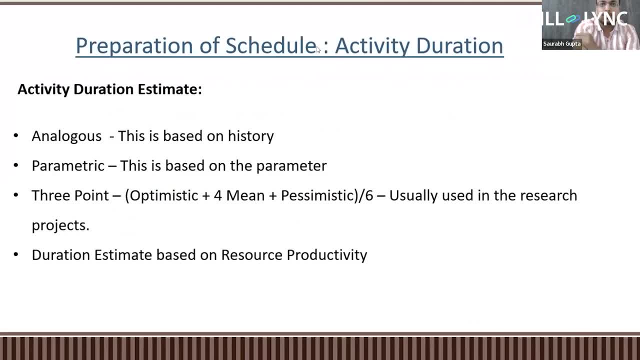 Okay, So Now? So Next thing is the duration estimate. Okay, Simple thing. We are preparing a plan, Okay Now. Firstly, we were having a lot of scope available. We broke down that scope into a logical things which is called WBS. under each WBS, 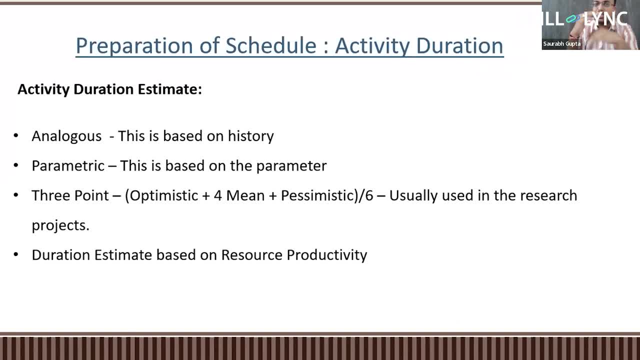 We were having activities. Let's say for this column work, WBS. We were having activities. We were having activities. We were having activities having four, five, six of activities and these activities we have aligned. that first activity was like excavation, then after the excavation, this staging, then rebar, then shuttering. 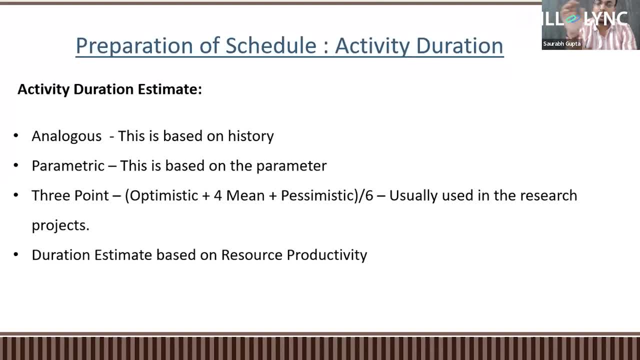 and we have provided the finish to start of relationship and start to start of relationship. Now next thing is we have to estimate the activity duration. Now let's say that if concrete is there, So in one column of this 10 meter height, we are doing the concreting in four. 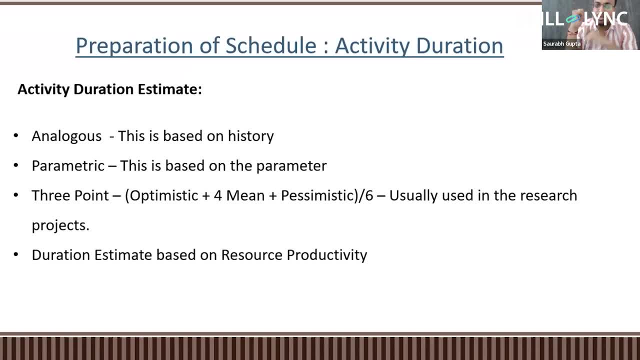 times 2.4 meter in one time. So for this 2.1 meter, how much time it will take? that we will be calculating. So generally we usually estimate the duration with respect to the resource productivity. So let's say this time: 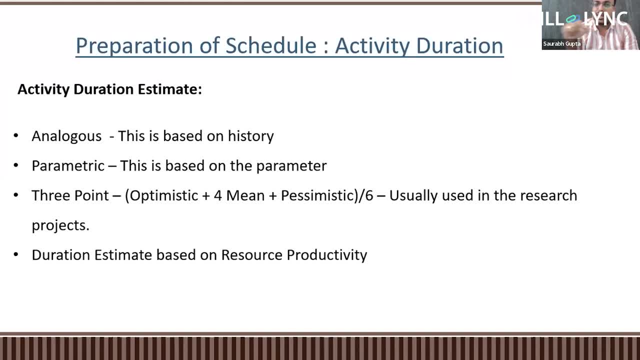 2.4 meter is there. That is the height. we will get to know the length and width and we get to know that, okay, we have to do, let's say, 10 cubic meter of concrete, to do the 10 cubic meter of concrete If we are bringing the concrete from the outside, from. 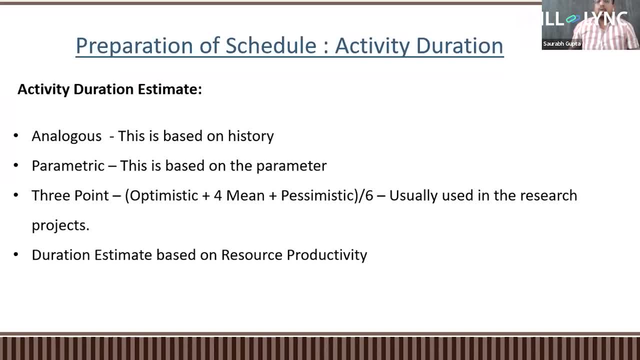 the some outside concrete provider through the mixer machine. So we have the labor, So we have the labor, we got the material. so how much time it will be taking? so let's say that if we will be having 10 cubic meter of concrete and we got 1.5 tms and we have certain labor and mason so they can complete. 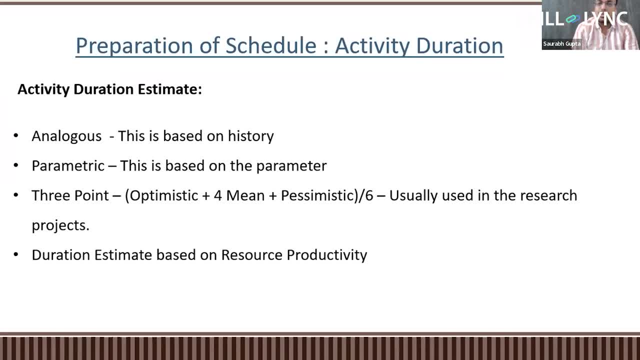 this 1.10 cubic meter of concrete in one day. so that will be the productivity. so we will be providing the activity duration that in this duration we can complete this one level of concrete work of column. so four levels, so for concrete work, four days. so like that we will be. 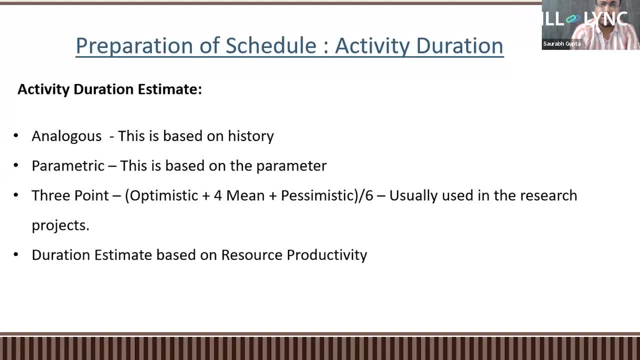 calculating the duration estimate. there are other methods also. so there are other methods also, like this analogous parametric. three point. three point is basically: it is done in the research, just like, because we do not know that how much time it will be taking to complete that activity, so we will be taking optimistic. 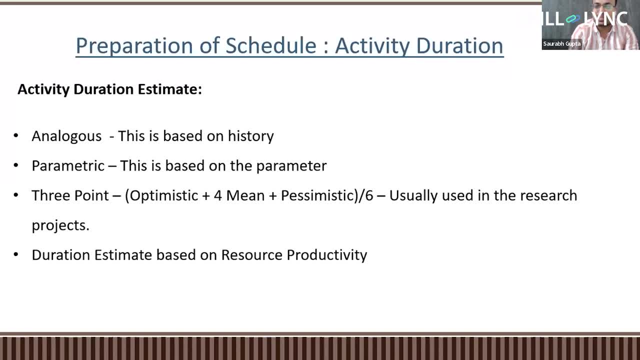 four times into mean and plus pessimistic and divided by six. so that is generally the three point estimate. but usually in actual practically construction projects everybody will be going with the resource productivity. so they will be checking that if we we are having these many resources basically based on their productivity mentioned, we can do the this, uh, this, any any activity in this period. 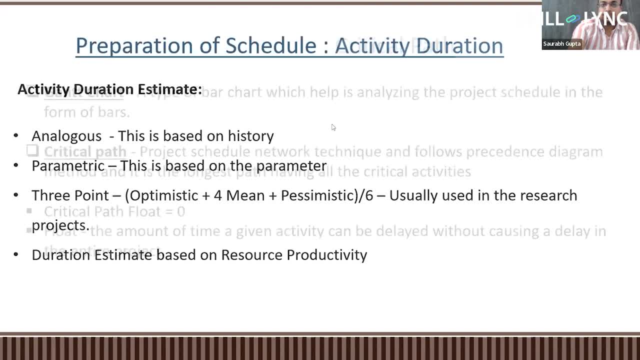 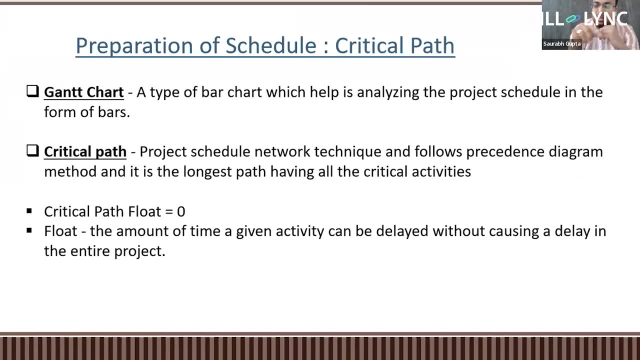 of time. now what we have done, what we have done wbs, we have done activity, we linked each activity, we provided the duration estimate. hey guys, if anybody is having any question, put in the please chat box. so now we want to see the. how does it look like? 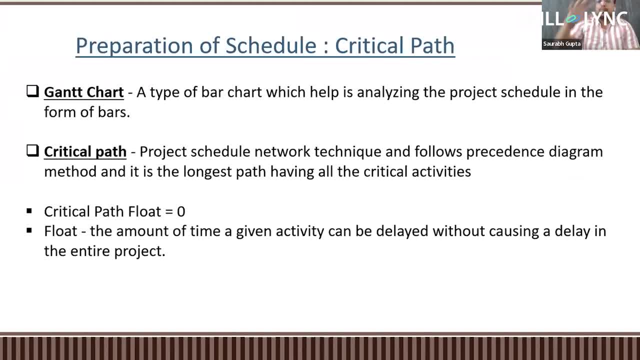 okay, so there will be so many parts available by which we can complete the things. so, before that coming- so there is bar. okay, let's say this concrete activity will be going on for this two year project. it will be going on for six months, okay, so then different, different sections will be there in that. 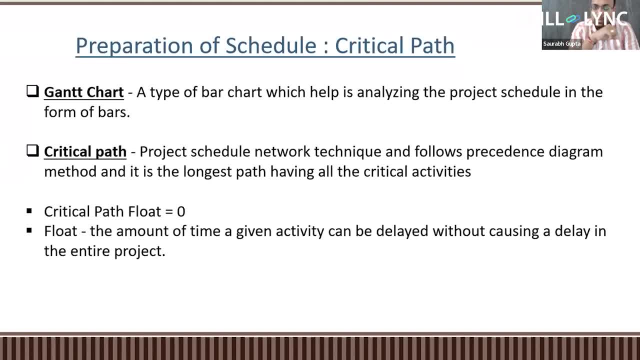 flyover, then each section it will be having different timing so we can take the multiple path. once we'll be, i'll be coming to next slide. then you will be getting more clarity on this. but before that, how do we see the things in a chart? we prepare the bars that this activity will be. 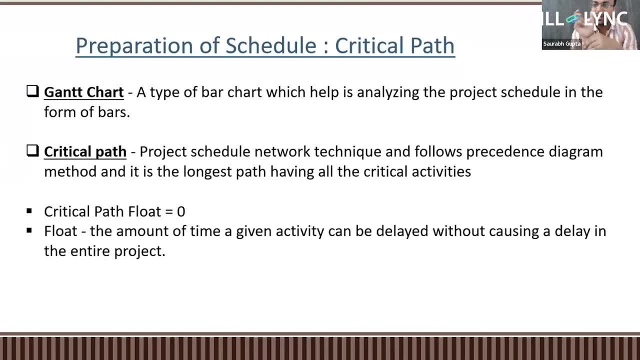 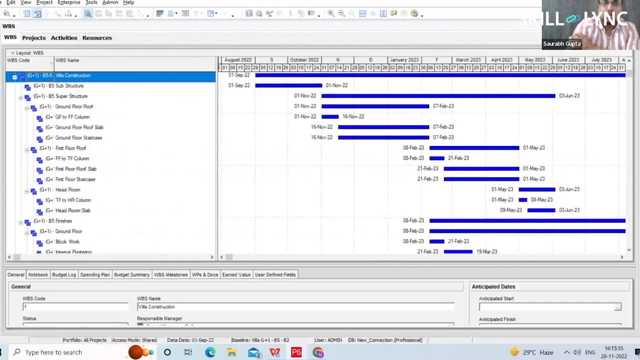 completed in this time period. so that bar will be depicting the time period of that particular activity. so one engineer was there. he his name was gant, so on his name we call it the gant chart. all right, so now here in this blue bars on the left hand side you are seeing wbs and activities. 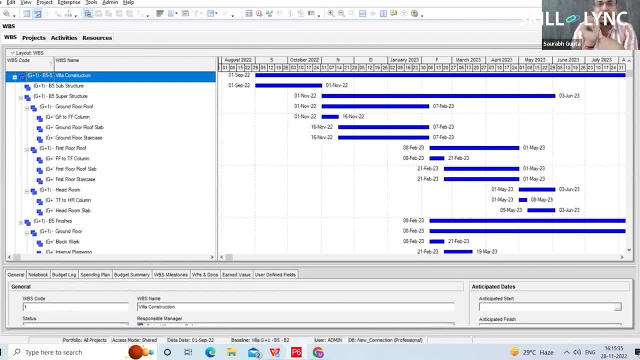 and on the right hand side you can see that first activity, which is the substructure it started on. it is planned to start on 1st september 22 and plan to complete on 1st november 22. so that bar is the, it is the bar, so this bar is. 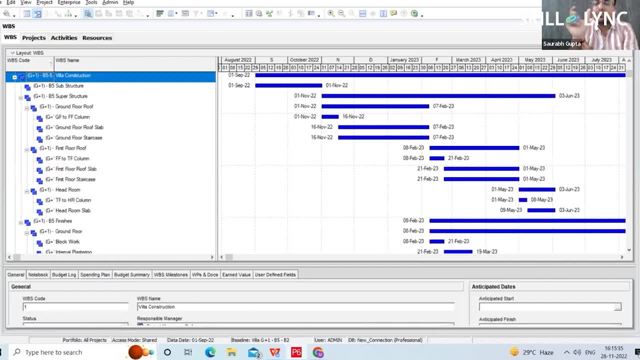 scaling the time, that in this time period this activity will be completed. so it is you know, rather than you know reading the things. it is very easy to look at the bar and to check the things. so this entire on the right hand side- this you are seeing on the primary screen, left hand side- we 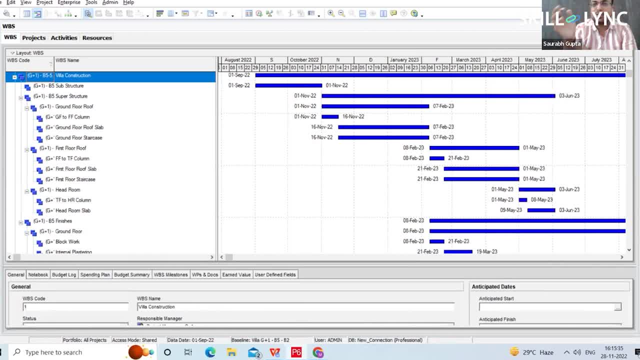 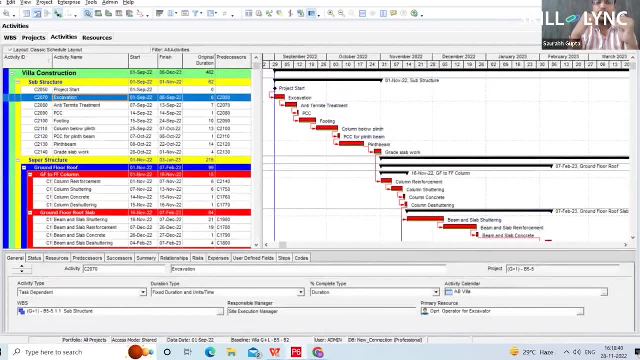 have created the wbs. then activities, right hand side. you are seeing the timeline with respect to the bar charts. now, next, we have aligned all these bars, okay, we have provided the relationship, so whatsoever you are seeing on the red color, okay, so that is the critical path. 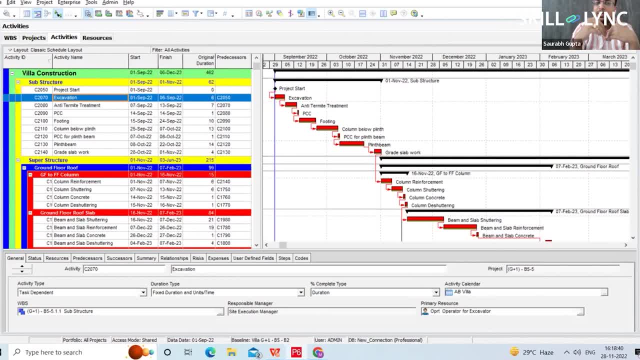 so now, what is critical path? so critical is the critical path is the path. if any activity on that path will be delayed even for one day, then the project will not be completing on time, it will be delayed. so that is why, out of so many activities and paths, we have to give ultimate focus on the activities which are lying on the critical path. 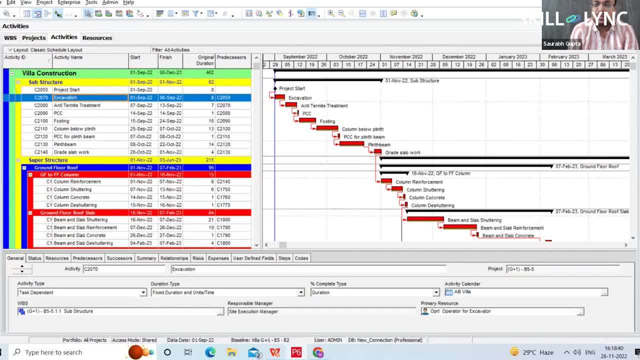 so critical path is generally defined that the float of the critical path is zero. now, what is this new terminology float? okay, we'll be discussing so. now we have understood that one path is there which is very critical. okay, so if any activity will be getting delayed on that path, 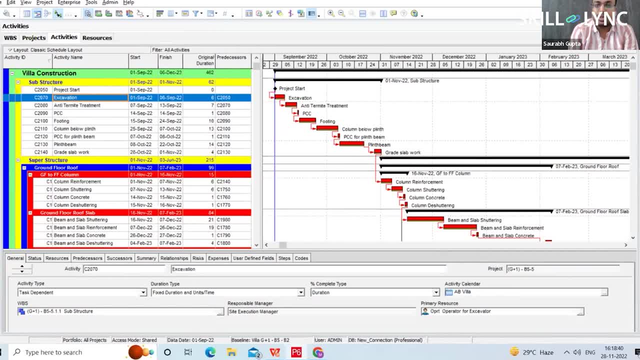 that then the project will be getting delayed. okay, now, how do we define a critical path? okay, so critical path: we have defined that if the float will be zero, then that path will be called the critical path. so float is basically the time duration by which we can delay that activity. 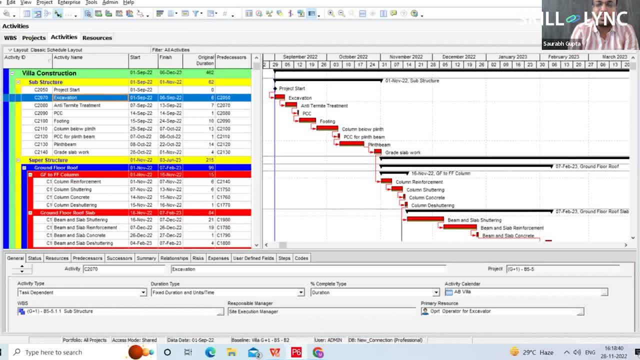 let's suppose in this, on the top, you are seeing the excavation. let's say that if we can extend the excavation by one day from seven days, which is mentioned in the original duration, so if we can delay this excavation by seven to eight days, so if that seven to eight days. 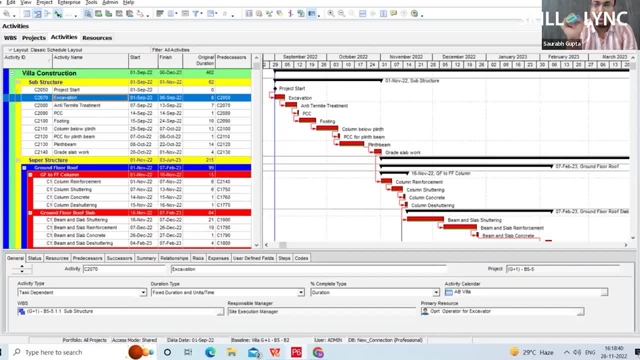 the project is not getting delayed, then it is not on the critical path. but if the float is zero, zero, okay, if we cannot delay this activity by even one day, so that activity is called the critical path activity, all right. so ultimately the thing is, we created wbs, then we created activity. 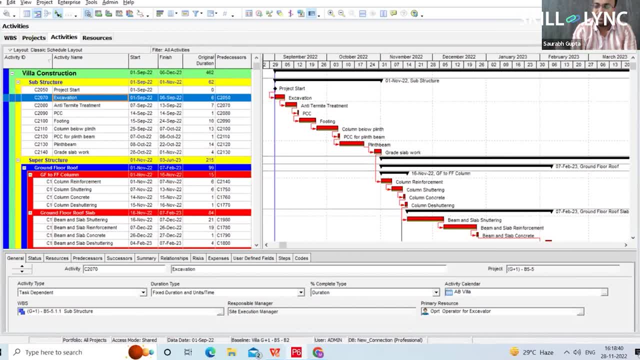 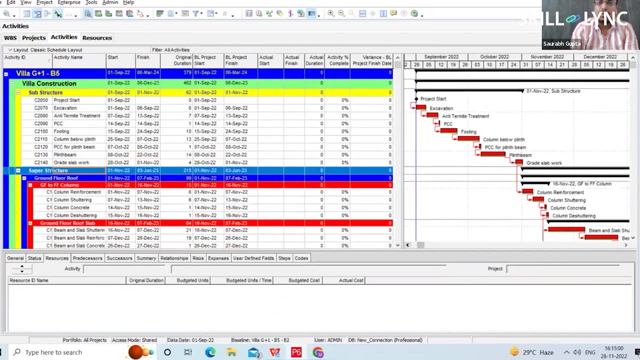 after created activity, we provided the relationship to each activity. after providing the relationship, then we provided the duration. so, after all doing all this, we got the critical path. we'll be getting so many paths- other paths are also there- but we get the critical path and we will be following the project with respect to that critical path. 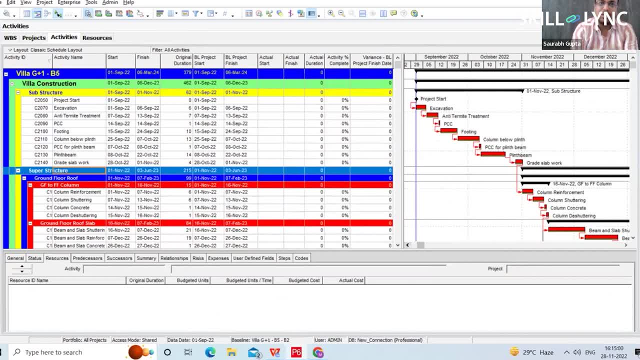 so here you can see that on the left hand side, activity name are there. start and finish date are there. then we will be having actual start and finish date. once we will be monitoring this project during the execution days, then we will be having the actual start and finish date. all right. 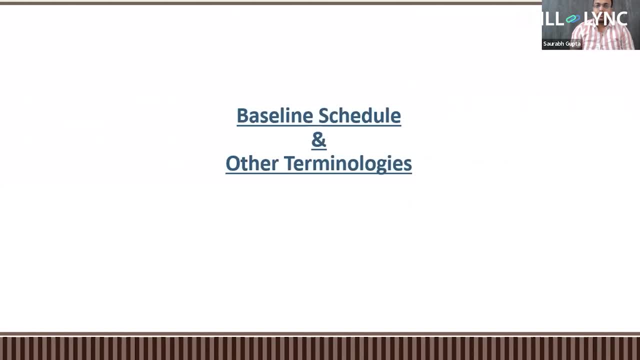 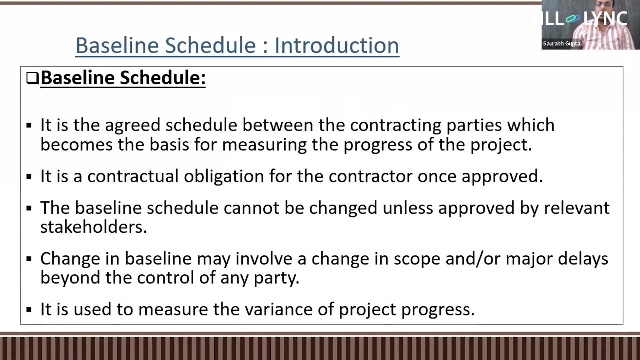 now we have prepared the schedule. okay, now we have to see that. what are the other time terminologies? okay so? uh, now it's not like that. you have prepared the schedule and everybody will be accepting it. okay, so, because there were two parties, one was the client, second was the contractor. 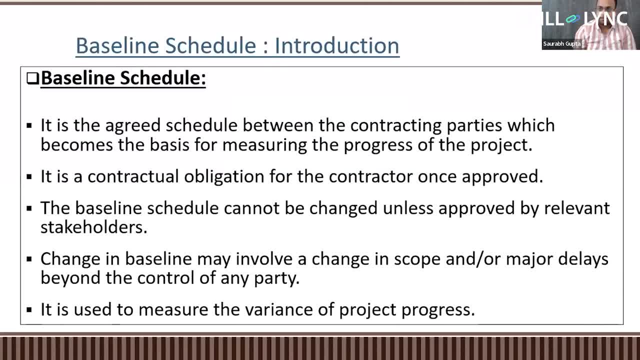 so sometimes what happens? until and unless the client does not accept the schedule, he does not have a faith that whatsoever schedule you are preparing and he does not get a, you know faith that or believe that you will be completing or he'll be asking to change it. so until and unless both will not get agreed, 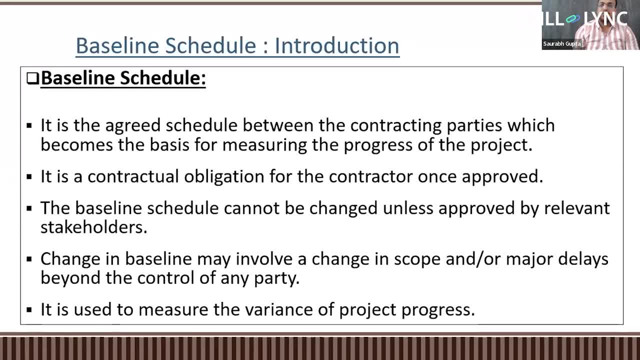 so that will not be called a baseline schedule. if the client will be accepting it, then it will be called a baseline schedule. then according to that a baseline schedule, the progress of the project will be tracked and so many times what happens? the top management asks the project team or the planning engineer or manager. 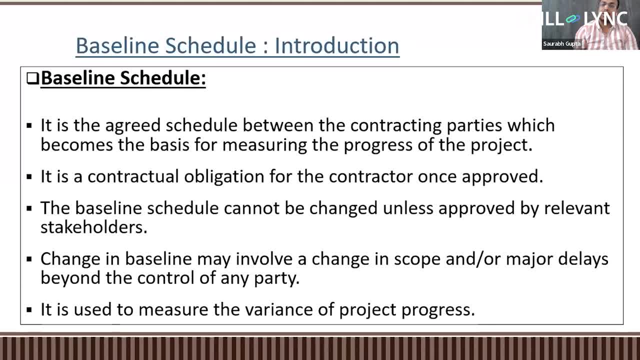 to prepare a schedule, then they approve the schedule, the internal management even so. that will be called the baseline schedule. so basically, baseline schedule. Baseline means that one thing has been finalized or it has been made the base that with that particular base or reference the entire project will be tracked. all right, 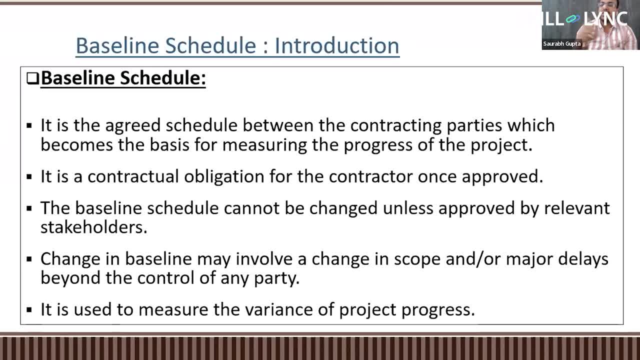 Because the planning engineer prepares a lot of revised plans during the execution. Sometimes the project will not be happening with respect to the plan. Usually it happens The project gets delayed, So therefore the planning engineer will be preparing a catch-up plan or revised plan. 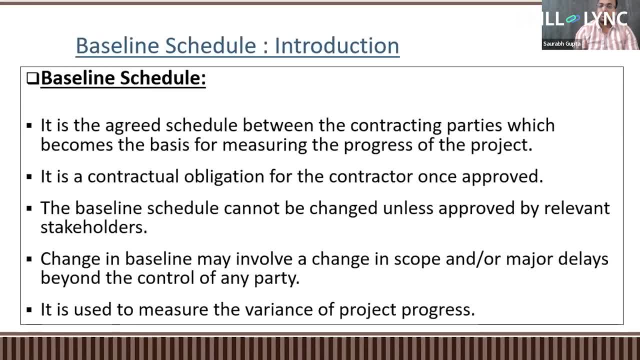 how they can catch up the things or if the project will be delayed, how much time it will be delayed. But at the end, either the top management or the client, they want to check the project with respect to the baseline schedule where we are standing. 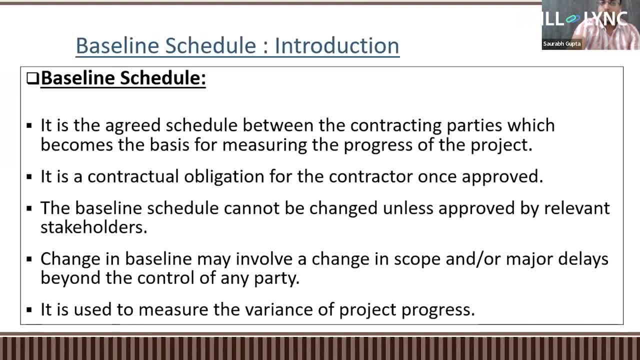 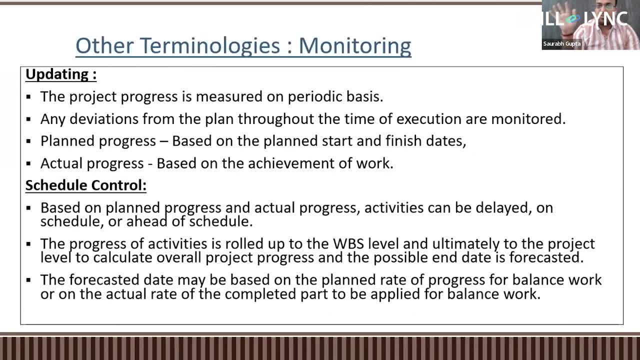 So this is the basic purpose of baseline schedule to measure the project progress report. all right, Next thing you know now we have done the Project planning. Next is the execution. It took few time. Project planning engineer have done every activity. 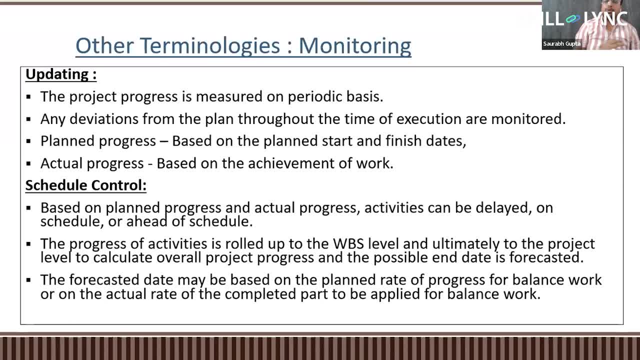 Now, with respect to that project plan. the execution people: they will be doing the execution activities at the site level. So, on daily basis, what happens? The site people: they will be updating the daily progress report. I have done this. cubic meter of concrete. 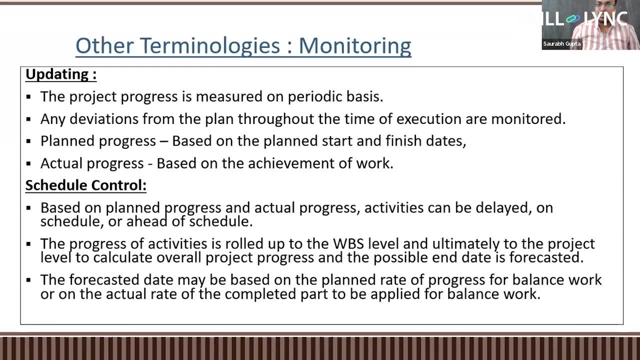 This much work of shuttering is done, This much work of reinforcement work is done, This much work of road work is done. So everything they will be making The templates that has been provided and set up by the company, and they will be providing 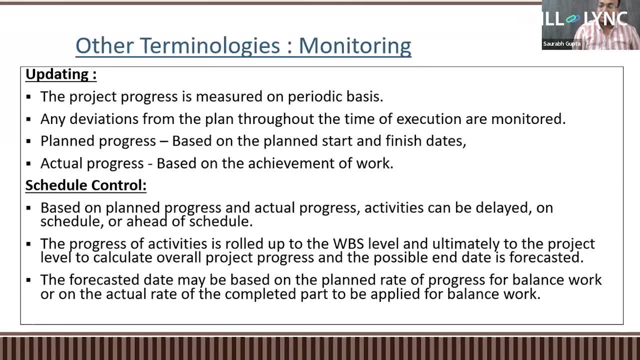 the daily progress reports to the planning engineers. So these planning engineers, they will be updating that project progress report with respect to the plan. So what they have done, they prepared the plan of two years, then they'll be broken it to monthly, then daily basis. that this on. maybe tomorrow they have to do the yesterday. 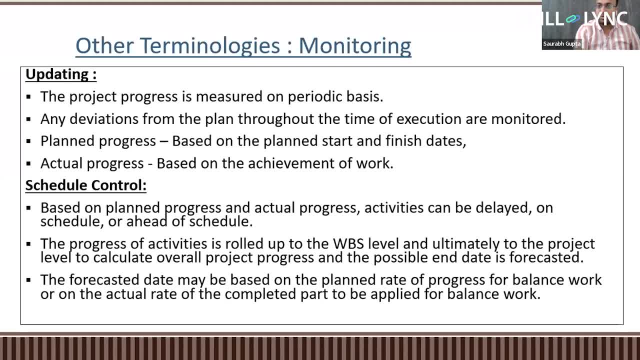 they planned for doing the 50 cubic meter of concrete. Then the actual site It will be coming. It may be 50 cubic meter, It may be 40 cubic meter or it may be a 20 cubic meter. Maybe the TM was not working. 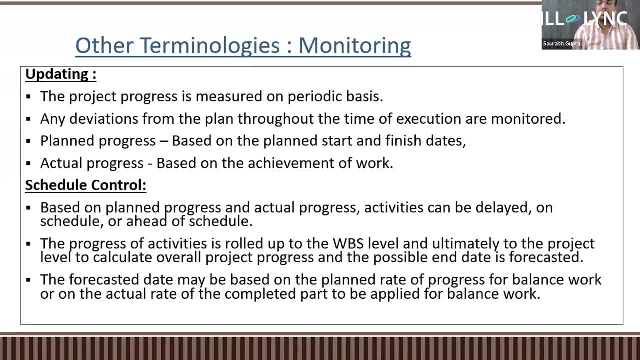 Maybe it started raining after lunch, So then they will be updating the progress of the project on periodic basis. Then, once this activity is done, off the updation. then second thing is to control the schedule. Now we have the baseline schedule, which has been fixed either by the client or the top management. 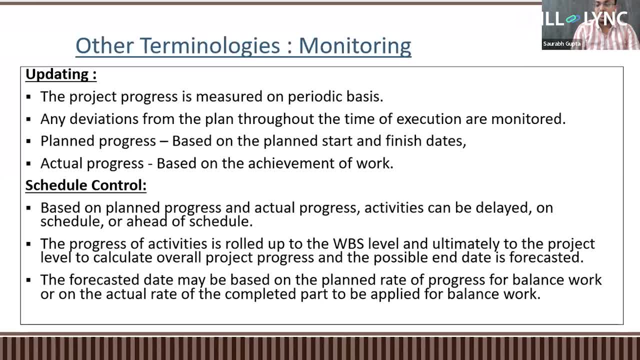 We are getting the updates on daily basis. then we are checking on the periodic basis- Usually it is weekly or monthly basis- how we are progressing. then we are checking that suppose in this month we have to do 1000 cubic meter of concrete, whether we did 1000 or 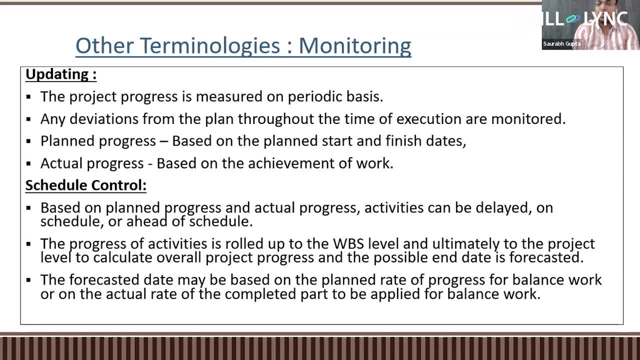 800 cubic meter, let's say for pipeline project. we plan that we will be completing 50 kilometer of pipeline. Okay, That was the plan, But we could have completed only 25 kilometer or it may be exceeding sometimes that we have. 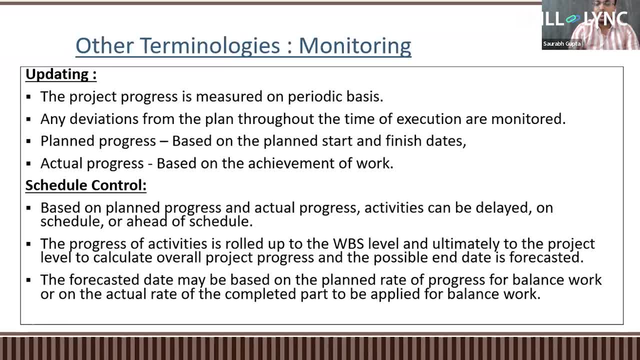 completed 60 kilometer of pipeline. Okay, So likewise, they will be evaluating with respect to the baseline. If we are lagging with respect to the plan, then the planning engineer will be making the revised plans So once. so they will be doing this entire activity till the end of the project. 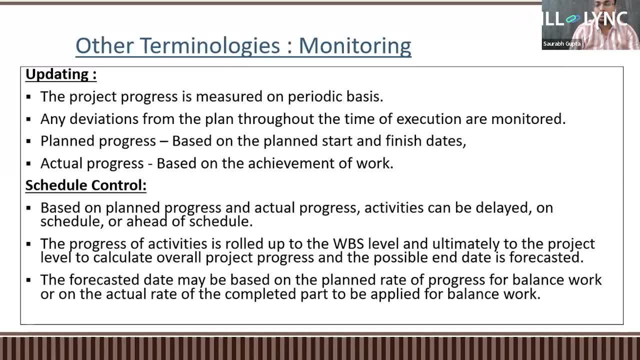 All right, So this will be the Schedule control. So three parts are there. One: they will be planning during the initial phase of the project, then they will be updating during the entire course of the project, during the entire execution process. then they will be controlling. 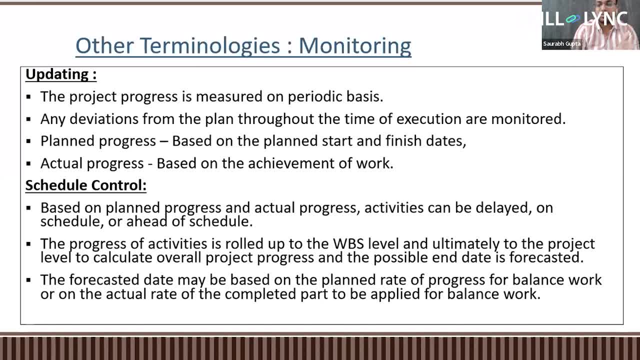 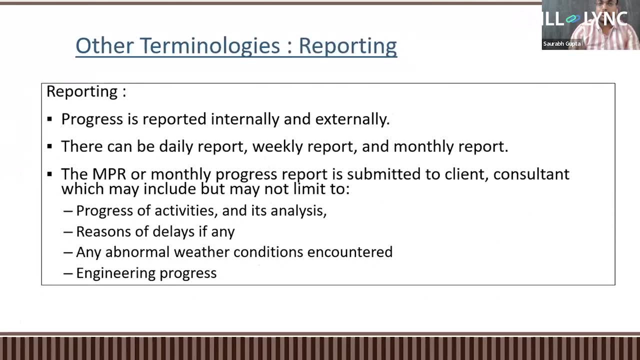 the schedule during the entire execution process, whether the project is happening with respect to the plan or not. if not, then they will be making the revised plans on regular basis. Okay, All right. Last thing is the reporting. So this is very important aspect, because you know each and every person in a company. he's reporting to someone. 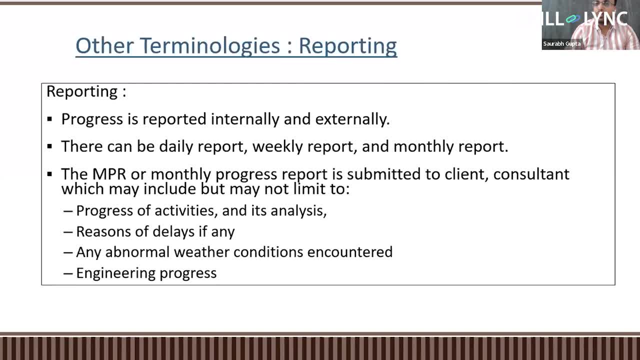 Even the CEO of a company. he's reporting to the stakeholders. They may be, uh, stakeholders, and they may be having shares in that company, or to the public limited company or anything. So that is why reports are very much of importance. So what to do if it is raining continuously, so that work is affecting, so that work is not going according to the schedule? 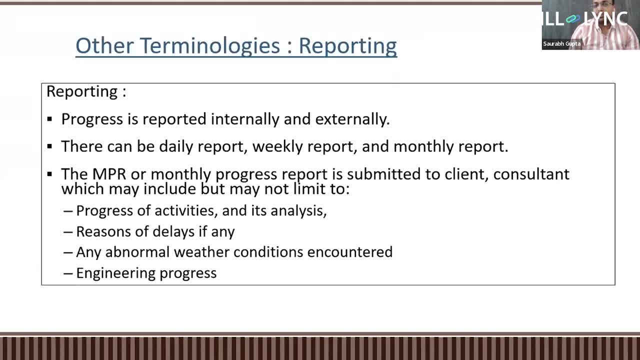 Yeah, that's a fantastic thing. So now I'll, uh, I'll tell you very uh basic thing. So once a good planning engineer knows the weather conditions, so he has planned his entire project and scheduling with respect to the weather conditions. 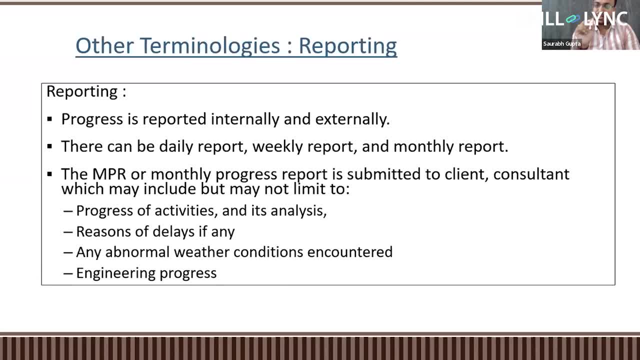 All right If he has not planned Considering the weather conditions, So ultimately his plan is going to fail. Second aspect: there are uncertain, you know, rain or incidences, some, uh, you know uh, any anything which is uncertain or which was not, as per the repetitive, like rain happens in. 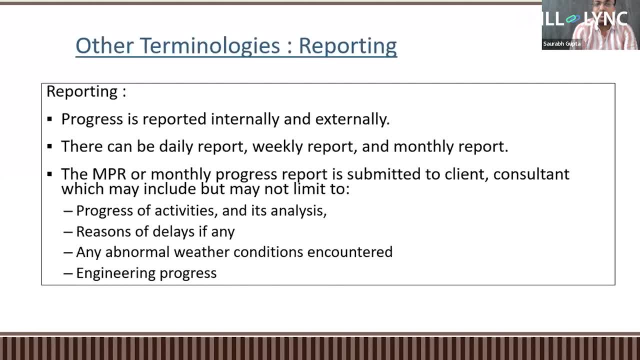 north in July and August, but uh, it's raining heavily, Let's say in this month of October, so that they have to inform to the client and then the client will be Giving them extension of time. So those kinds of clauses will be available in the contract. 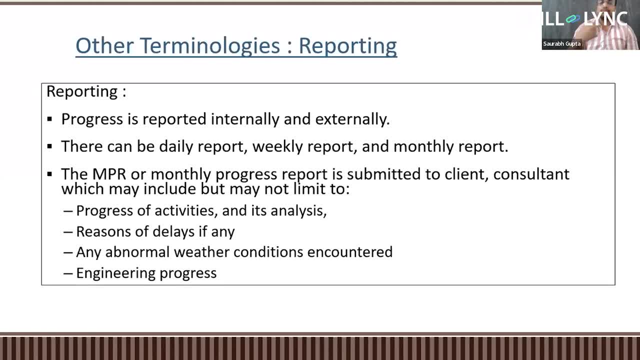 Okay, But it should be. it should not be regular, So it should be very uncertain event, All right, So that is part of the planning. Yeah, Same way it goes with the local effects. So all right. So now let's come to the reporting. 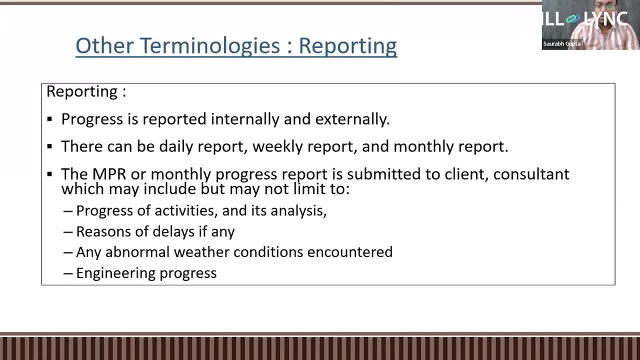 So reporting is very much important. Okay, Either Uh a planning engineer has to report To the boat, He has to report his uh project manager, then a regional offices, then top management and externally he has to report to the client. 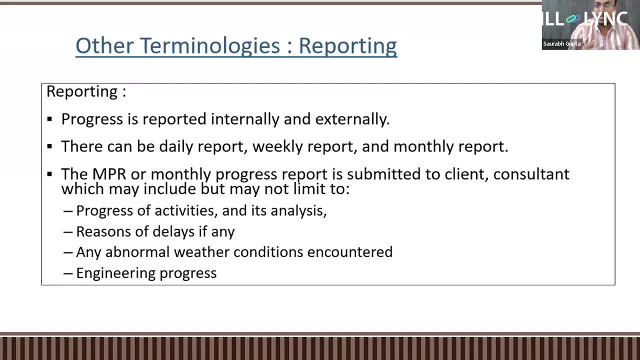 So therefore, he'll be making a lot of reports. He's making daily reports. Uh, he'll be getting the progress update from the site. He was having the plan which he has prepared. He'll be making daily report, weekly report, monthly report. 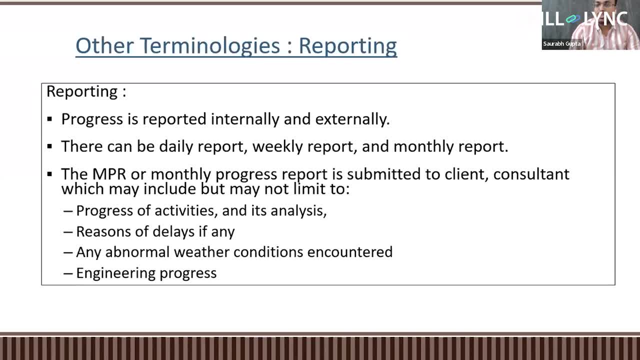 Uh, likewise he'll be preparing, So in this monthly progress reports generally, they'll be preparing all these aspects. What was the plan? What has been achieved? If any delays there, what are the reasons of that delay? Any abnormal conditions were there? 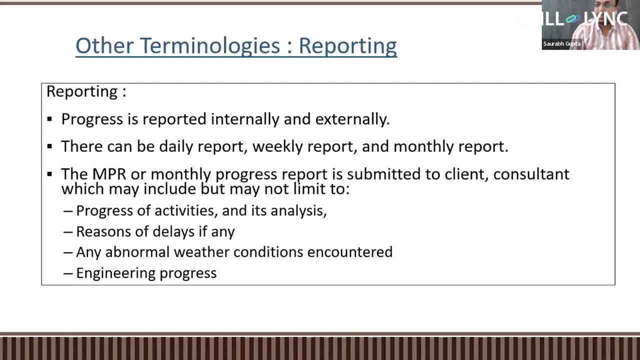 It may be local conditions, It may be. you know weather conditions, It may be strike from somebody, It may be you know political conditions, It may be like pandemic was a thing. Okay, Then they will be putting, So they'll be putting a lot of things and they'll be mentioning how this everything is going with respect to the 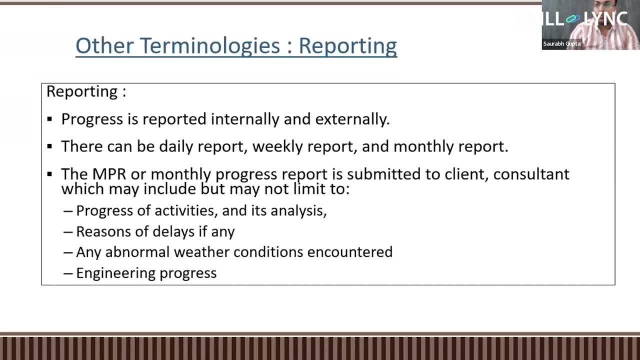 Okay, I'll tell you. uh, you know my first task in my GDT period, graduate engineer training period in L&T construction in 2012,. I was sitting on a desktop and for each month, at the end of the month, I have to prepare the monthly progress report. 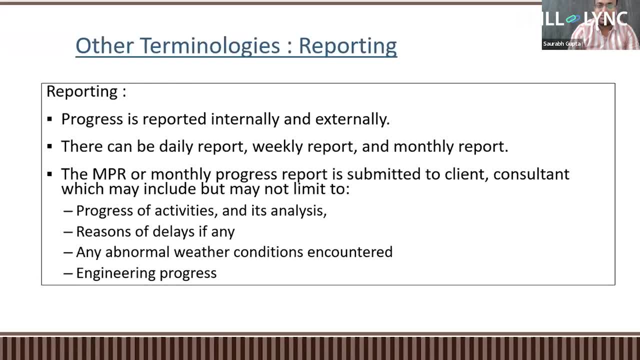 So daily, once I was coming to the office, I was making daily progress report. I was sending it to my project manager and copying it to the construction managers. Whatsoever the progress I was getting on at the end of The week. on each Monday I was preparing the weekly reports and circulating to all. 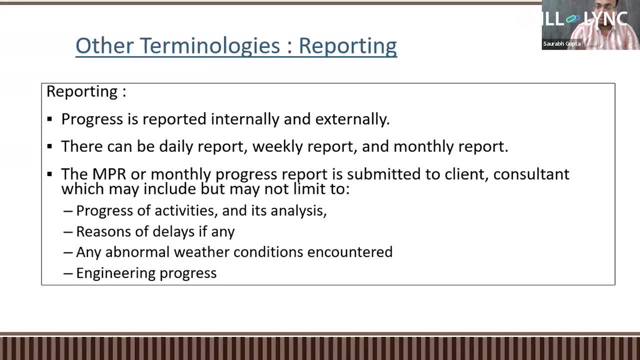 And at the end of the month then I was preparing the monthly progress report and that monthly progress report was going to the client And then it was going to the uh top management regional offices. So that was my first task which I was doing in the company. 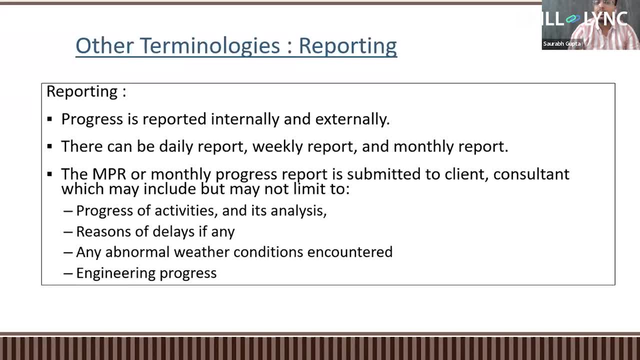 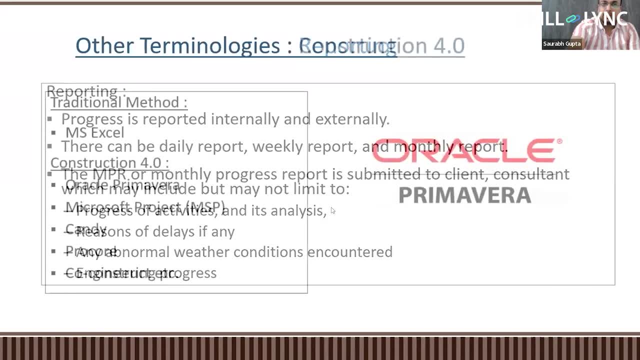 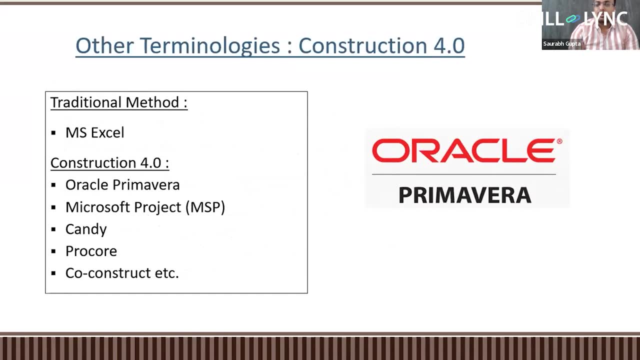 So by doing this task, we were doing the planning and monitoring, reporting. reporting I was Doing all right. So now we have to understand that you know we are doing a lot for this thing, but how to do this entire planning? 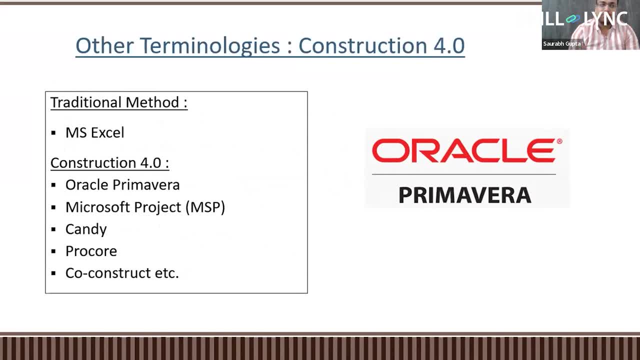 So earlier what was happening? People 50, a hundred, 50, 70 years back that they were doing on the paper. Now, last 20 years back, they were doing in the MS Excel. but now we do have softwares. 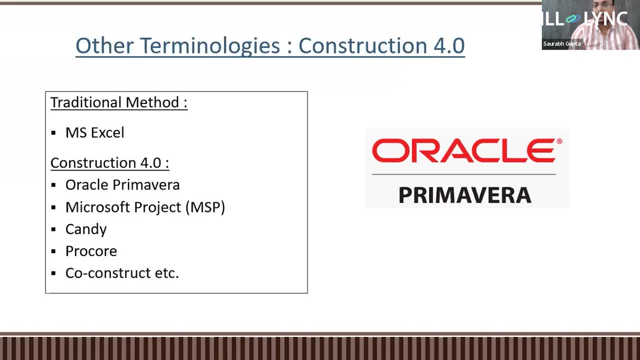 Those softwares have been provided by the companies, software companies based on The requirement by the of the construction industry. So one of the major software is the Oracle primary data. You know why Oracle primary is important? because it contains all the techniques to plan and monitor the entire project. 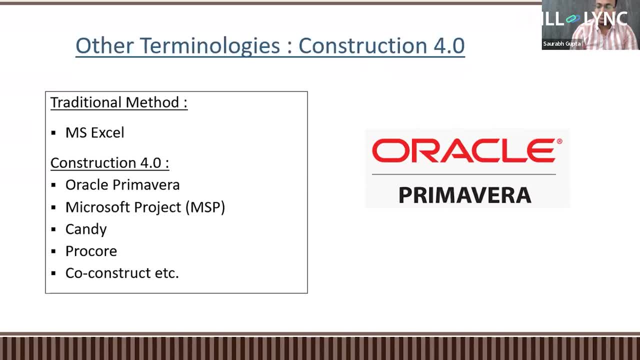 Okay, Because a project is having a time aspect, They have a resource aspect, They have a risk aspect, cost aspect, So everything can be integrated and with the help of this primary, Yeah. So what happens is that Oracle primary data software, they'll be getting critical parts. 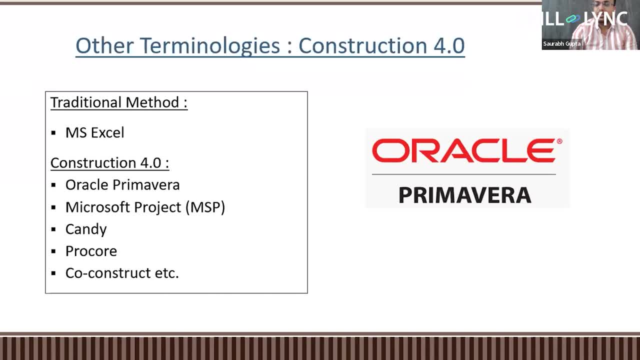 There'll be. these softwares will be helping them in managing. You know generally what happens. you know what we follow, the Gulf, what the Gulf is doing and Gulf follows what the Europe and us is doing. So now, generally Gulf was doing the Oracle primary data from last five to 10 years, or more than 15 years, starting from the 2000.. 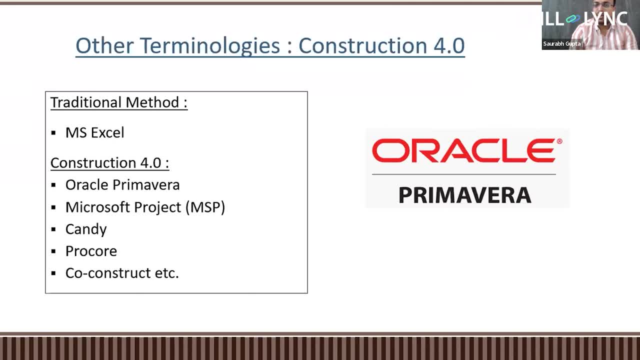 So now we are following the Gulf in the same fashion. know they are asking the persons to be proficient on the oracle, primary. so if you will, if you will say for the gulf, then definitely they'll be asking only one question, whether you know primary or not. 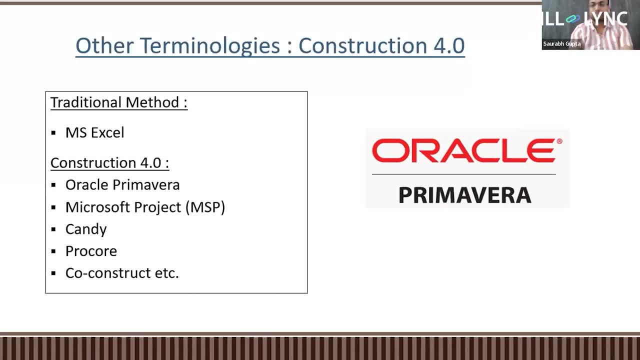 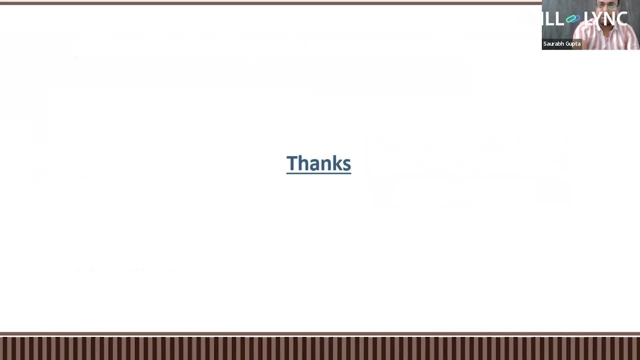 even in india, every company now is demanding for the primary data. so, guys, this is all uh with respect to the technical session whatsoever we have covered here. yeah, uk is using primary. yeah, every country is using primary. so you know, this is the uh as on date, this is the most proficient software. uh for the, you know, planning and monitoring purpose. 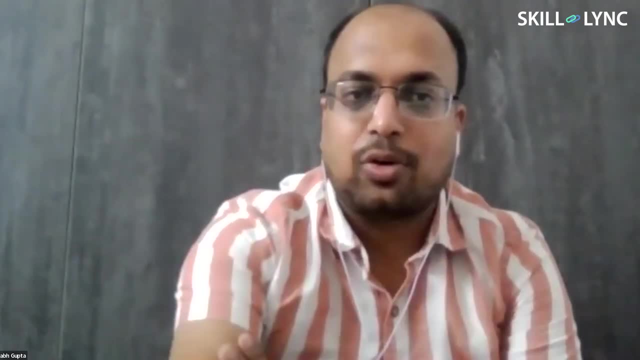 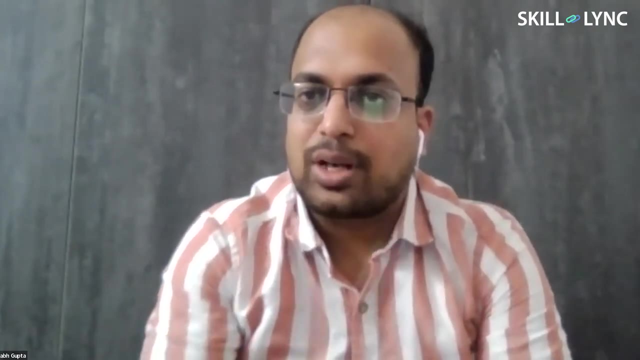 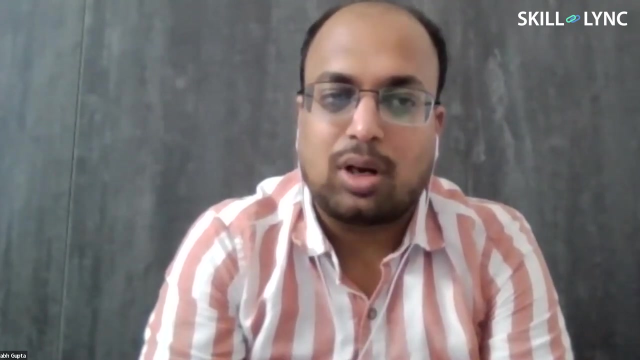 so, yeah, guys, uh, now, if you have any questions or any sort of query, uh, don't be hesitant. and we ask. so i'm a final year student. please say me, uh, which coaching should i take for job after completing civil engineering? okay, so, uh, you know generally what happens. even that happened with me. 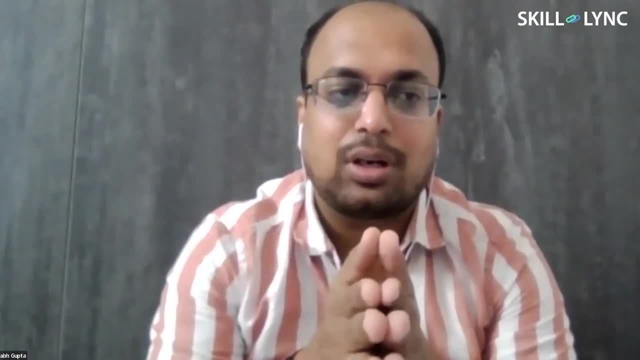 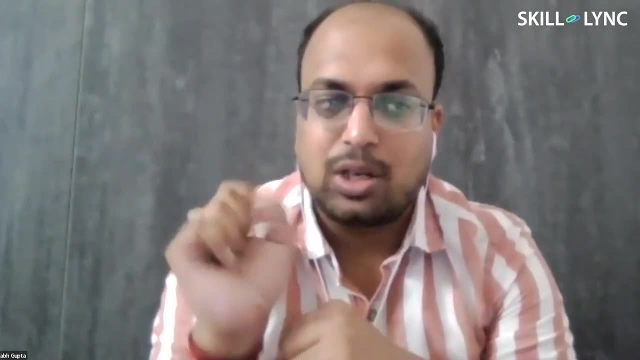 uh, what we do in the engineering that is, you know that's not much industry relevant. so then each company will take you as a graduate engineer trainee. so why do you? why they don't call you as a trainee? because they know that we have to teach this guy everything. 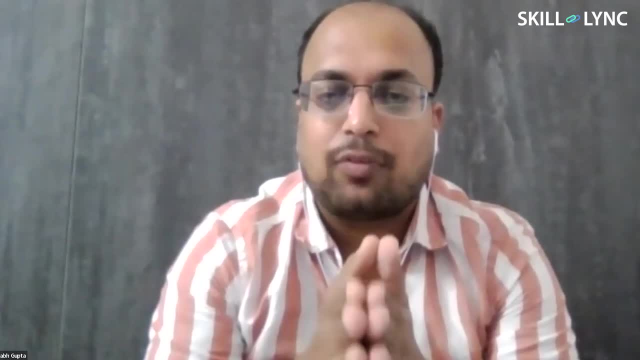 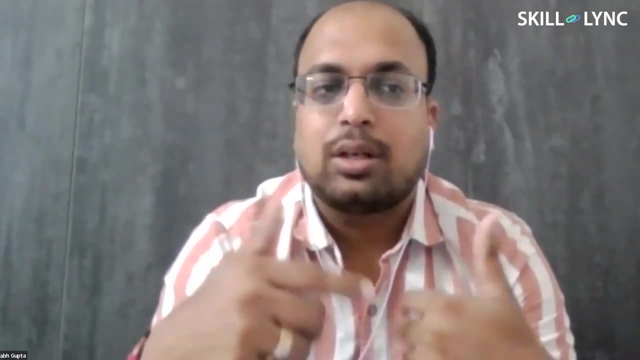 into, how to go into that company, so that, therefore, we should know about the techniques and everything you know, like in construction, project management, how to learn the construction, how to do the construction. so, therefore, we should know how to manage the time, how to manage the cost, how to 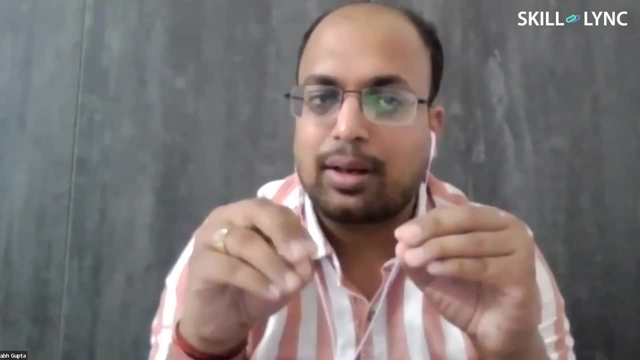 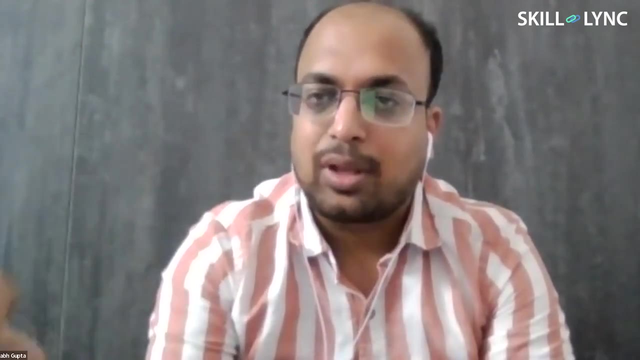 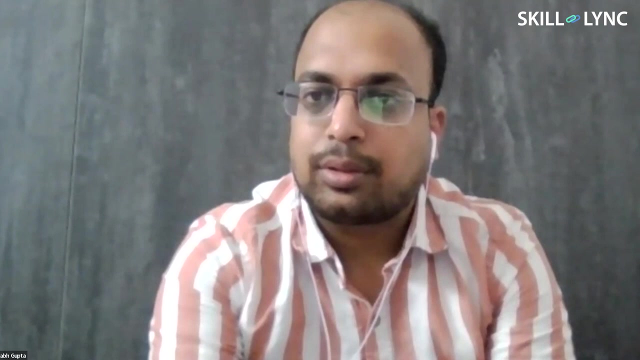 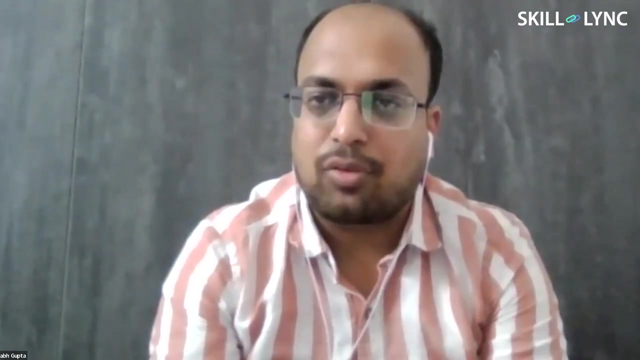 manage the contract. so if you will be knowing those things even now at a college final year, so you will be having a better aspect to compete with the other persons, great uh. so yeah, oracle primary: see it's. uh, anybody can download it. there is a method for it. 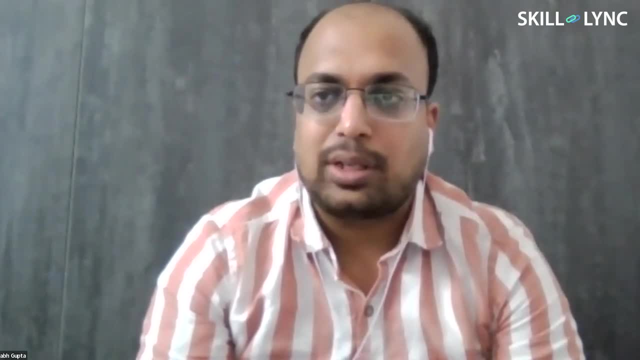 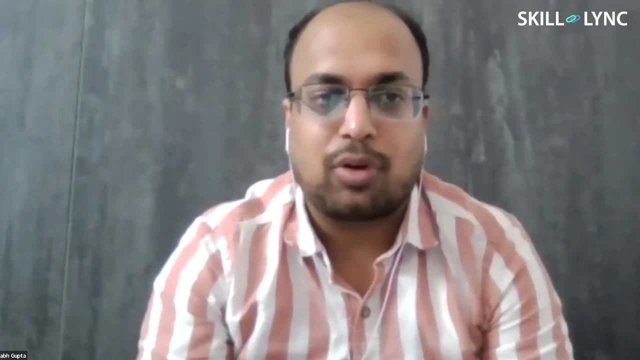 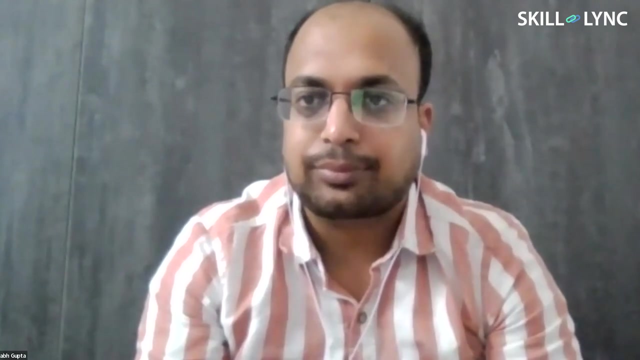 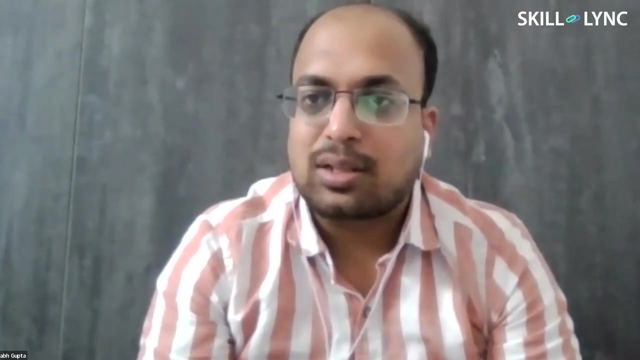 uh, you can utilize it for three months. so it's a very expensive. software companies are using the software and they are paying two lakh rupee per person. but, uh, for a trial person, trial purpose and study purpose, the three month it's available, uh. so, uh, somebody has asked that he's a fresher and 1.5 experience in realistic construction. 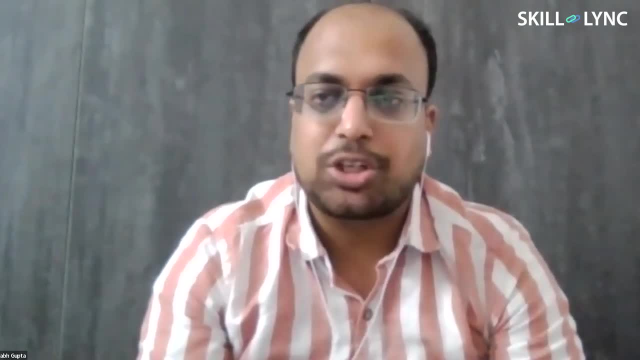 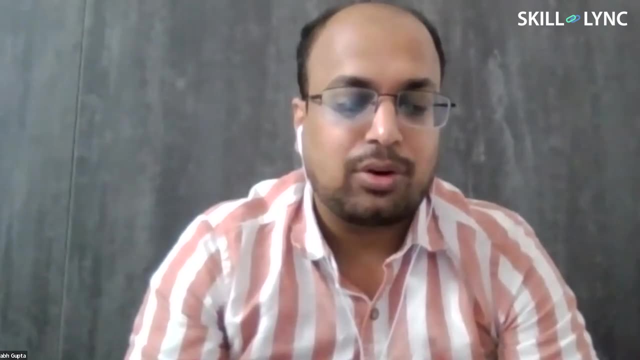 sector, how he wants to switch to the infrastructure and he wants to switch to the infrastructure sector. see, i'm not sure that you are a site engineer or in which particular role you are working. so that is why you know there is a very simple thing: if anybody wants to progress in, 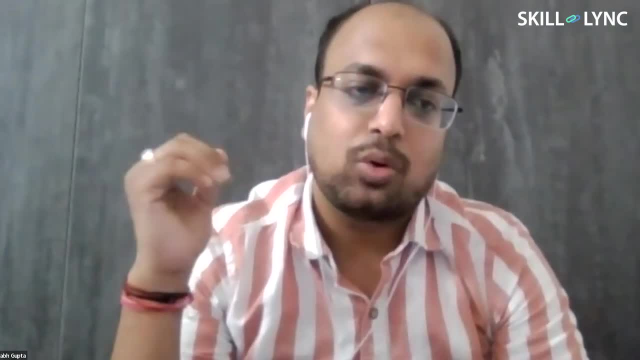 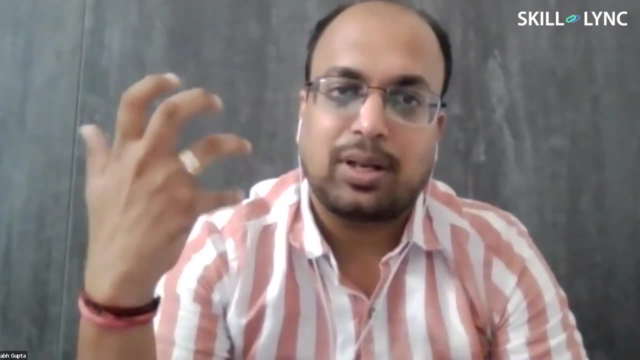 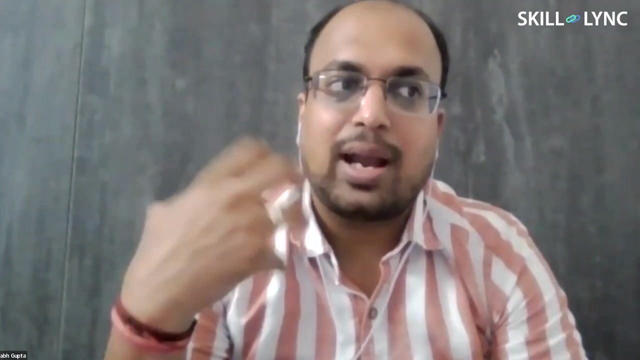 construction industry under the construction management, ultimate goal is to become the project manager. so to become a project manager, they should know project management. you cannot become a project manager initially, even after learning this. it takes a lot of time, but you know, today i had a call that 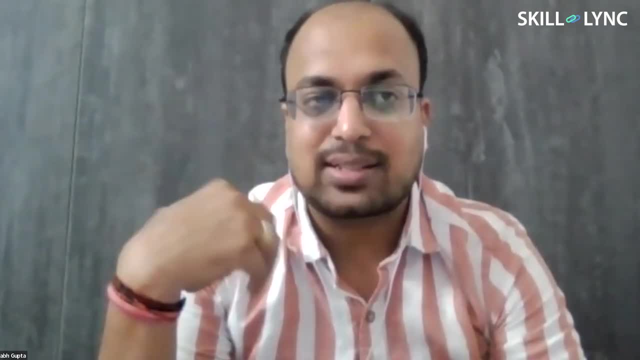 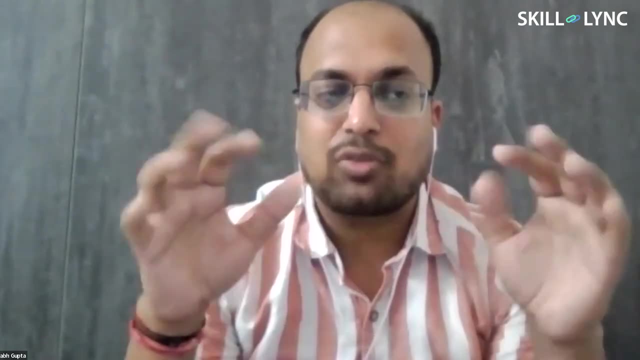 guy was 46 years old, he is working as a site engineer from last 22 years and now he wants to learn construction project management. so this is just one of the rare example i'm giving you. so at any point of time, they have to learn construction project management because 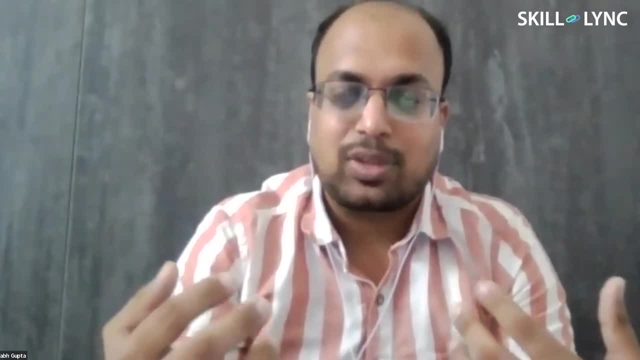 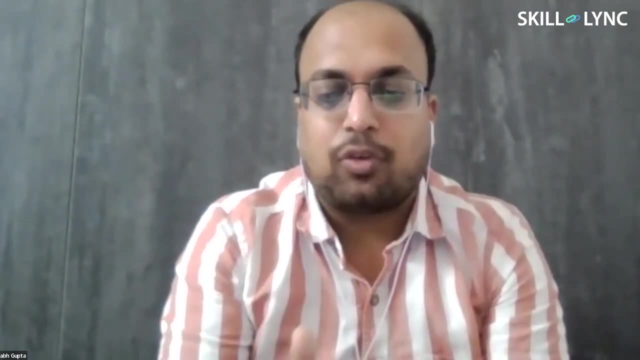 you know what does this project director or project manager does? simple thing: they work for the money. every project is there for money, only to how to gain the profit. so therefore, they have to learn time, cost and score. they have to learn time, cost and score. they have to learn time, cost and score. 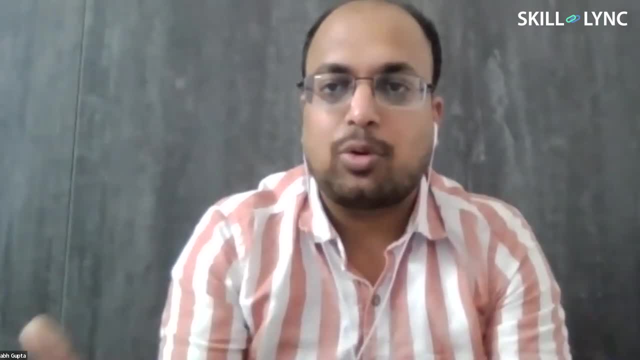 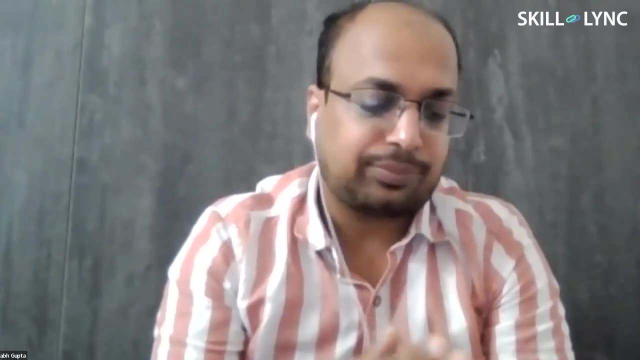 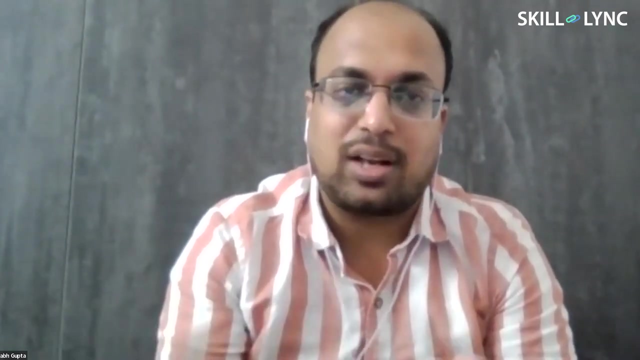 scope management. if they will be. knowing these things, you can. you can achieve anything in the uh. you know your career, so the. if you are a student third or final year, you should learn it now. then you can focus on other things in during your profit professional level. if you are in the 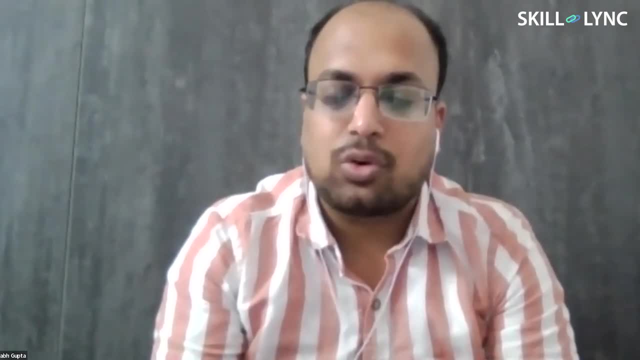 initial phase of your uh career. so if you are working as a site engineer or any anything, you should learn project management, because if you will be learning now, you can immediately grasp the things. uh people have learned this thing and they have moved from site engineer to the planning engineer office role that i have seen in last couple of months. 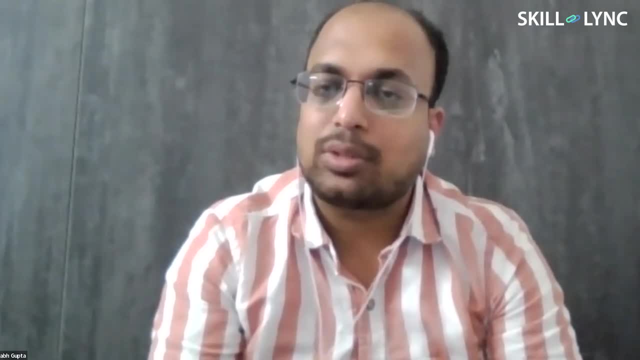 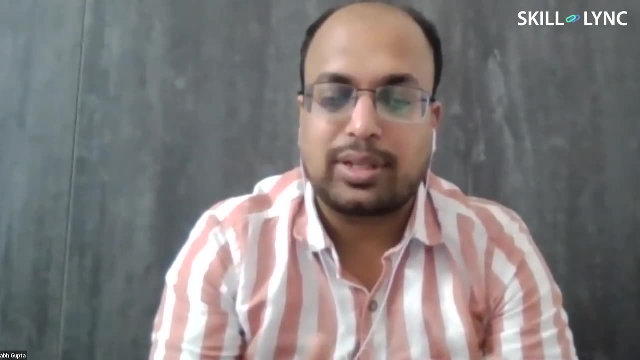 how can we learn to operate primary without actually working on a project? okay, yeah, that's, that's a good question. see, sometimes, like in skill link, what, what is available here? so there's a program available here. they provide the self-paced learning program and similarly they provide the 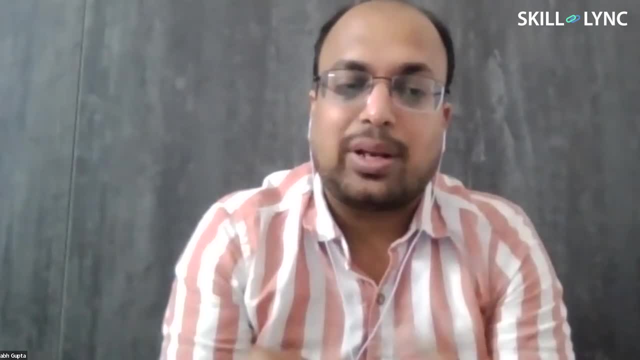 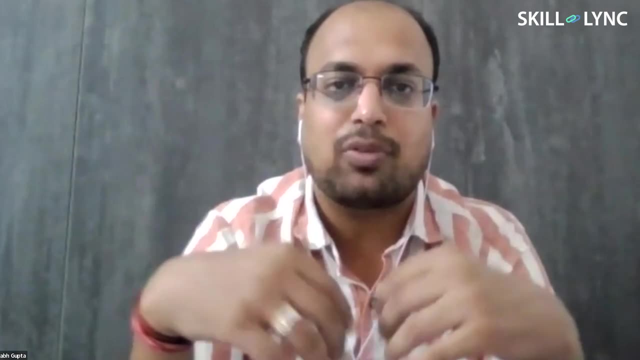 learning project in order to be able to do these kind of business, and so that means they provide the self-paced learning program and also they provide the self-paced learning program, and so they provide the step by step learning program for this, and also they provide the professional 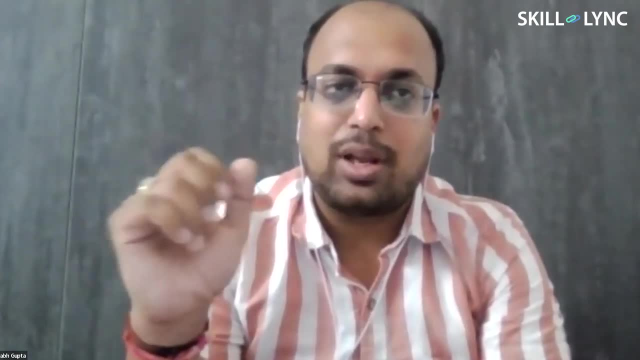 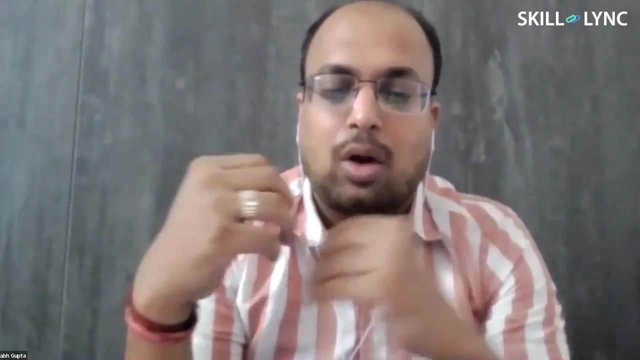 learning program in order to be able to do all the other projects. so this is what we are talking about in the field of digitalization. and then the next one is the third one, which is the um. the third one of the integrated technical projects doesn't change like from one to the other. 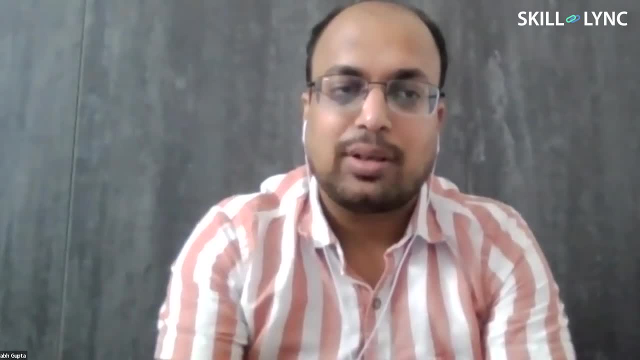 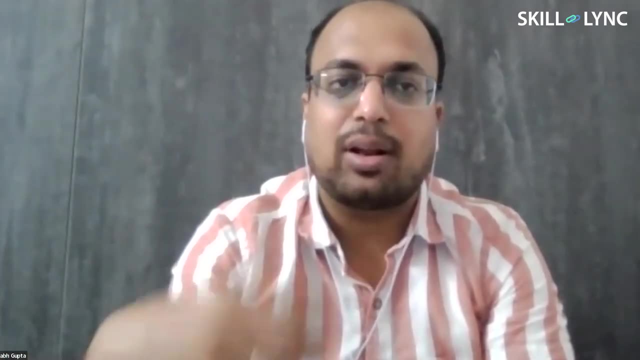 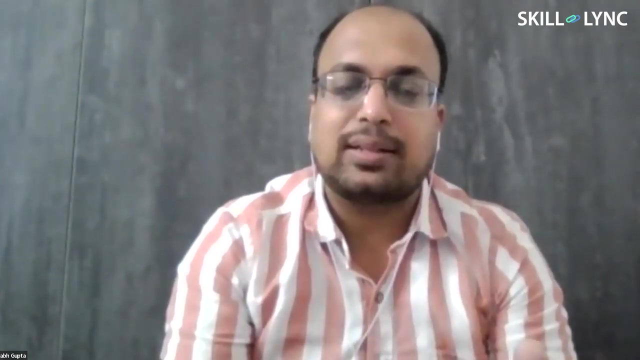 so you will be getting the entire case study to do the case study, you will be getting the all the assets and then you have to perform that thing in the primary after learning that module, so then you can demonstrate it to anyone. yeah, i have done this, and even before that i'll say that you will. 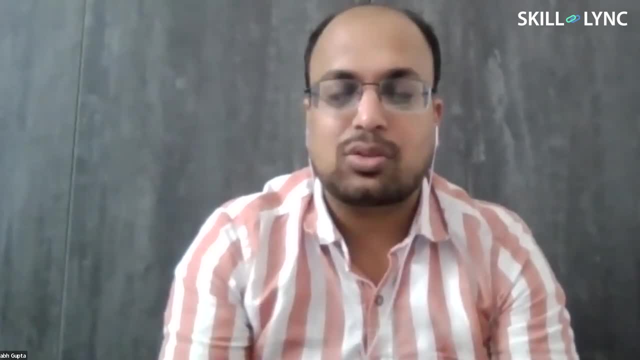 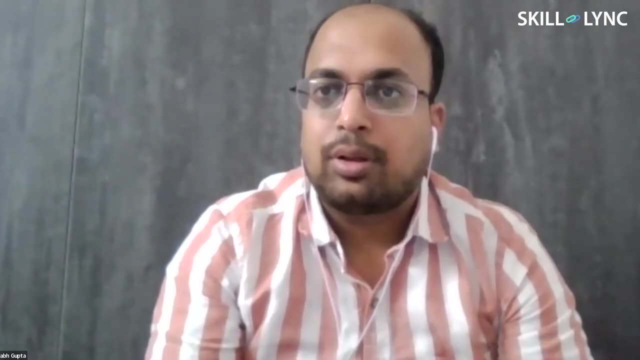 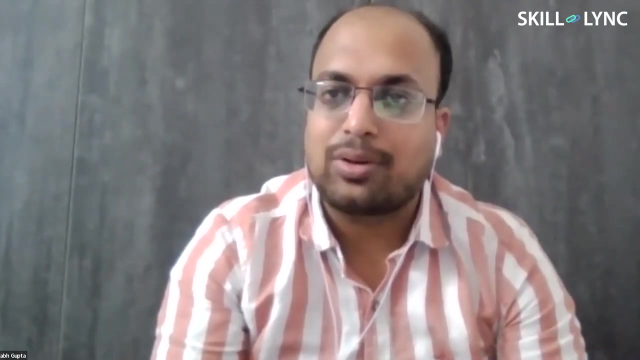 get a confidence level. yeah, okay, i can do this, so then you can demonstrate it to anyone. all right, many people say that civil engineer does that, doesn't have any career, so what do you think about it? and i can feel that because i have seen many people with no job, see your. 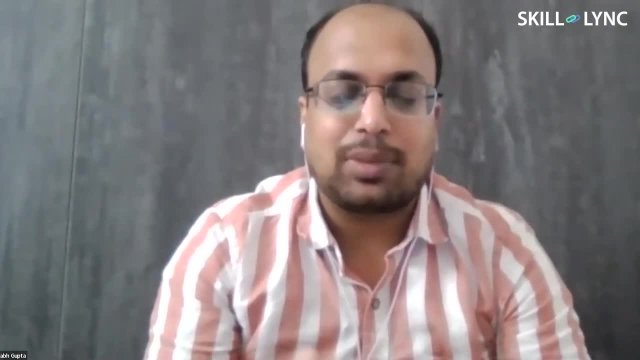 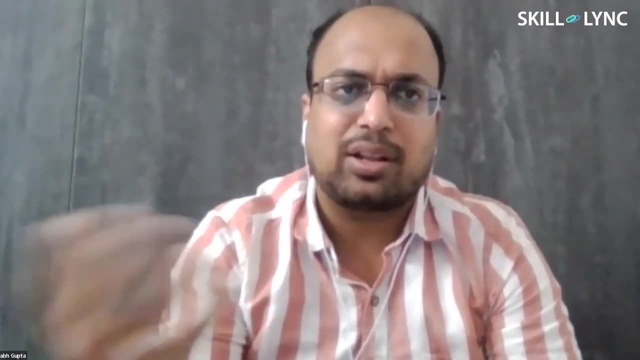 ultimate knowledge is the thing. okay, uh, i'll say simply: i i just told you so you just uh mentioned somewhere that you know uh national pipeline projects. so there are 8 000 projects that are happening in india. okay, you just mentioned that you know uh national pipeline projects. 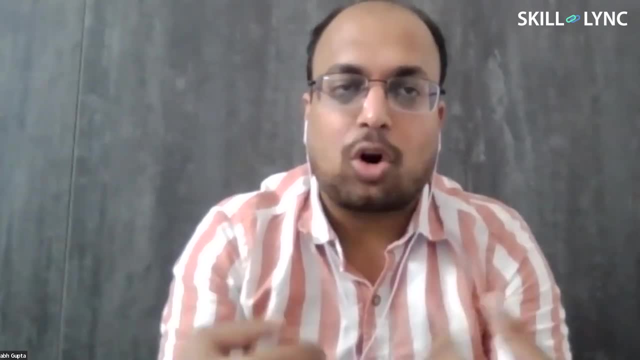 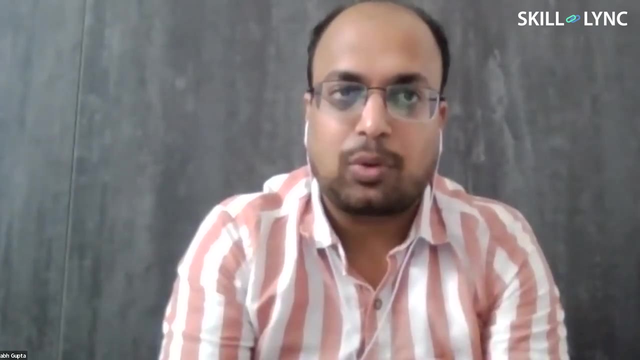 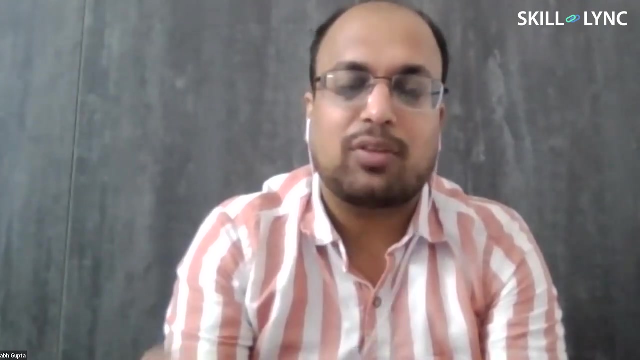 you know, whensoever. uh, you know, uh, companies talk to us so they say that there is a huge deficiency of the right talent. okay, the right talent is not available. so that is why people say that jobs are not available. a lot of jobs are available. you search or anything, but you know. 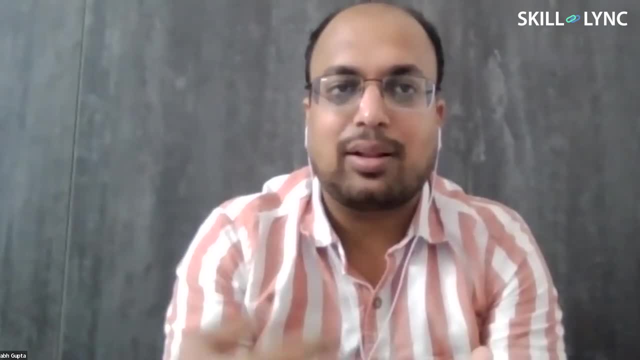 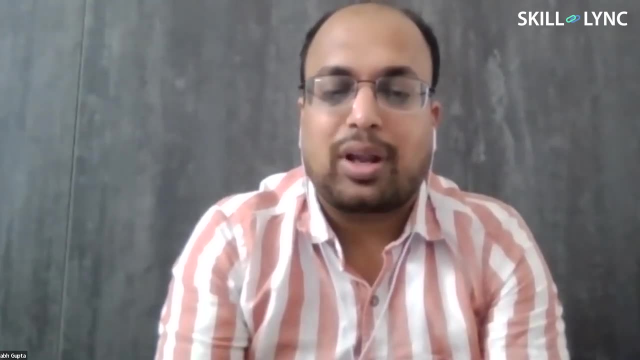 the people are not correct. uh, you know, learning the right thing. they are not cracking the interviews. why they are not cracking? because they do not know what the industry wants. so that is why it is important. uh, there are two aspects to see. you know you are on the other side, uh, but you 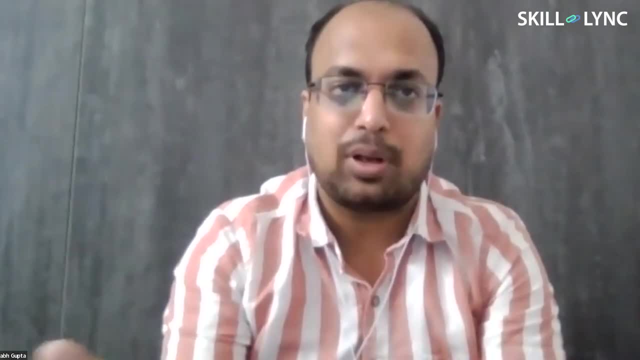 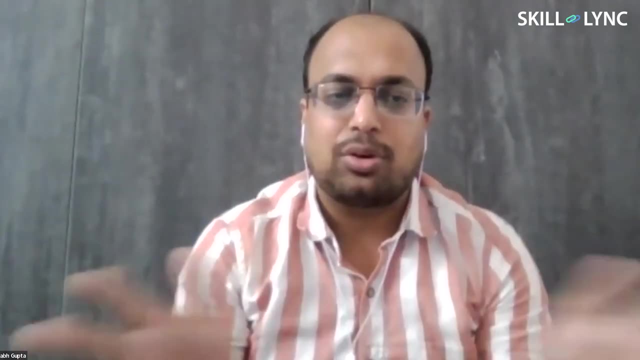 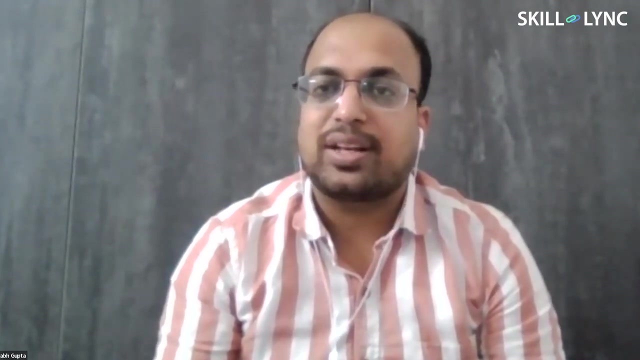 should put. you should put yourself into the shoes of the industry people. if i am taking the interview of a person, i'll be requiring him to know the industry things. so that is what you know. the gap is there in the education. i'm a site engineer to become a planning engineer. how my site engineer 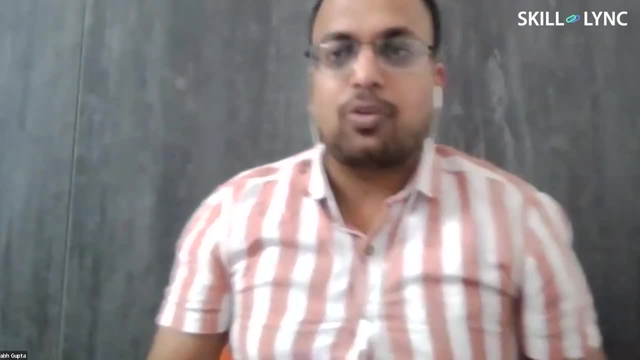 experience is helpful. yeah, it will be totally helpful for a site engineer, practically saying, because then the company will be able to do the job, and then the company will be able to do the job, and then the company will be able to do the job, and then the company will be able to do the job. 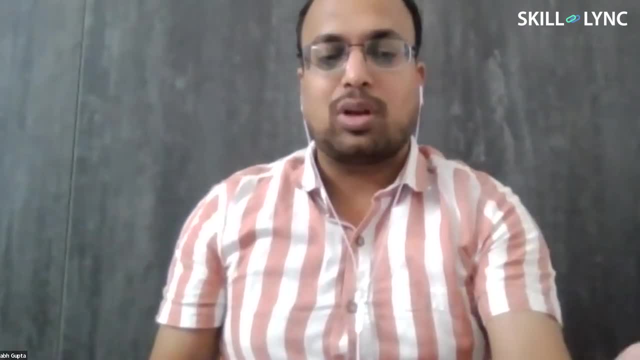 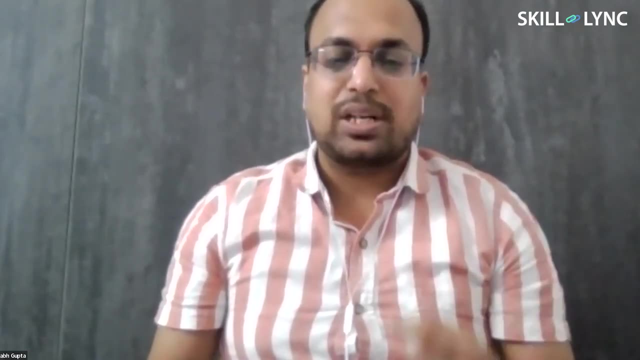 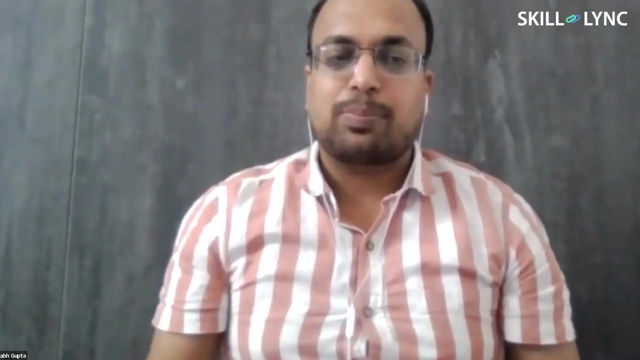 you have to be thinking that you have gained much exposure at the site level. now you have to learn the construction management techniques. you have to learn how to plan the project, then you have to learn how to prepare the cost budgeting, then you have to learn how to do the contract and subcontracting. and once you will be learning all these aspects, 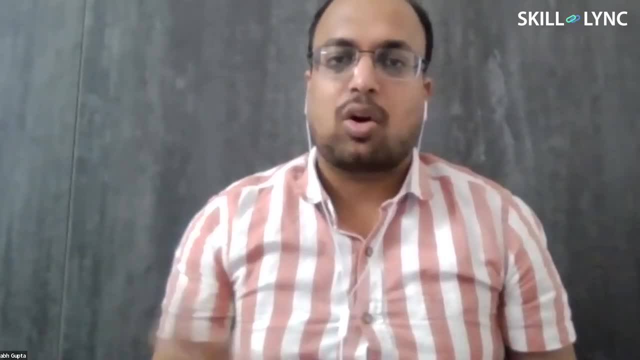 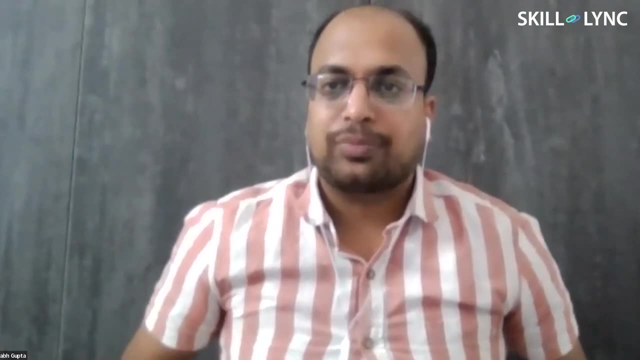 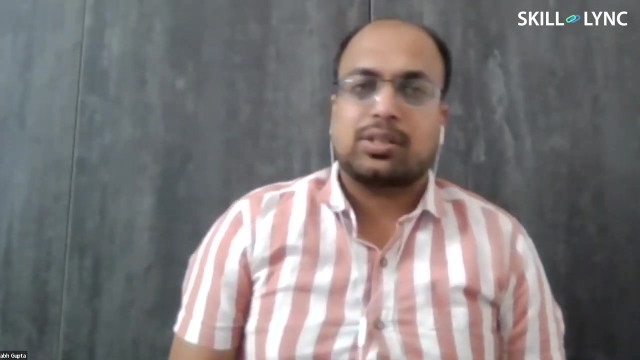 then the company will be taking you in any manner. you can see a lot of? n number of linkedin profiles. those were site engineers, they learned the construction management and then they move to the different Lee. IIT is that they are offering one crow rupees of package or threecro? rs of package, but that's not. 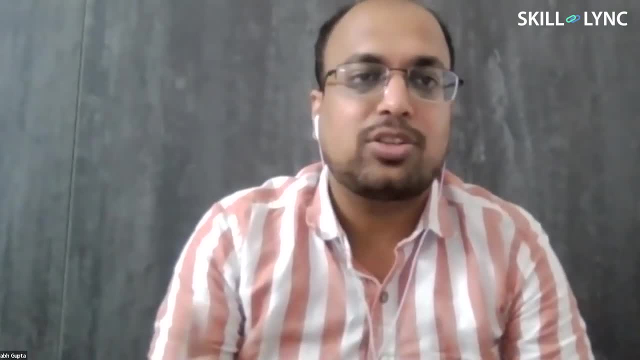 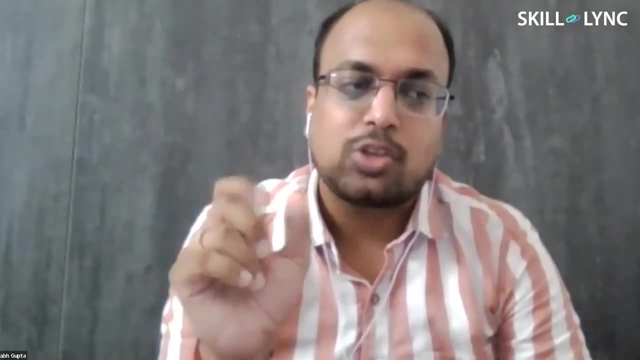 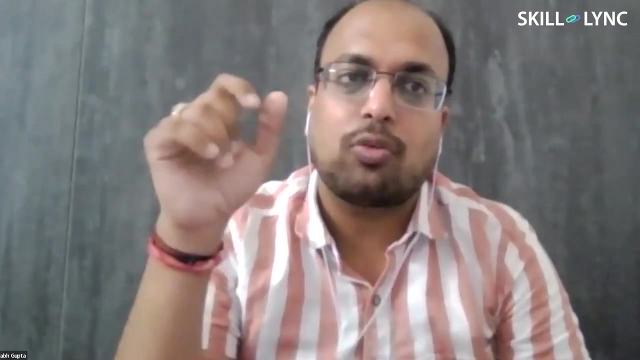 the package. that's a you know hype. what's the average package? okay, so even an average package of iit is eight lakh rupees. so that means people are getting eight lakh rupees but out of 4500 iitns. how many are getting one crowd rupees out of 5 000 iitns. so this is good for our entire company. because you don't have to do the whole thing. you don't have to just go out and do all the work. you have to do it for yourself. you don't have to do everything. a lot of people are doing this, but i tree. you have to do your job in your company. you have to do everything, so everyone who is also involved in it. 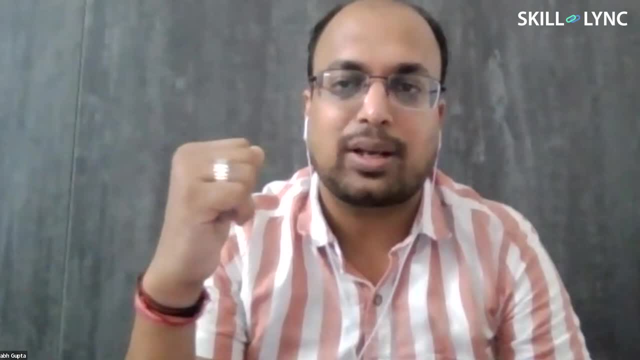 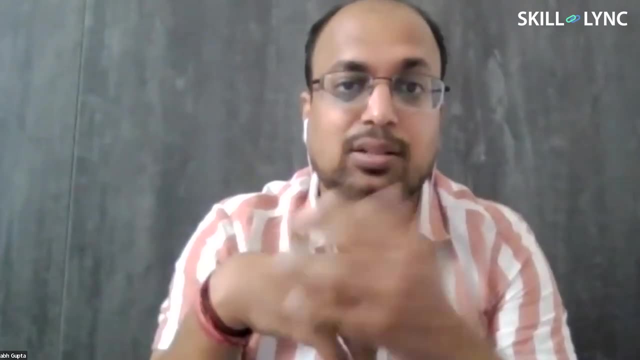 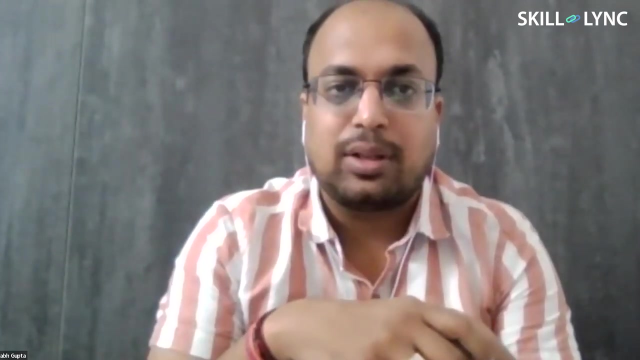 package. but everybody is saying that yeah, they are getting one product package. so even in what requirement i am getting? we are getting six lakh rupee for freshers. that is also the requirement available, all right, so it depends how much knowledge and skill you do have. then, with the same level of company you will be going. so minimum it starts with the 2.5 lpa and it ranges from 6 lpa. so now you have to see that, how much knowledge you do have, which company we can target. so all these things will be happening. 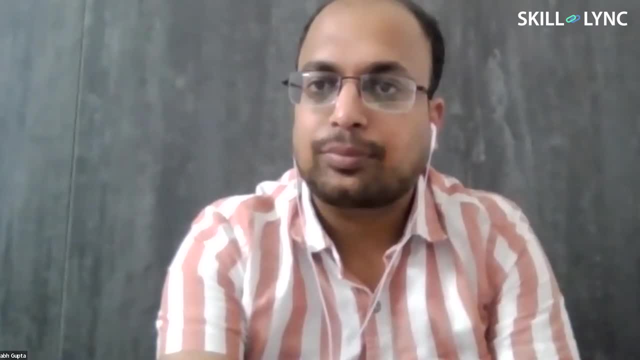 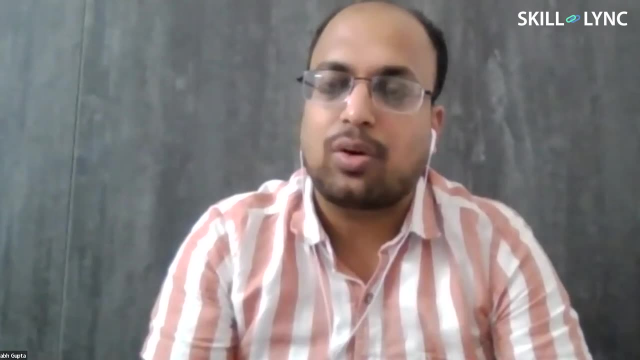 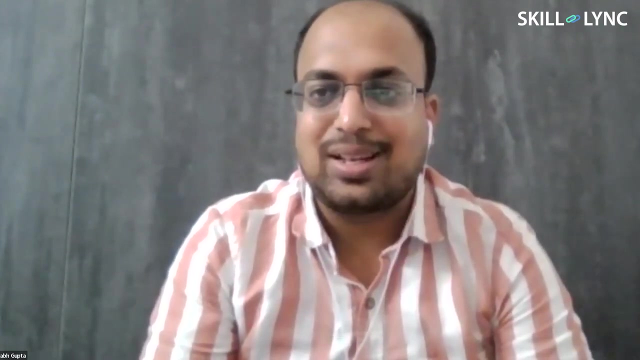 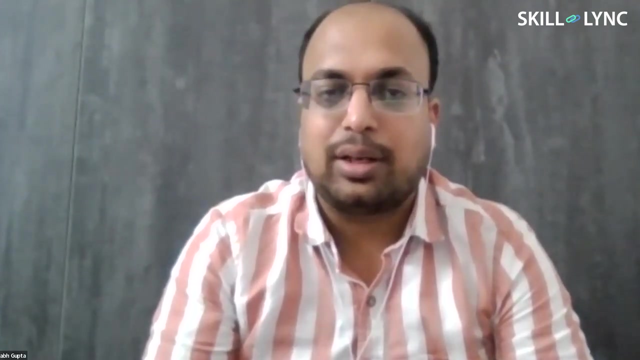 uh see, it's not like that. the everybody is asking for the fresh, uh experienced one. only uh. a lot of people are working as a freshers. i started my career as a fresher- only so uh is power bi is using in construction field. yeah, it's, it's the new thing and it will be coming. uh, power bi and ms excel- they both will. 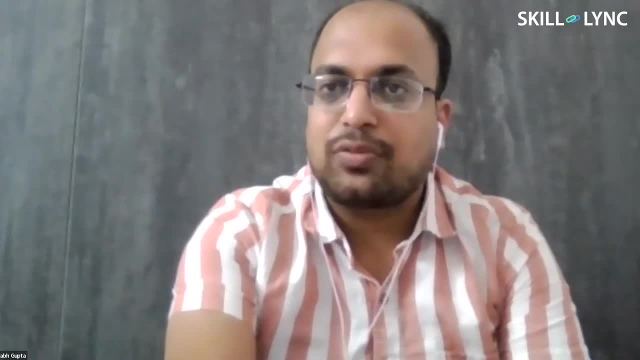 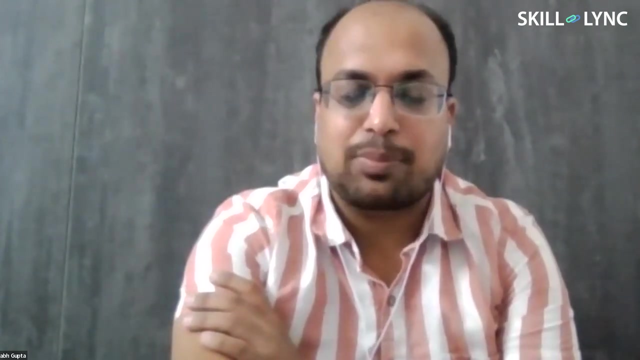 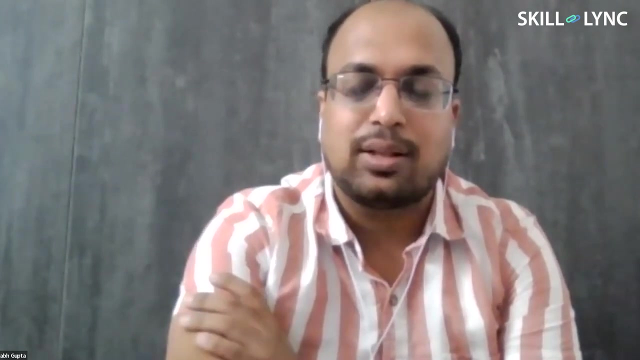 be utilized in the uh construction field. see if somebody has asked that what other softwares are required for the construction planning. see if you have learned primary, where all the things are there, that's the most powerful software. then you understood the psychology and terminology. then it doesn't require that you have to go for any other software. uh, it will take just three to 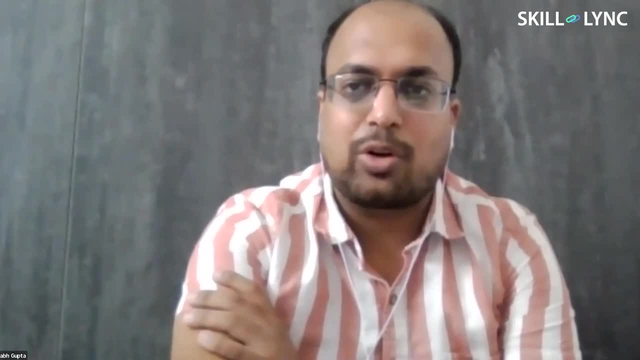 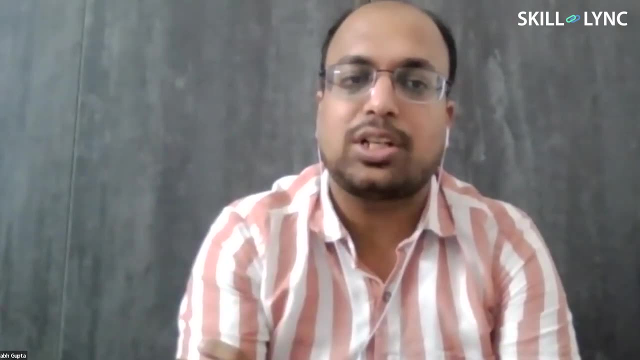 five days because you have understood all the concepts and everything. so don't waste you on your time. you know, on these kind of things you should. you should see that how i can demonstrate that knowledge. you can demonstrate that knowledge by completing some kind of projects, all right. 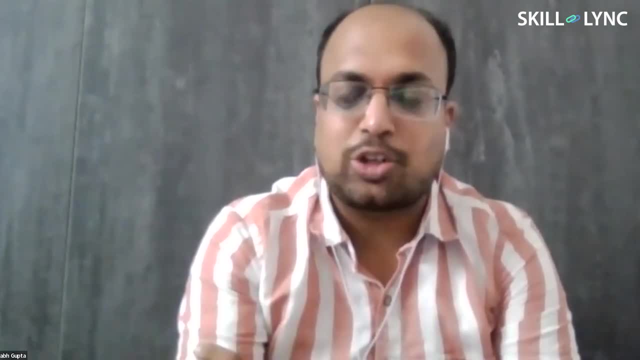 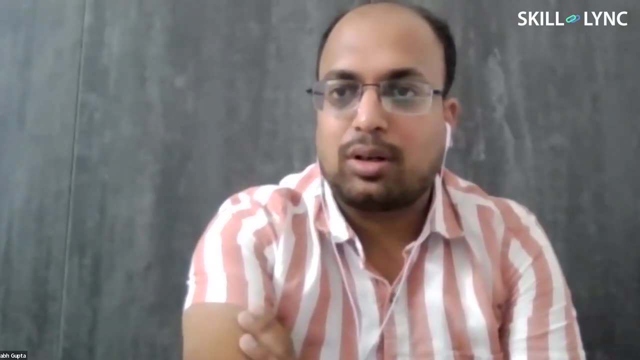 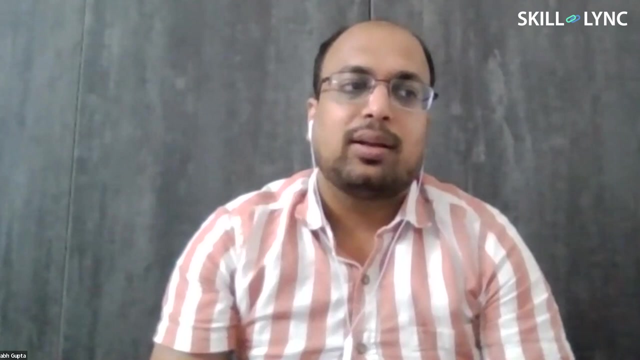 from where i can get those sort of projects and challenges. that should be the task for you. yeah, hope i have covered all the questions. can you please can you repeat critical path and practical example? okay, let's say that, uh, in your project that there are 1000 activities. 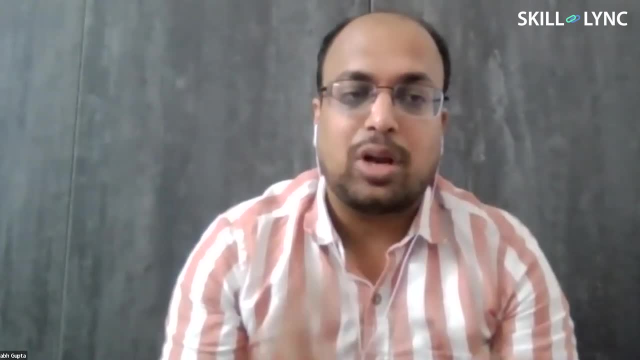 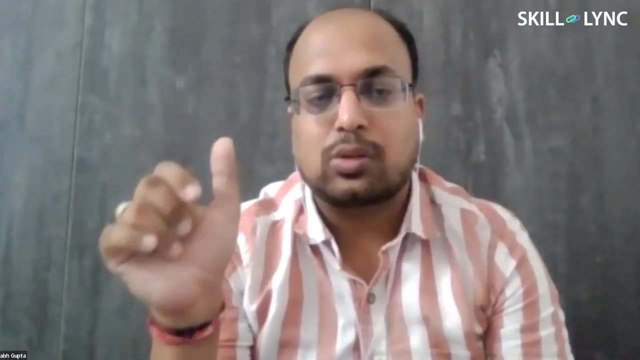 one 1000 number of activities. so it will, and you have provided the relationship of that 1000 activities. but it will not be like that that out of all these 1000 activities will be coming on the critical path. let's say, out of those 1000 activities, 150 activities will be coming on the. 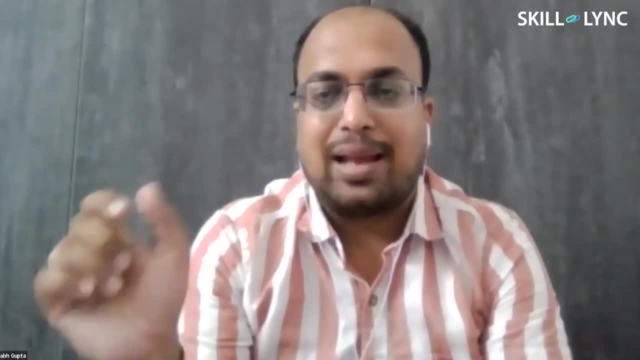 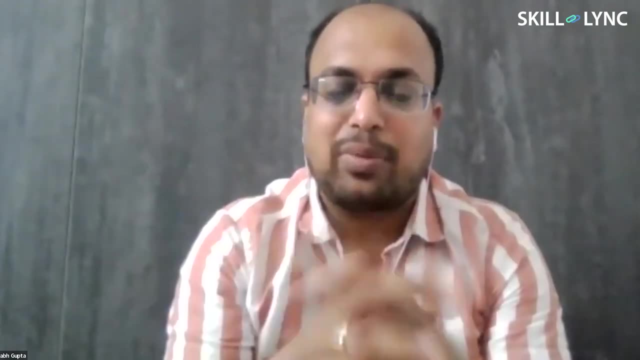 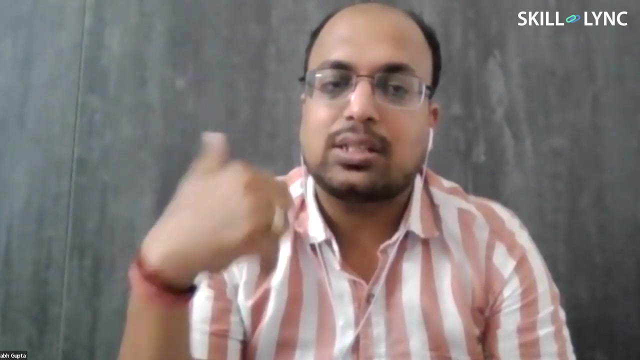 critical path and balance. uh, 850 activities are there which can be delayed, so that will be auto generated in the primary software. okay, i'll not be going into theoretical one. so that is why these 150 activities the planning engineer will be paying much attention. it's not like that on the 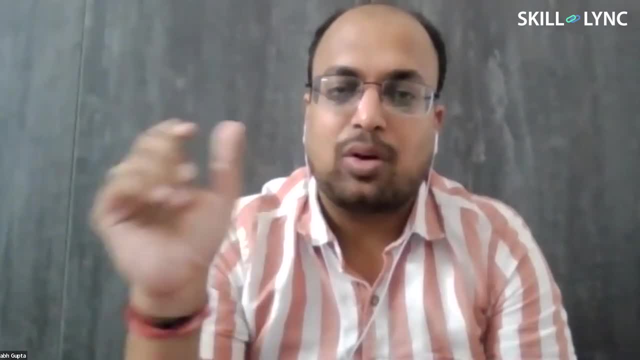 other activities. they are not paying attention, but it will be a more attention will be paid on this 150 activities. if this activity will be delayed, their project will be delayed, okay. so that's why i have provided the relationship of the 150 activities that are coming on the 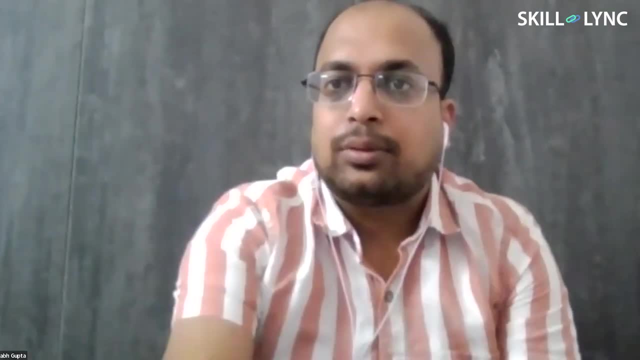 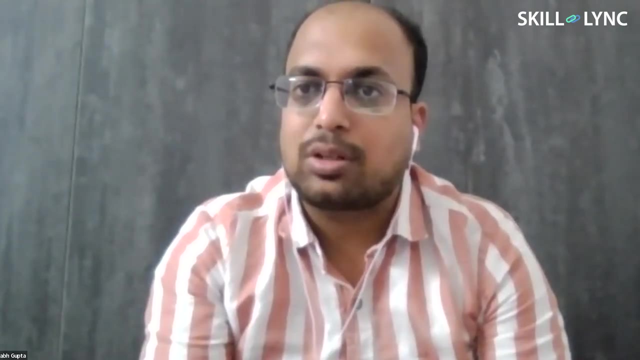 project. so that's why i have provided the relationship of the 150 activities that are coming on the. okay, i've got one question. i have worked as a design engineer for one year, but for growth i've joined as a project coordinator in bangalore. please guide me. what i learned to? uh, yeah, so the? 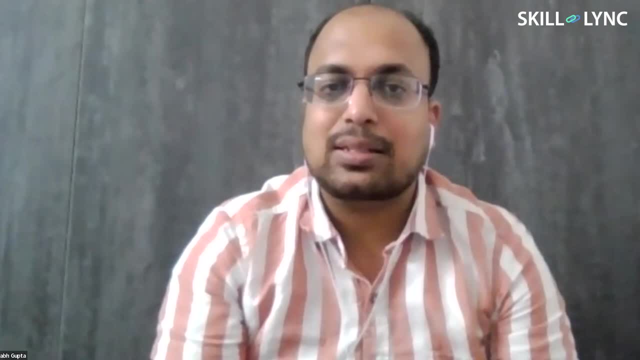 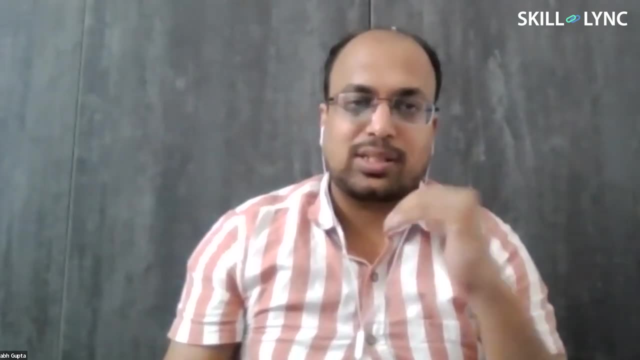 simple thing is you have to learn the construction project management. so the thing is, uh, i'll tell you very simple example. so, uh, first thing is the you know either a fresher or a site engineer, anything. the next target is to learn construction project management. after learning construction, 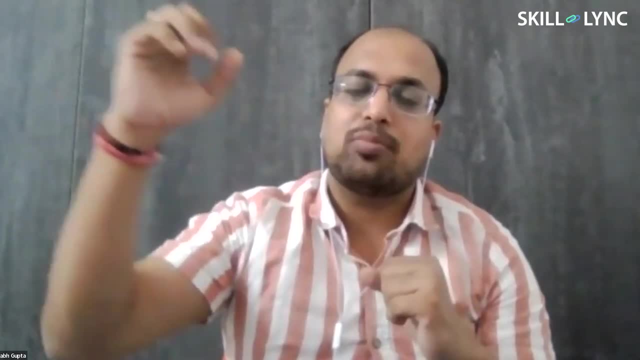 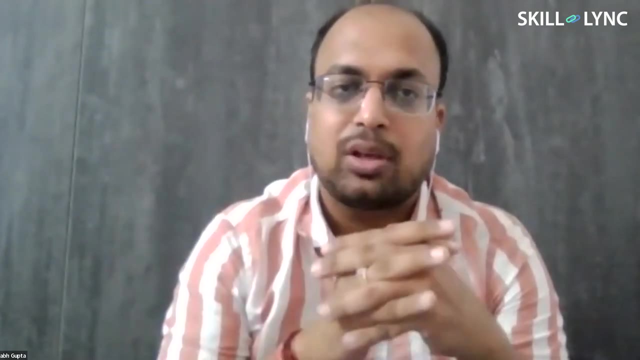 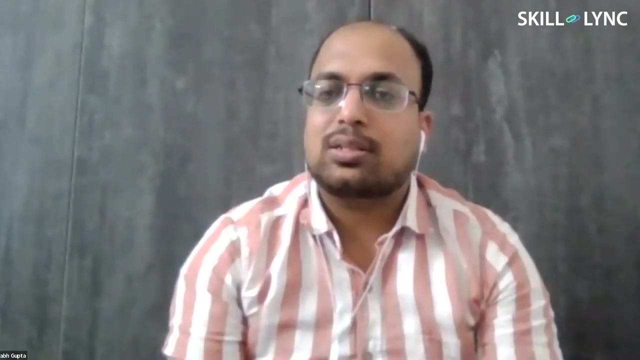 project management after learning construction project management. after learning construction project management and working in that particular role, then you will become the project manager or you will be working as a project management controlling lead in the offices. so that that's the goal. uh, you know. yeah, don't go girls, it's for girls. you know so many friends of mine. they are working. 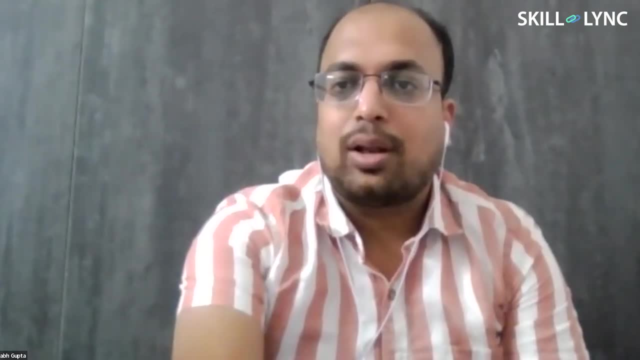 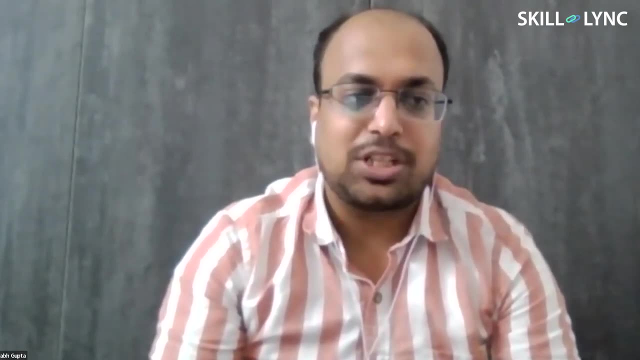 in construction project management. so, uh, you can learn construction project management. you know, i'll give you so many example. one friend of mine i was talking, she's, you know, she's a construction project manager. she's a construction project manager, she's a working in contracts department. she's now got another job as a contracts head. another friend of 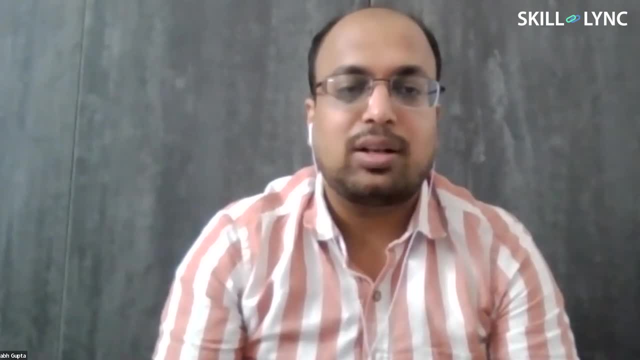 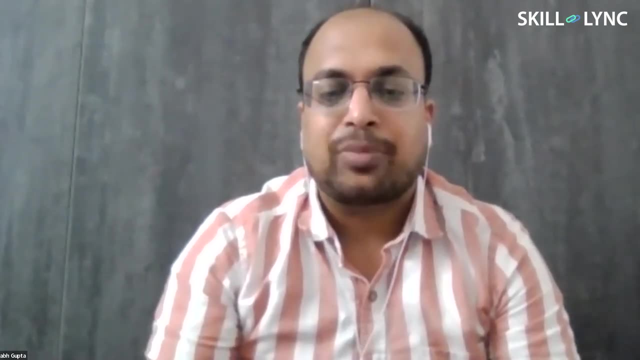 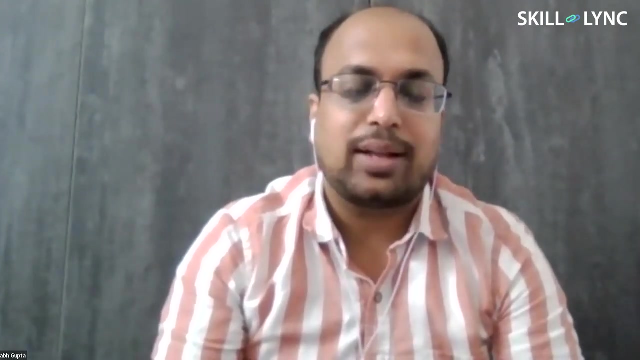 mine. she is working in the tendering department. so if a girl is learning the construction project management, definitely uh 99.9 percent chances are there they'll be absorbed as a uh office job. so right now for skill link ramki infrastructure. it's a very good company of the hyderabad based. 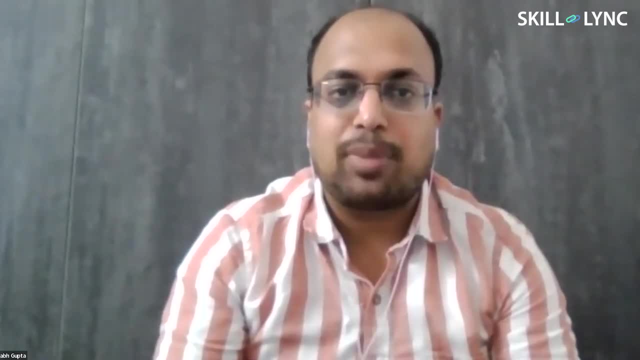 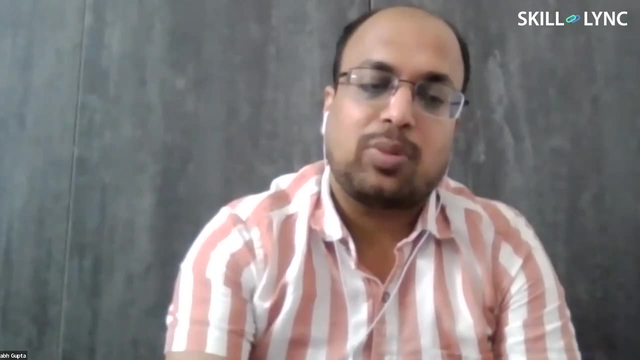 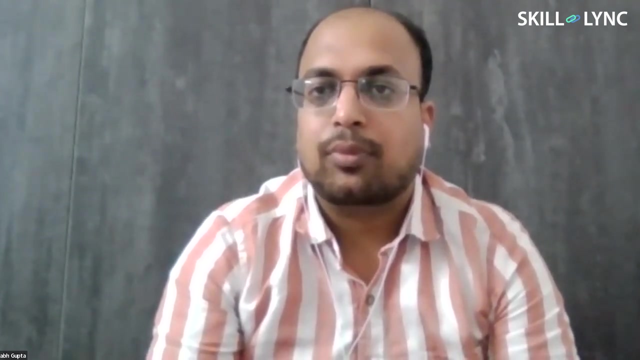 ramki infrastructure. so they appointed 20 people from the skill link out of uh that those- so uh whosoever girls- were there. they have been given the job at the head office. see uh choosing you know construction management, see, it depends upon your interest. so you know once. 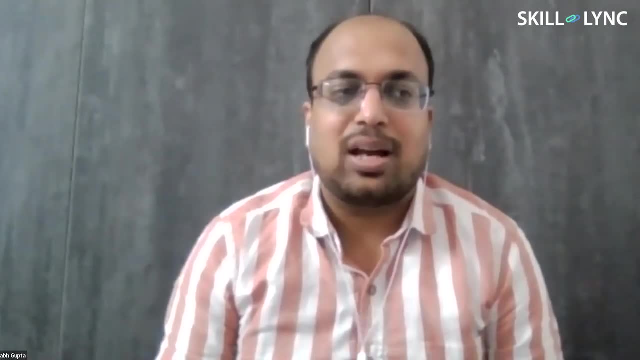 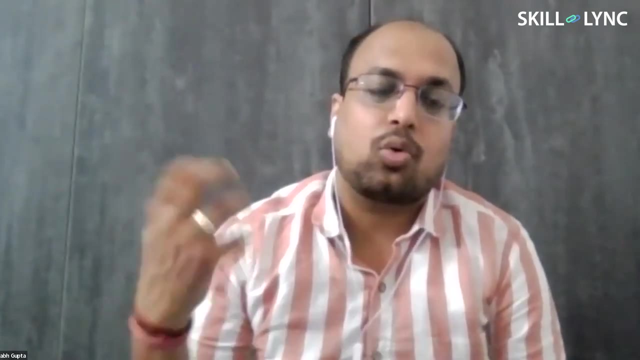 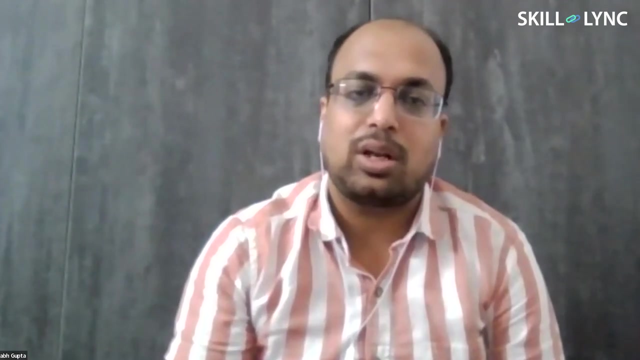 i was in the college. uh, my simple interest was like that: yeah, i want to opt the construction management because you know, uh, there, you know, every big picture is there, how to complete the project, how to handle this kind, this sort of money. uh, then ultimate goal is to become this c? cx of some company after 20, 25 years. so to become that. 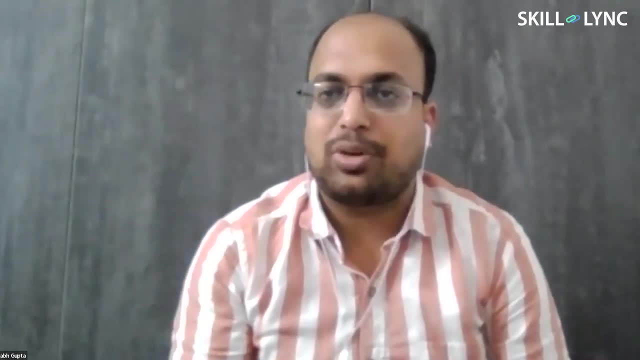 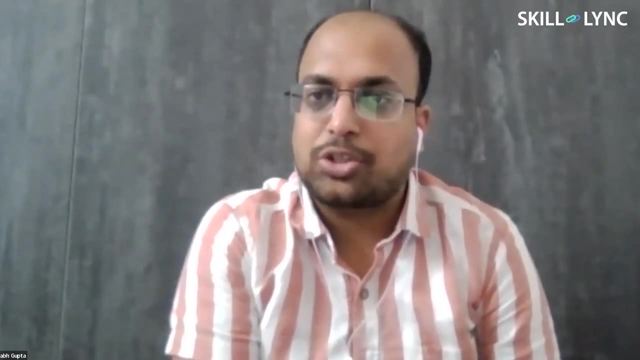 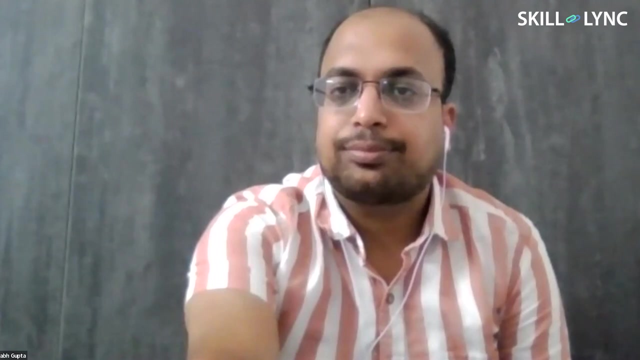 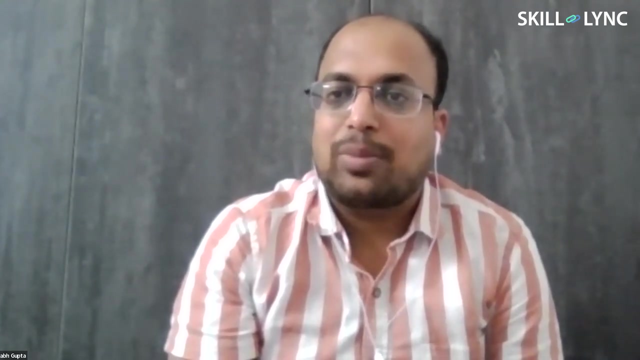 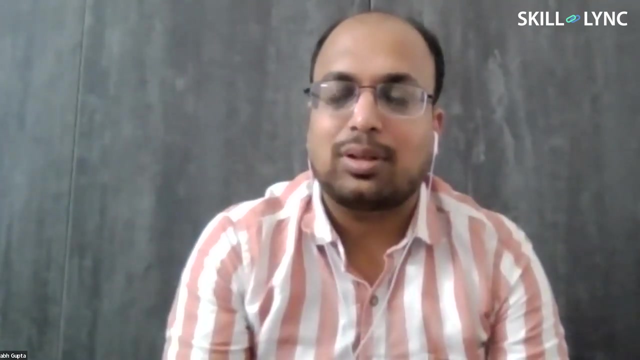 uh, some someone has to learn construction management, so it depends upon interest. yeah, but a lot of job opportunities are available. 80 people work in construction project management, that's that's for sure. uh see project management, or construction project management. see ultimately, uh in if project management. uh, so it's related to the construction industry, so that is. 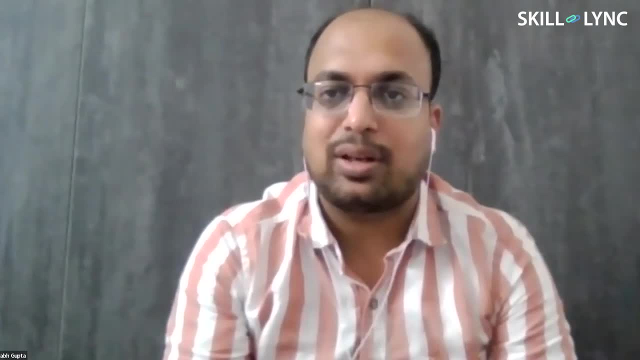 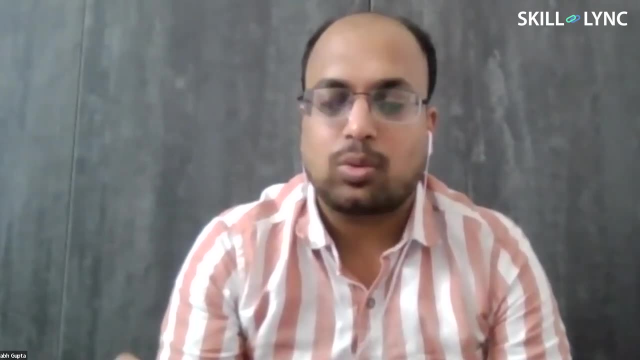 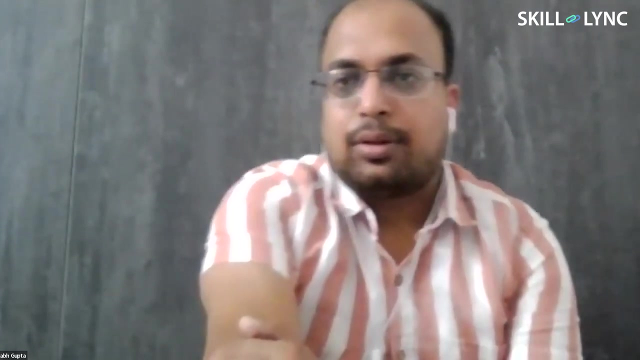 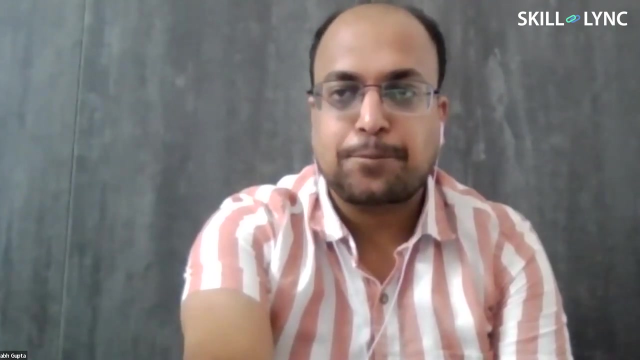 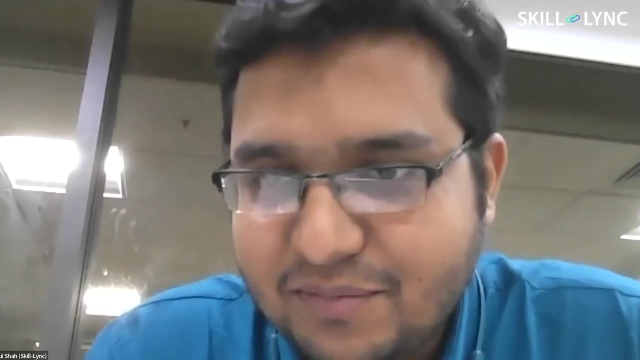 why it is called construction project management. there is no other difference in it. for stat pro software, there are jobs for design roles. yeah, hi, mehul, i think, uh, we have covered all the technical aspect. all right, uh, great, uh, uh. sorrow, but i have a couple of questions in my inbox. i'll just 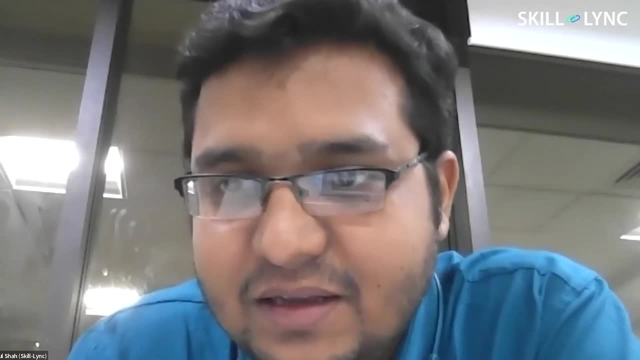 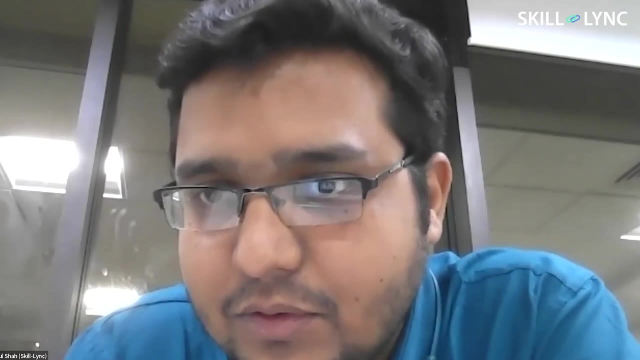 you know uh ask those questions so that uh folks can get the- uh you know- answers to their question. but i think a couple of questions uh they already asked you, uh i might be, you know uh repeating those. so if you have answered just a couple of questions, i'll just ask you a couple of questions. 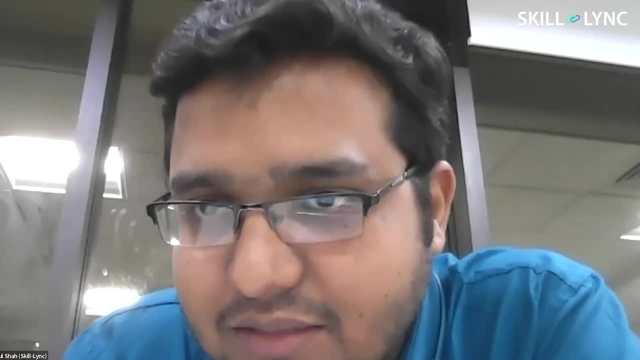 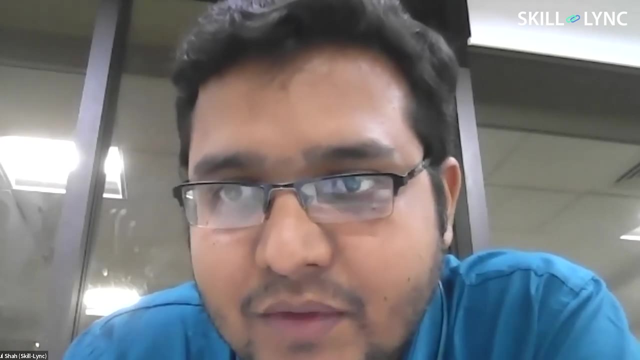 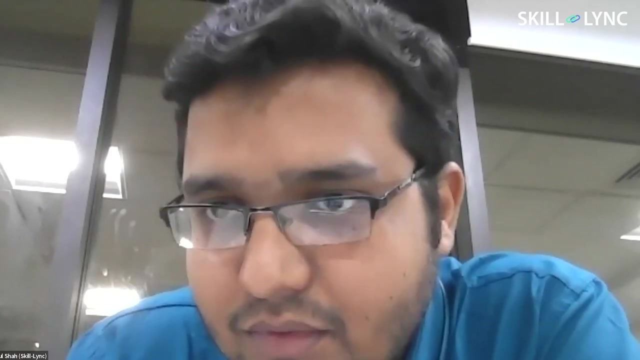 let me know. so the one question asked by am i is like: how can i find a job after construction management? construction project management: i have done an architecture degree and also i am pursuing the construction project management from mit acd. uh, i don't know what is this mit sd? you want it. 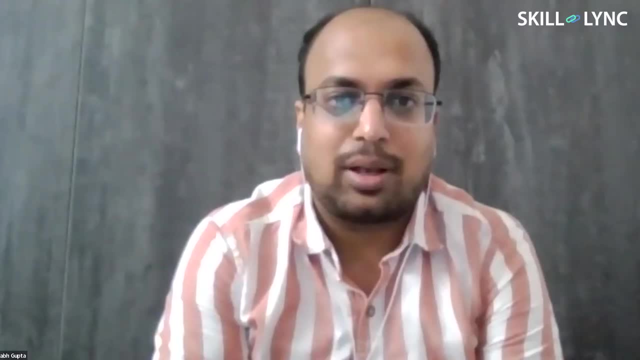 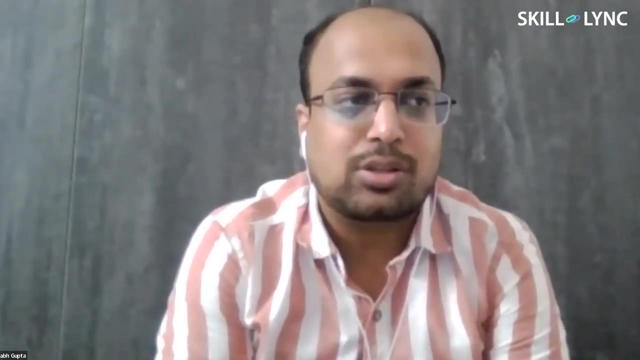 might be a college. yeah, it might be some college. uh, i know my statute institute of technology, which is world's number one college, uh. so, but you know, if you have done architecture, so uh, i think it will be very difficult for you, but you can go for the project. 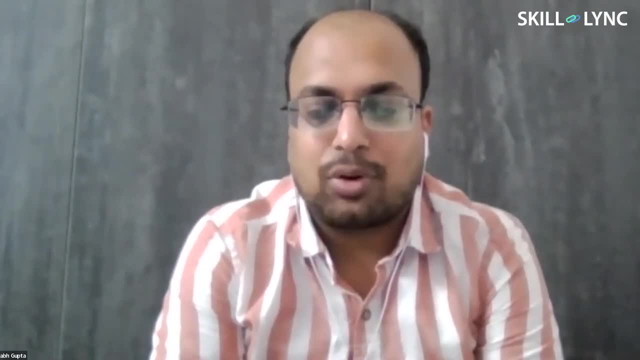 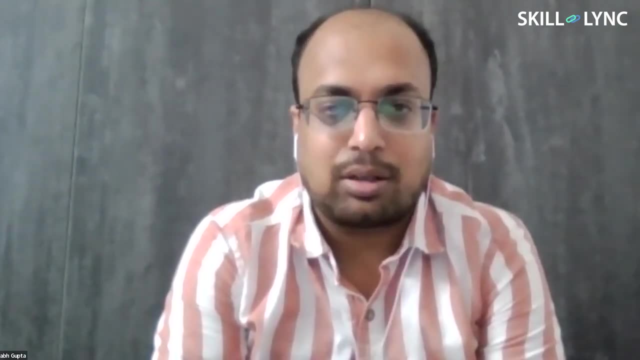 coordination role, but then again, you have to evaluate that. you know why, why you are not going for your architectural role. uh, i think, i think, uh, she, she can have a one-on-one session or demo session with us, because we will be getting more clarity about her previous role and future. 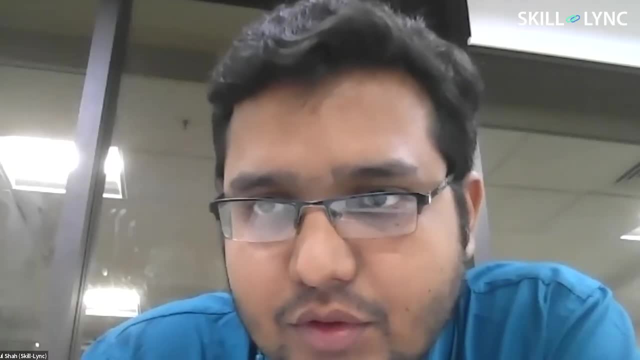 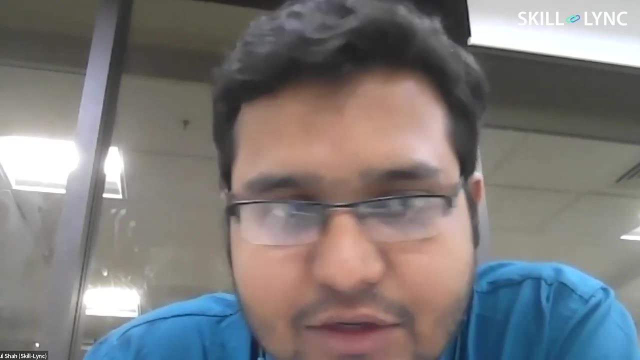 aspirations make sense. so i hope you got the uh required answer. i know it was uh, not to the point, but uh, as mentioned by saurabh, you can basically you know or get in touch with us and we'll help you out, because we require more details. 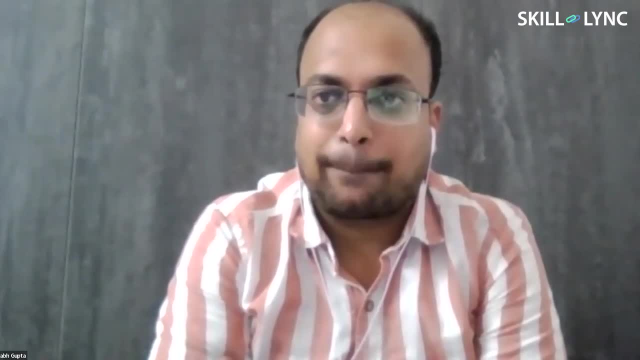 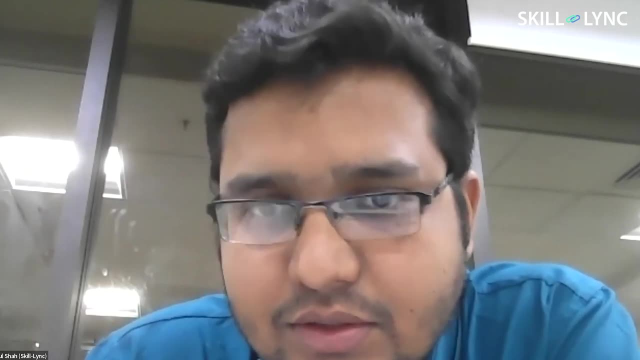 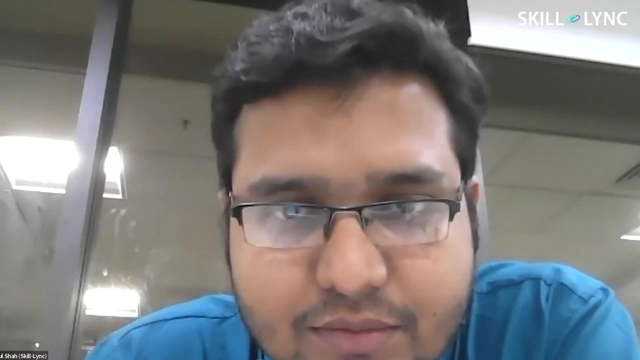 to understand. you know what happened exactly. so another question asked by anushri is like: what about pget structural? is there a chance of becoming a planning engineer? sorry, pget structural, uh, is there a chance of becoming a planning engineer? yeah, it's okay, because you have done the b-tech and once you will be doing some course and you do not. 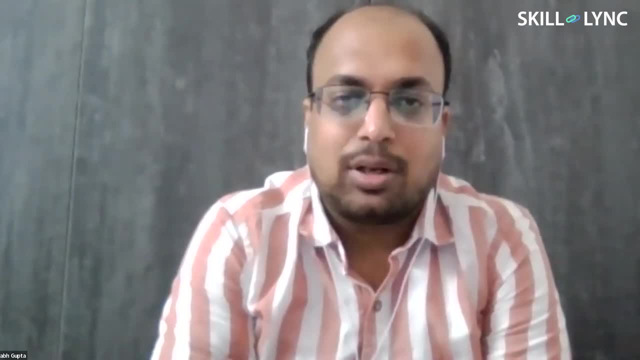 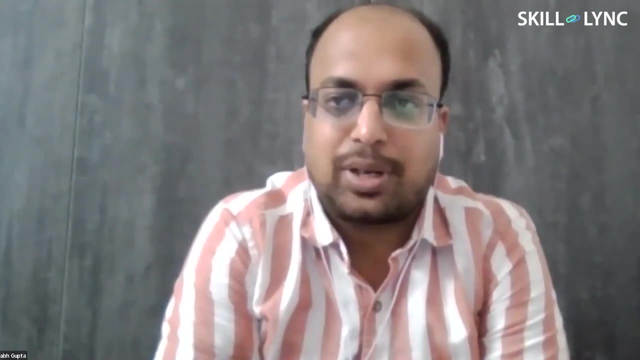 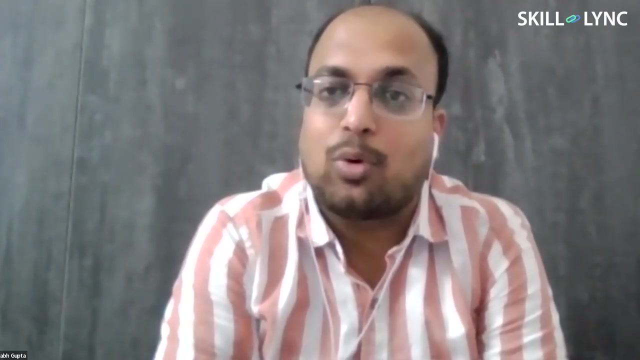 have any prior experience in uh- even design, i'm assuming- uh so you can go for this course and uh take up your uh role into uh this construction planning and management. so i got a very uh difficult question here, as you have experience in mncs: which sector in civil gets paid more design? 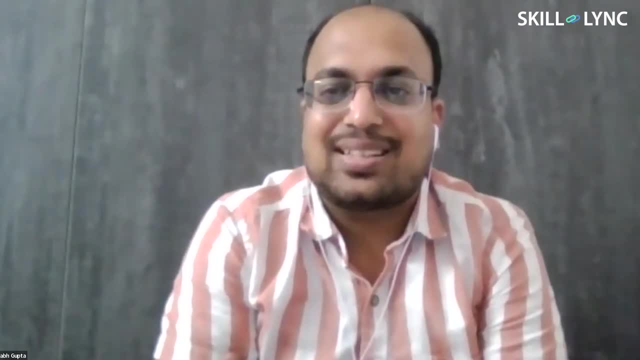 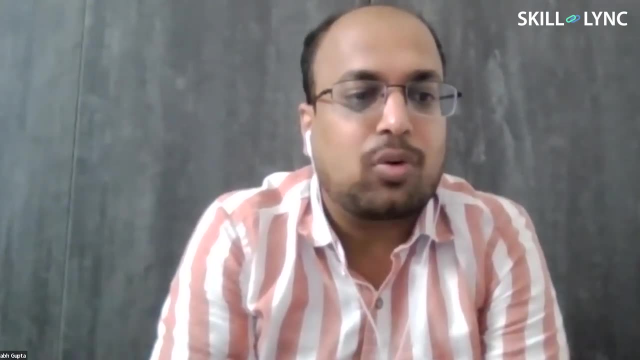 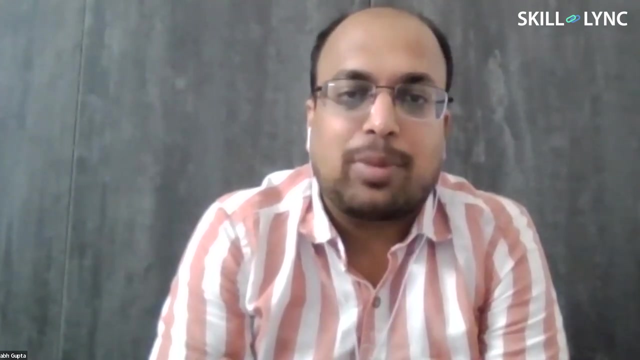 or management or any other. so so the thing is very simple: if 100 civil engineers are there, 80 people are there for the construction management and ultimately- you can google it today. uh, why i love construction management? because you know, if i was an lnt, so the chairman of the lnt am nayak, or the 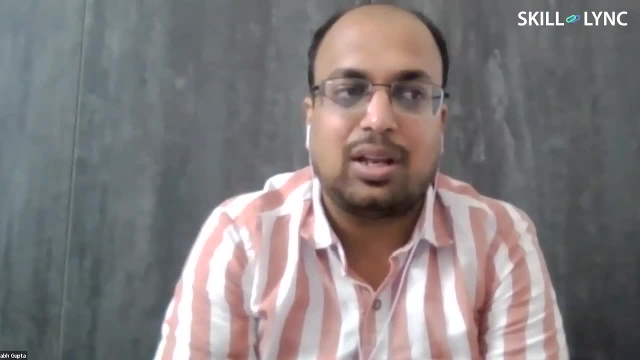 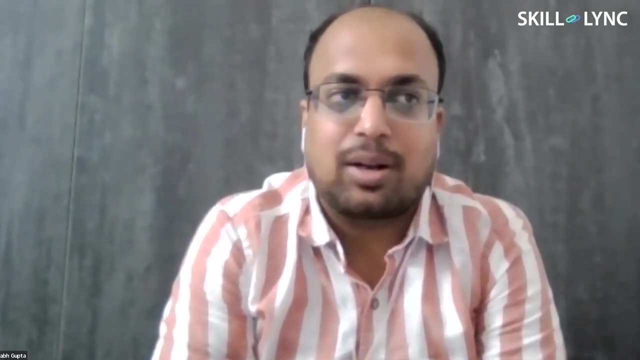 current chairman sns. they started their career as a get. they were working for construction management. so any any ceo, you take it from any construction company. so they started and they were doing the role for construction management. so that was the inspiration for me when i was in college. 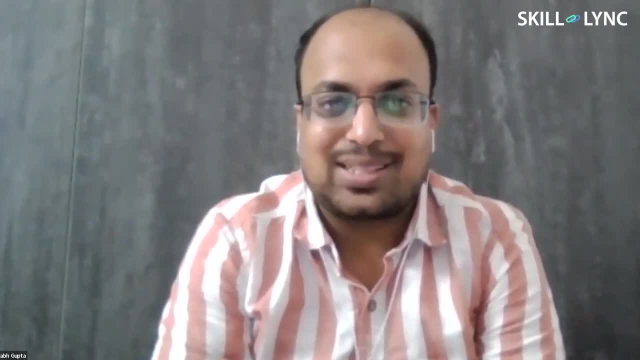 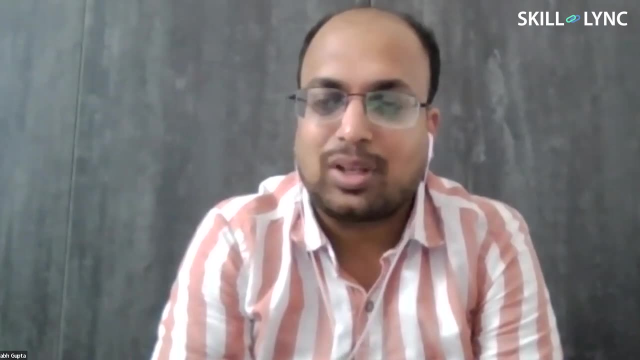 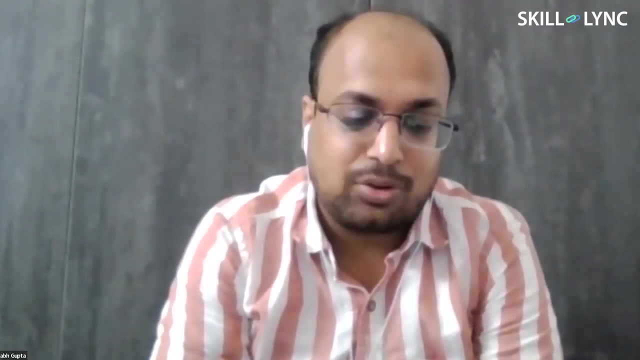 that one day, maybe after 25, 30, 40 years, i'll become the ceo or something like that, cxo. so that's the thing for me. otherwise it depends upon interest. yeah, they are paid well and you know, uh, you know it's. it's very motivational to say that you know ceos of like. i'll be saying that. the biggest construction company in india, ceo, is getting 100 crore rupee, more than 100 crore rupee per year, so the salary is 22 crore rupee per year and they are getting stocks of 100 crore rupee per year. uh, so that's the salary. that's the ultimate thing. 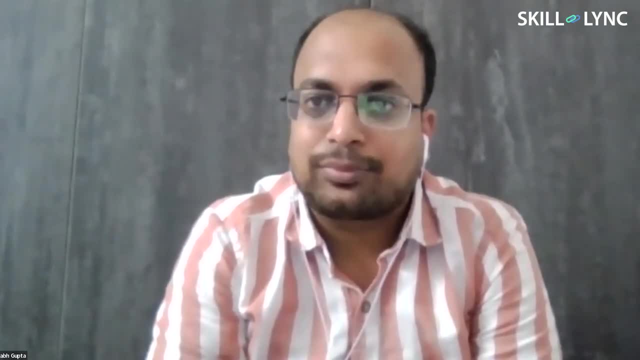 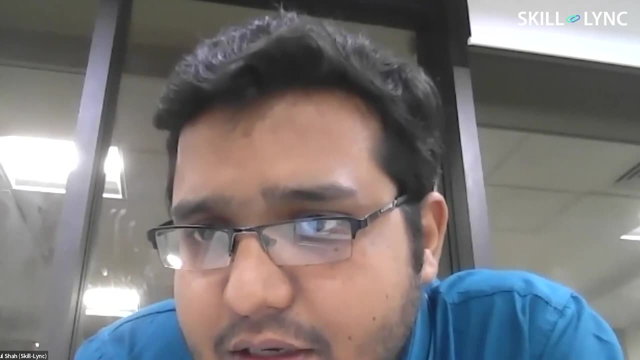 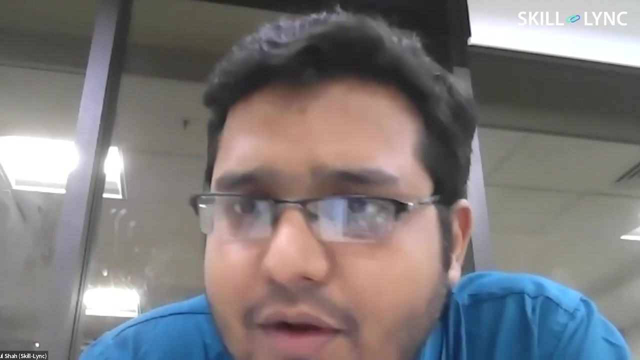 maybe you can get motivated from that great. uh, another question which you know: uh, we are basically having like one or two question. uh, like, currently i'm working as a site engineer in normal company. how can i switch to mnc? uh, if you have answered, you can skip. yeah, it's simple. learn the construction project management first. 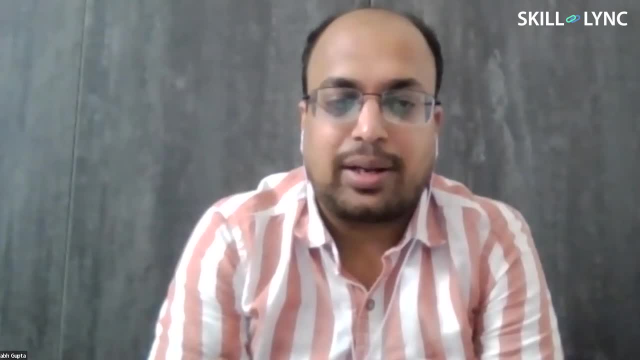 and uh, then uh, you will be getting the carrier guidance by, like, skilling is providing the program, so you'll be getting the carrier guidance. uh, people are working like in shoba: builder rohan, builder ramki. people have moved to lnt construction, something like that. 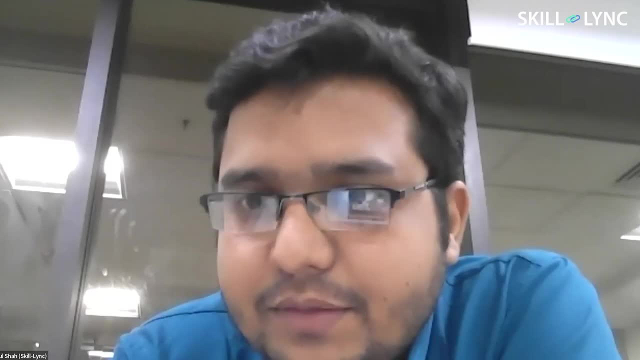 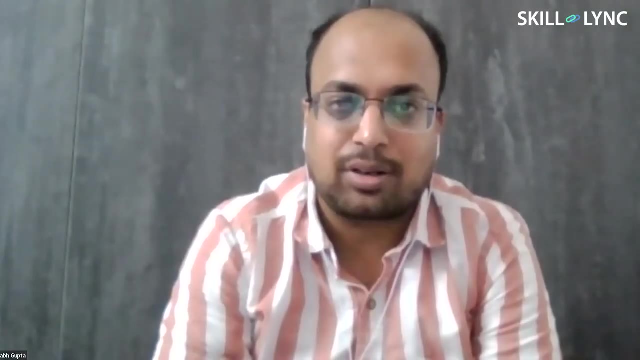 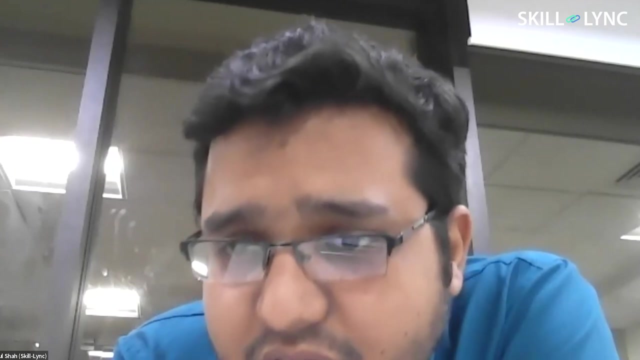 so, uh, how to start a career in construction management. i have completed my integrated mtech in 2020. now integrate uh mtech in what uh subject? uh, what? in which subject you have done, yeah, if you are interested in uh uh. uh, i think, shushri ananya, if you can, basically, uh, you know help. 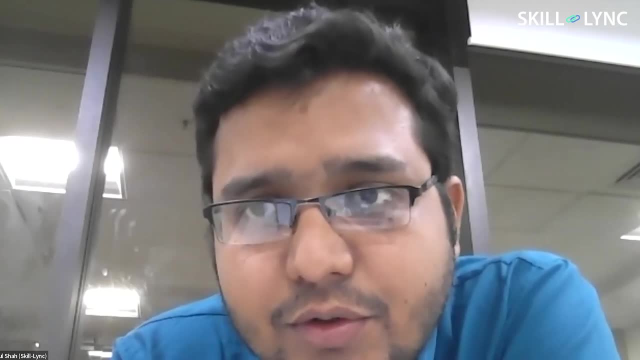 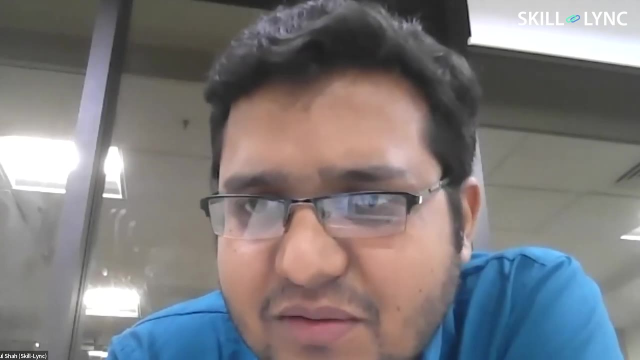 us out with that. we will be answering your question. uh. pg 18 lnt. is it good pg? ask banushri, pg et i don't know what pg et it is. if you can, what is pg et, by the way, anushri, if you can? basically, i think this: 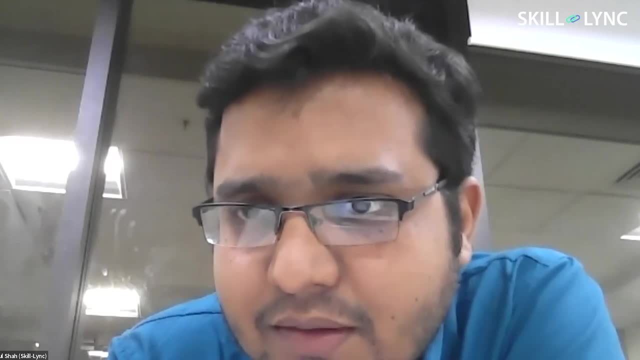 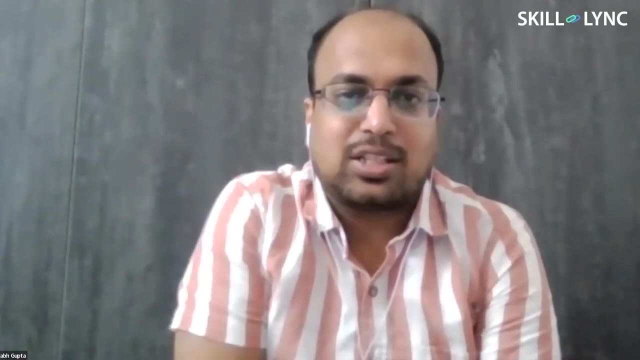 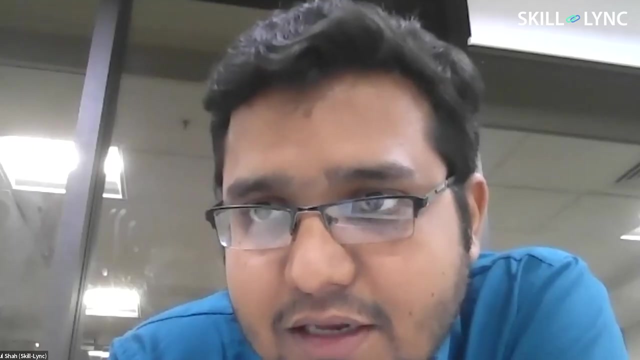 is the second time you're using this word- pg 18 lnt, so if you can help us out with that, i think it's post graduate engineer trainee, so one is geet, and then it is post graduate engineer trainee, so she's working somewhere or i don't know. i don't know. she's asking. 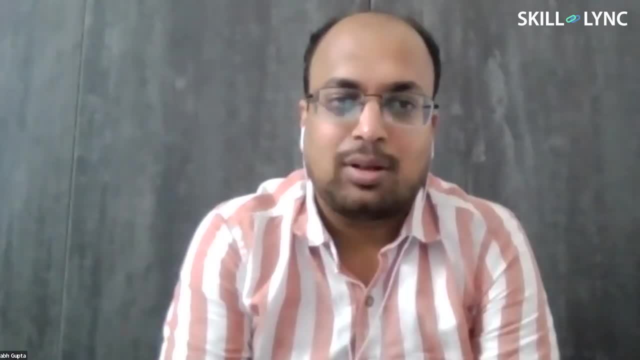 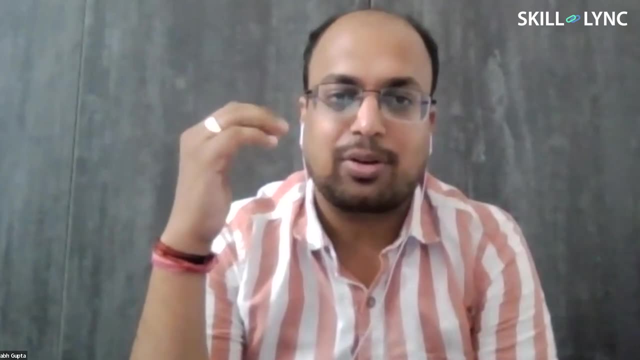 in lnt pg c is good or not? yeah, it's good, only so, uh see, ultimate thing is: you know you should make your career choice is very simple, that you know. i want to see my 30 years like this and what's my next goal. so if you cannot make 30 years, make five or ten years. 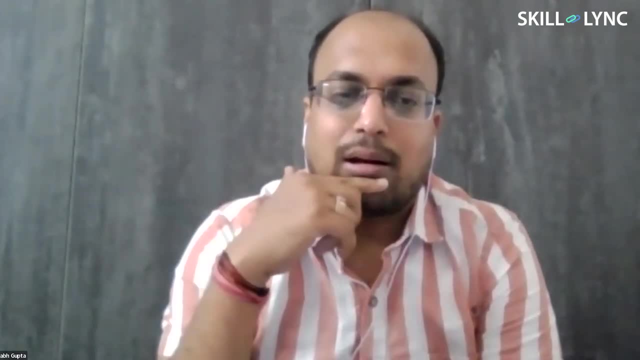 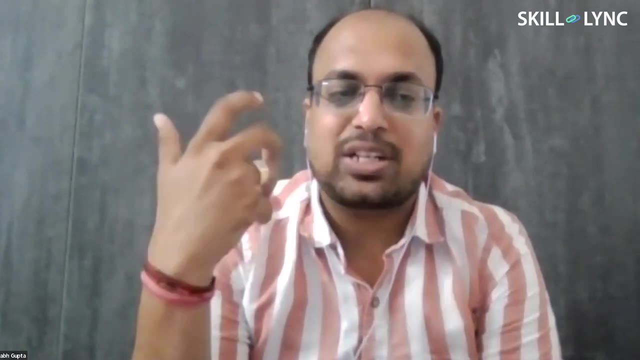 yes. so i'm putting almost five years first. so it's hard to um see if one year is not enough target, okay. so then, uh, i i do need a- you know- big construction company. that is required. that's my first goal. second thing, uh, what's my specialty? so then i have to learn in first, initial five years. 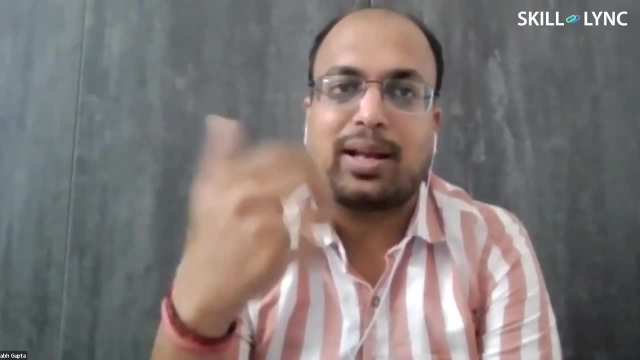 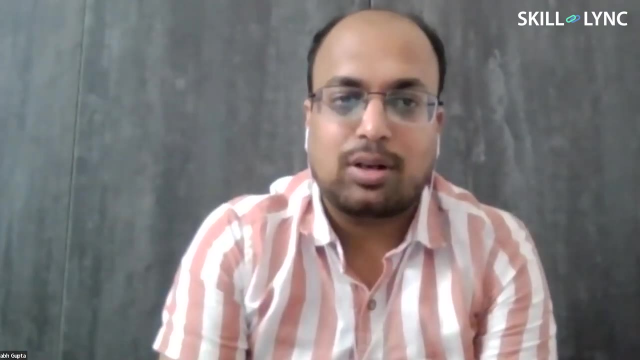 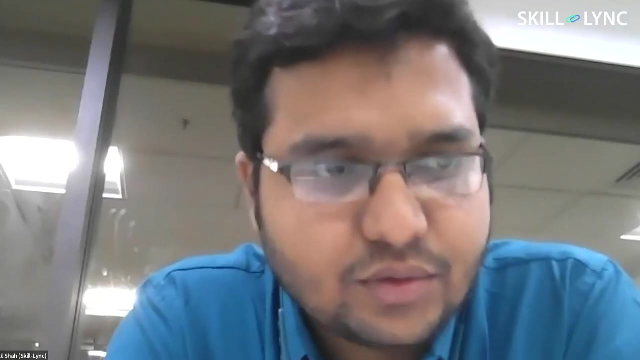 and i have. i should be knowing about these things, maybe like construction project management, so that i can advance my career in from 5 to 15 years. so like what you have to decide. so, um, the person who did mtech in structural engineering, so he did in structural engineering, so he is asking how to. 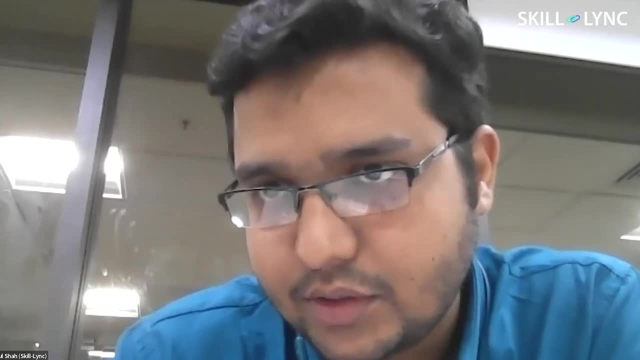 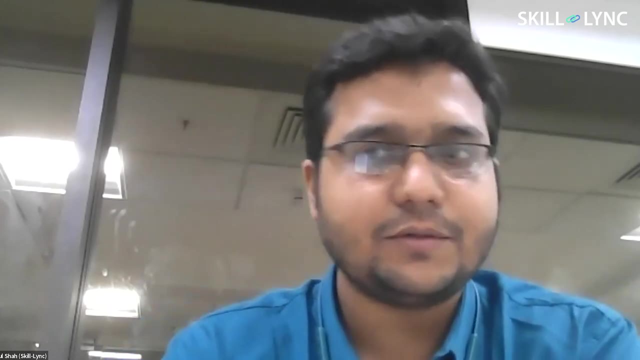 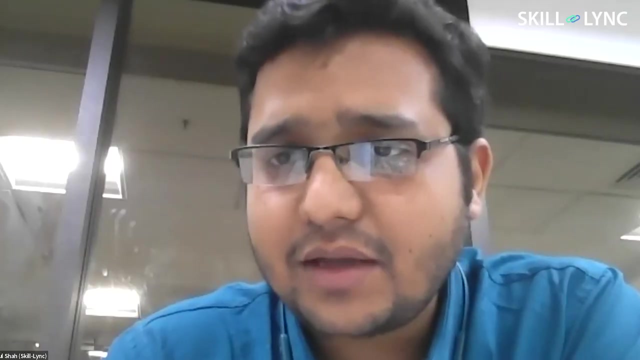 uh, you know, make my career, or how to get a job right in construction management, or start a career in construction management, you have to learn the program for construction management. so so how about sarah? but i think a lot of people are asking the same question. i think so. 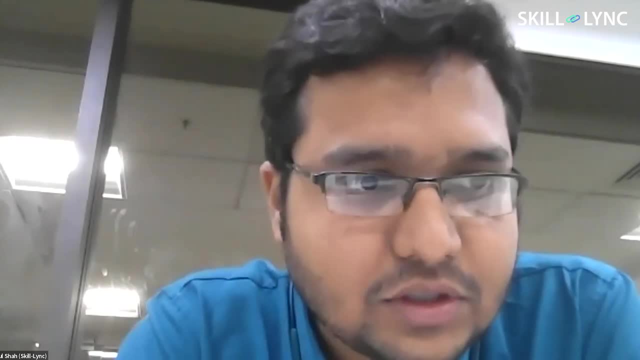 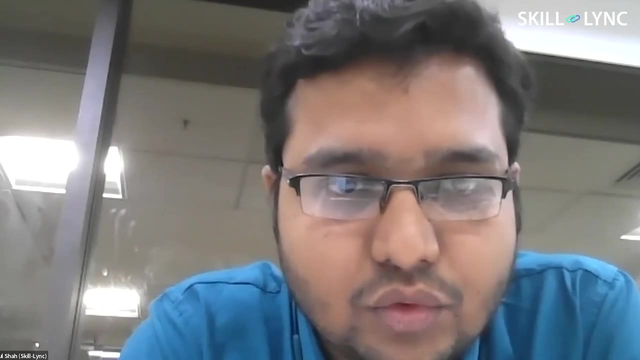 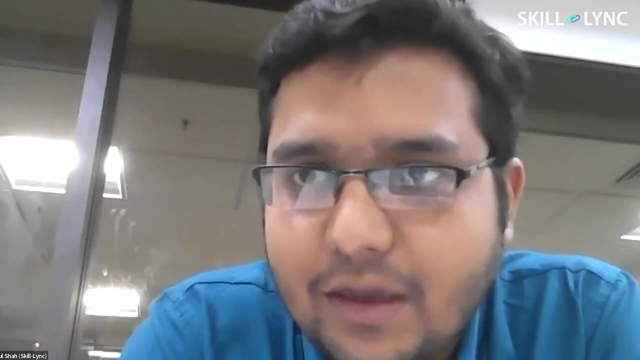 so how about you can basically give a walkthrough about the construction project management program which we are offering? uh, so that people get the clarity about what exactly they are going to learn in terms of tools, projects, etc. and in the meantime, guys, um, those you know who are keep on asking about certificates. so, yes, people will be getting 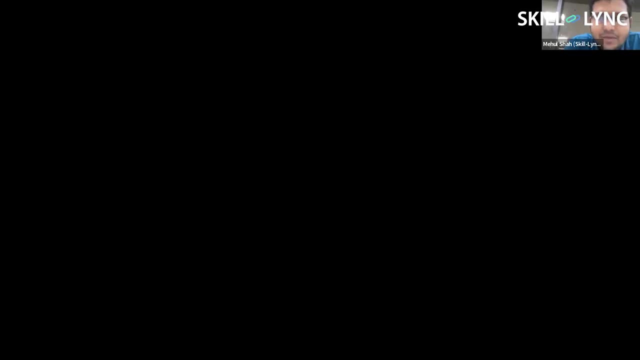 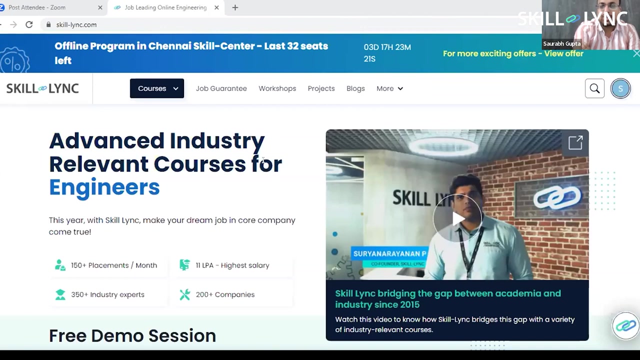 the certificate in two weeks of time through email, but you have to fill up the feedback form which we are going to share in another four, five minutes. all right, so, guys, i'll not be taking much time. uh, so, and that was the robustness me, i really used my time for this. skip the course. restart the pieces. 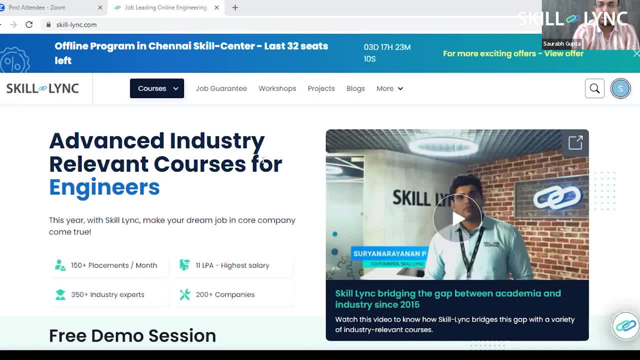 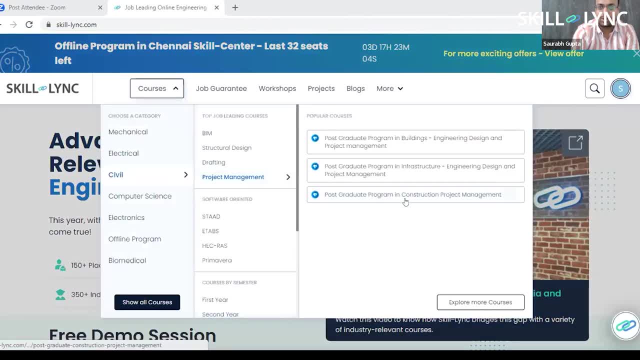 so first, of course, i gave the six modules: uh, very simple and data Heh2 good enough to give the before and after of, let's say, you flirting off like with, you know, with uh having social security and uh experiencing the movement of your whole body, like all the weird things. 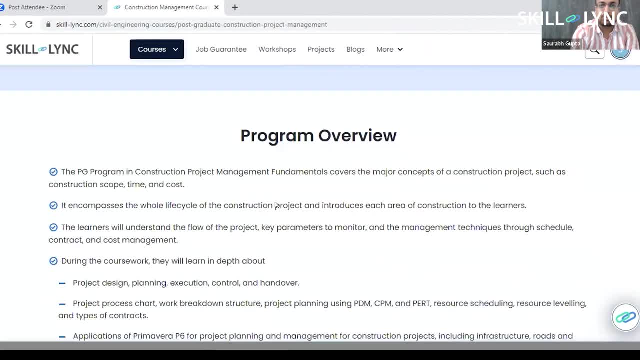 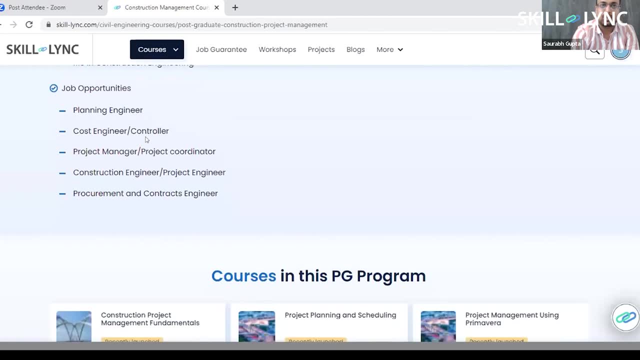 you can say in the course: um and other five things you can actually let me show you sometime about this program. uh, it's very simple, you know. as simple as uh, it's a three- Gimme. these, you know you call this niche, you know, as subgroups, so under them you can use a users for if you. 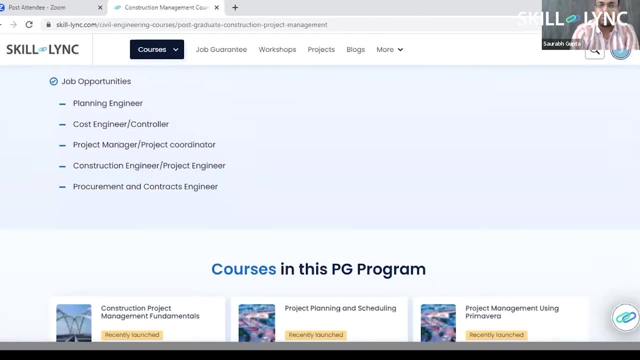 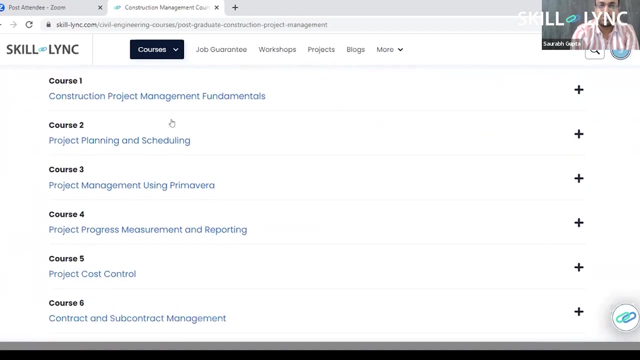 want to access these ange, indefinite- or even the vendors for early design services, depending on your cost: engineer if a experienced person is there, project manager or a project coordinator. get if a fresher is there, or a procurement and contracts engineer. so this program consists of basically six courses. so first course is related to the construction project management fundamentals. 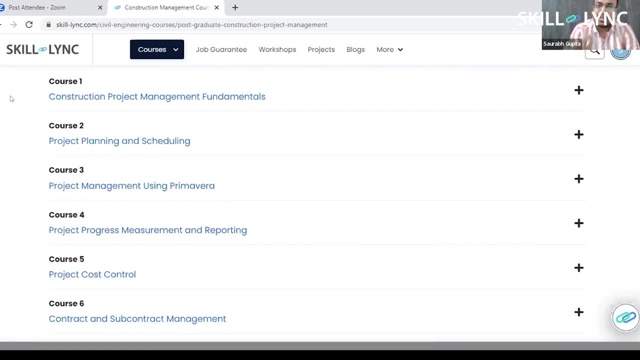 so you will be learning, guys. uh, you know what is the entire project life cycle starting, which which we discussed initially like starting from the tendering for each thing. then second course is related to the project planning and scheduling. here you will be learning how to plan a project. 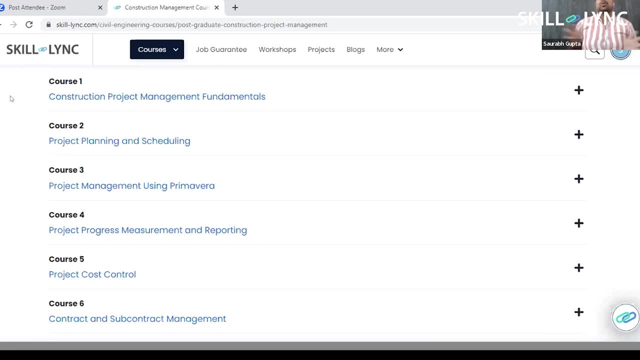 how to- uh, you know, make up your mind how we will be doing the planning and scheduling. third thing: the same we have to learn with the help of primavera. so you will be doing entire things on the primavera software. so this is the latest software, which, which i believe that everybody 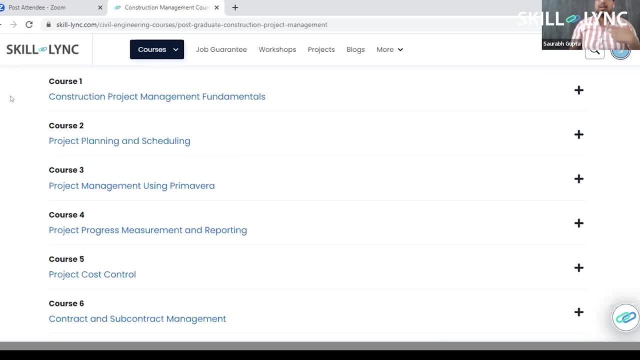 should learn. fourth thing is the progress management, measurement and reporting. so here a lot of techniques are available, like earned value management, a bar chart, techniques s curves and you know you have to do a lot of reporting, you have to do a lot of communication, you have to write a lot of uh correspondences. 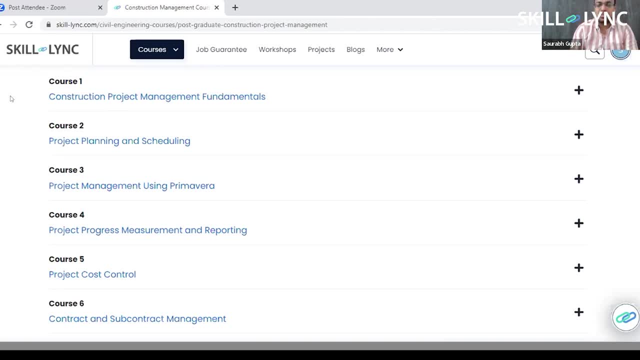 and later that you will be learning in this course for then. fifth course is related to the project cost control. so you know you have to develop a budget. um, one beautiful thing is that construction projects are a lot of. you know they are either in hundred crores minimum or in thousand. 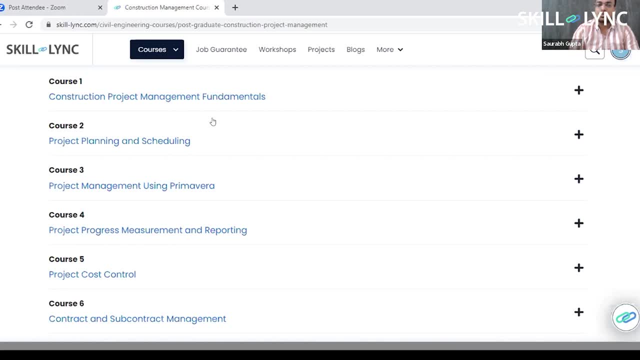 crores. so then you have to make the estimate of those projects it may be of. you know how to make the direct cost, indirect cost, how to make the financial statements. everything is done by the civil engineers. so you don't think that this civil engineer is just going to the site and he's just 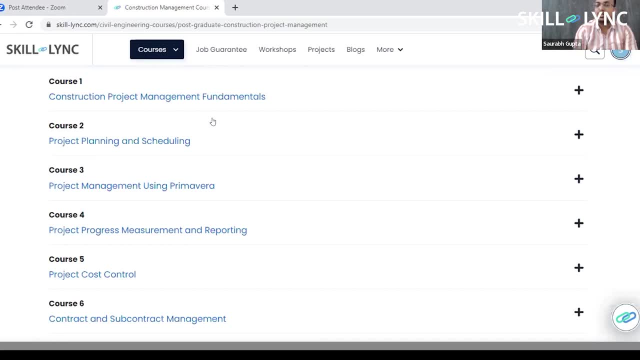 watching how the construction is going on. no, everything is done by the civil engineer only. so now in contract and subcontract management, how to read the contract, how to read the general conditions, special conditions? what is the international type of contract that is free contract now, big companies like lnt or tata or shop or j. they don't do everything by their own. 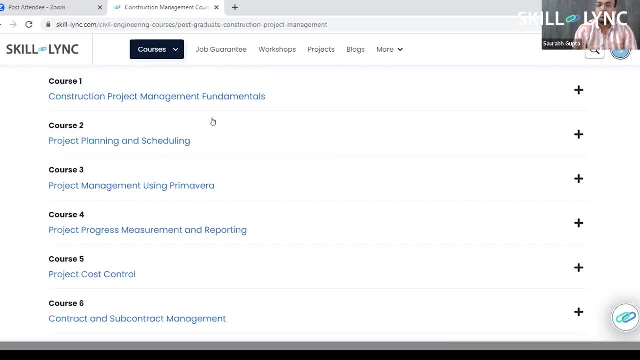 they will be deploying so many subcontractors, petty contractors- if they have to buy the material- cement, steel or anything- they will be buying it from the outside companies because they are the oem companies. so how they will be giving the contract to these small companies then there. 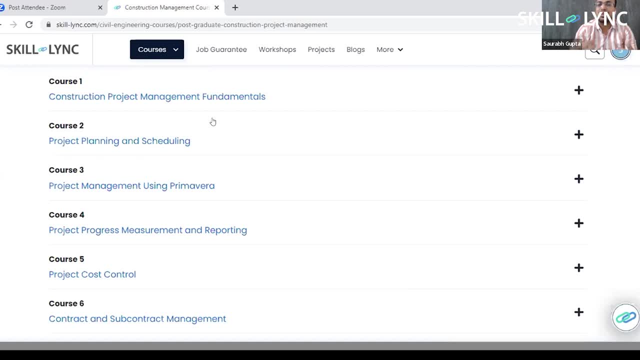 will be disputes, so how those disputes will be handled. it's not like that any lawyer will be coming. so under under this, you know a lot of uh friends who are girls of mine. they are working in contract and subcontract management. so all these are the job roles, uh, which anybody has to learn. 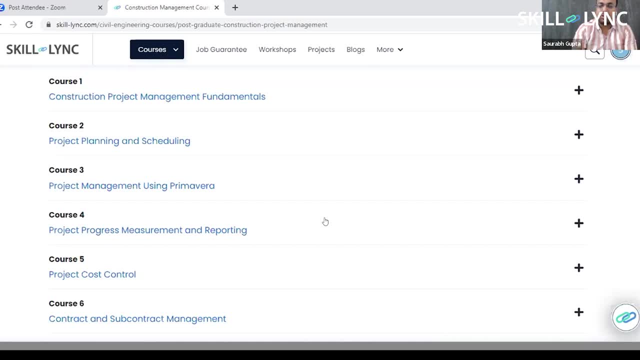 in their career. if you are a fresher, you have to learn. if you are in student, you have to learn. if you are working from last 10, 15, 20 and number of years and you do not know construction project management, you cannot become a project manager, that's for sure. you cannot become a regional head. 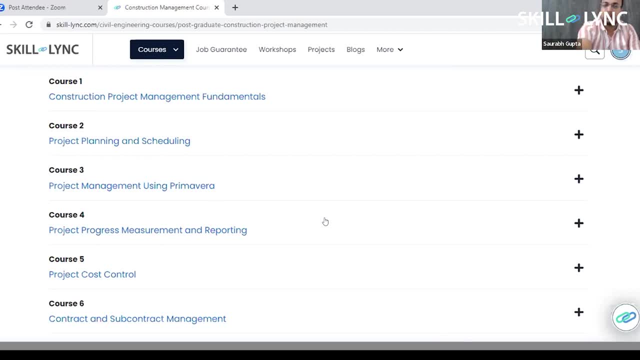 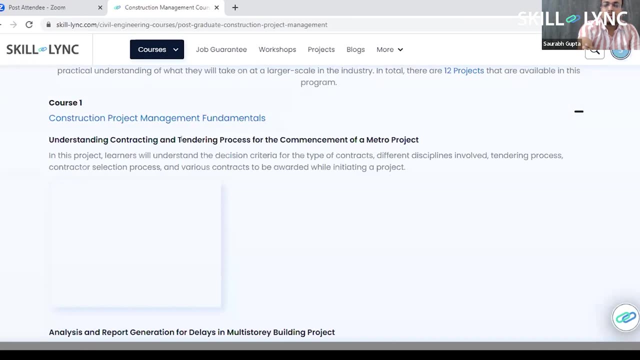 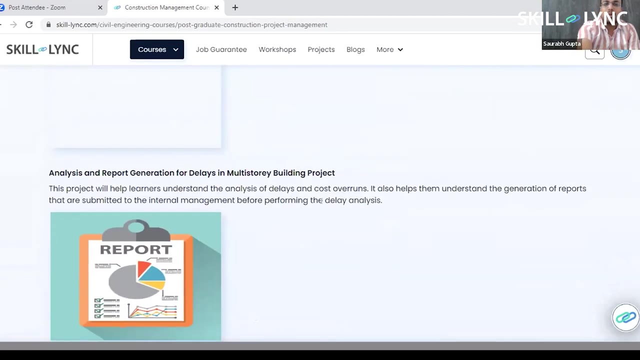 you cannot become a business head, you cannot become a cx of that company and similarly, you will be having you know uh projects. so, like one that uh, you will be working on these projects. that you know how to do the tendering process for a metro project, how to prepare the reports. 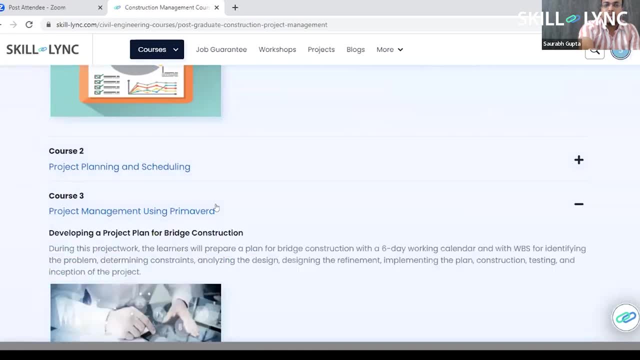 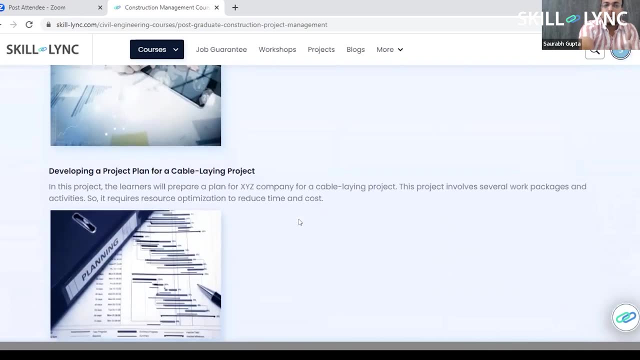 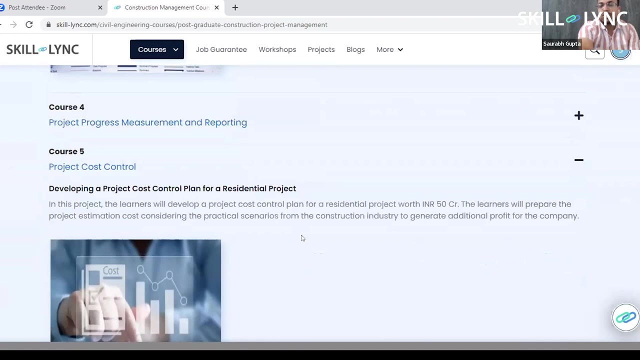 and delay for a multi-st, multi-story building, then how to prepare a project plan for a bridge construction in Pramaveda, how to do the make a plan for cable laying project, how to make a uh project budget for a residential project. so these kind of extensive projects will be there on which you will be, you know, demonstrating and 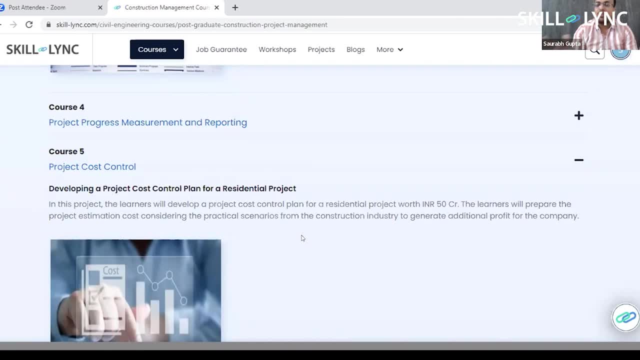 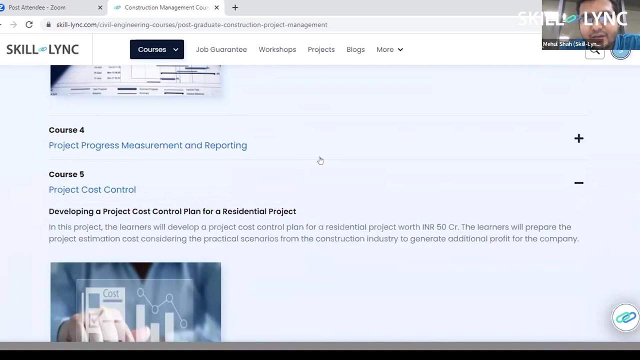 practicing, so then you can demonstrate it to anyone. yeah, I have done these kind of projects and I have gained the knowledge, so likewise you will be learning all these aspects. great. I think that helped you know a lot of uh folks in getting the clarity like what exactly needs to be learned. yeah, thank you so much for having me. thank you so much for having me. thank you so much for having me.